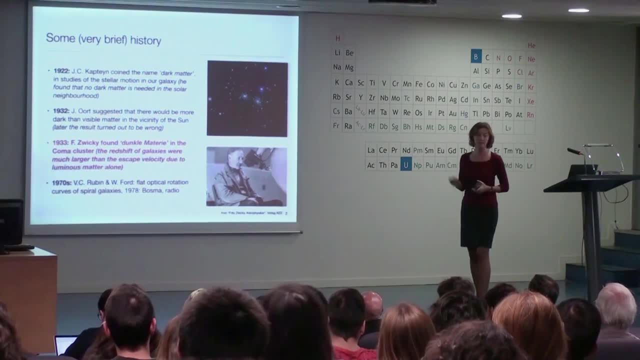 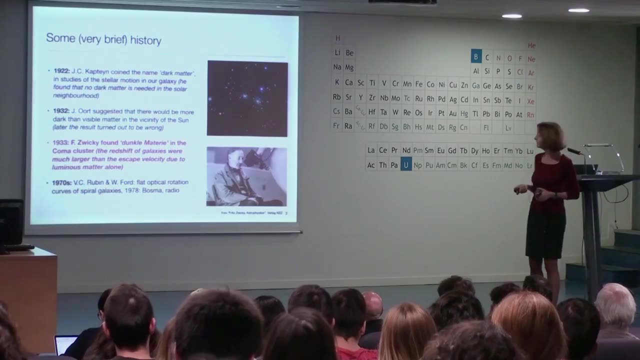 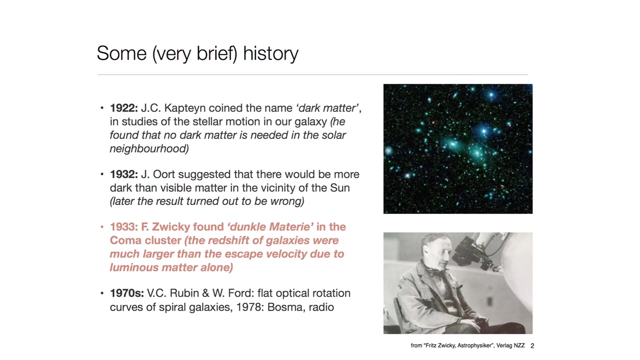 And finally, you know, fast forward 33,. Fritz Zwicky found this dark matter, dunkle materie. He was a Swiss astronomer, working, however, at Caltech in the Coma Cluster, where he studied the redshift of galaxies, And those were much larger than the escape velocities that would. 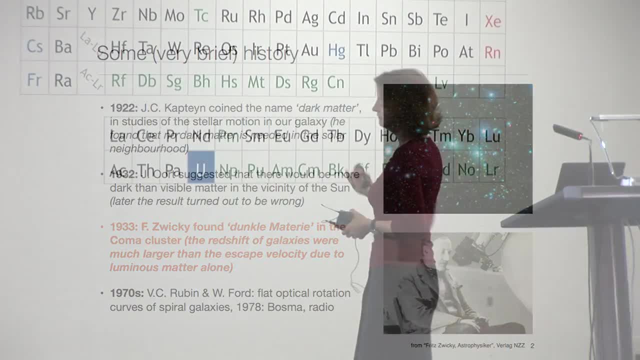 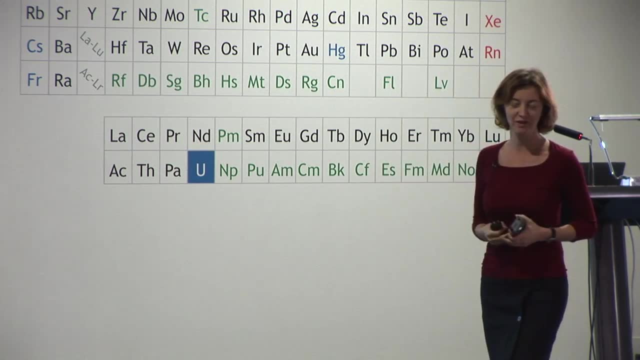 be due to the luminous matter alone. And well, this was a very, you know, very, very interesting study. He was in many ways ahead of his time. You know, he was quite famous. He's quite famous now And it seems also he had a difficult character, But in 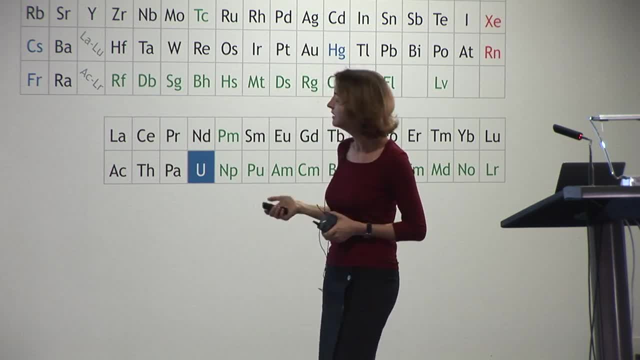 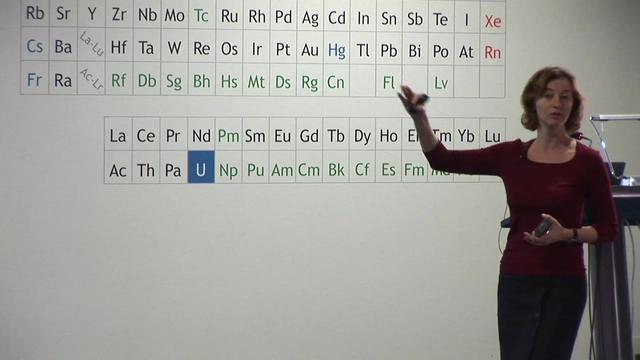 any case, this result went quite unnoticed for a long time, maybe until the 70s, when Rubin Ford and others studied, in fact, the rotation curves of galaxies. They saw this well flat optical rotation curves. Later on these were studied also in the radio. 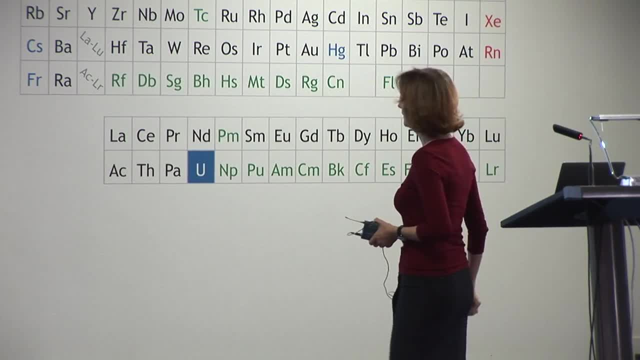 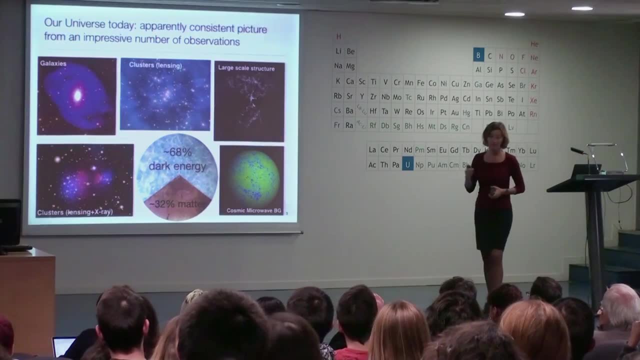 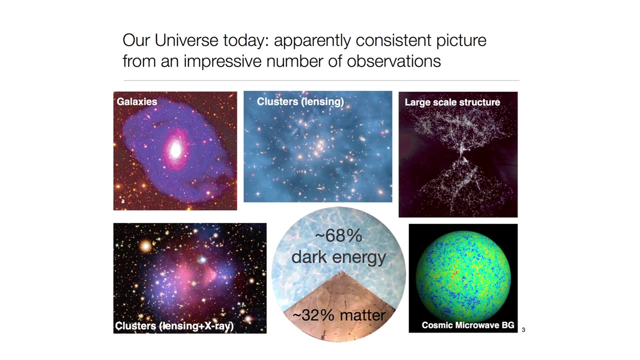 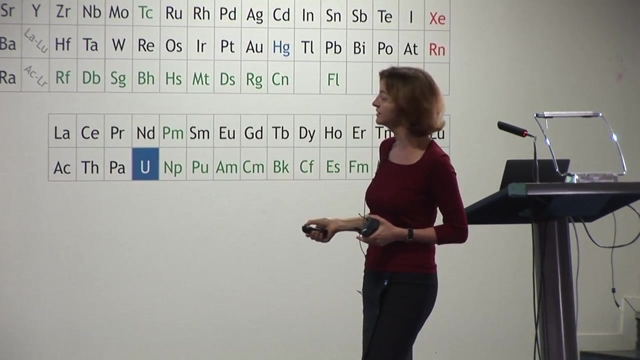 that allows you to go to much higher radii. So this issue then got renewed attention. let's see until now, really fast forward to today, when we have many, many observations, astrophysical observations, cosmological observations on an impressive range of scales, you know, from galaxies to clusters of galaxies, to large-scale. 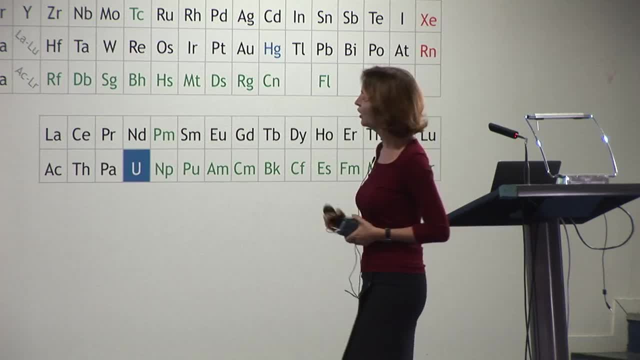 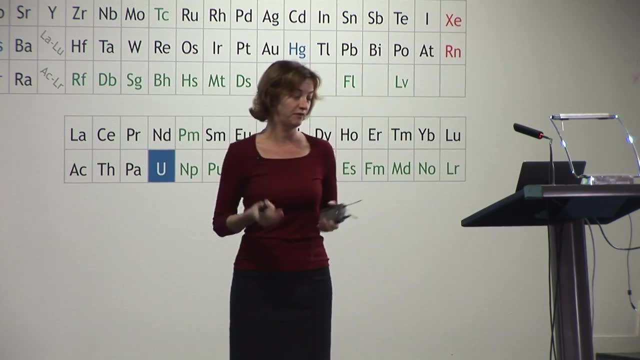 structures and finally also to the very early times in our universe, And you know this very well here. So this is a very interesting study. the cosmic microwave background And all of this seems to give well a so-called consistent picture of our universe, where about 68 percent 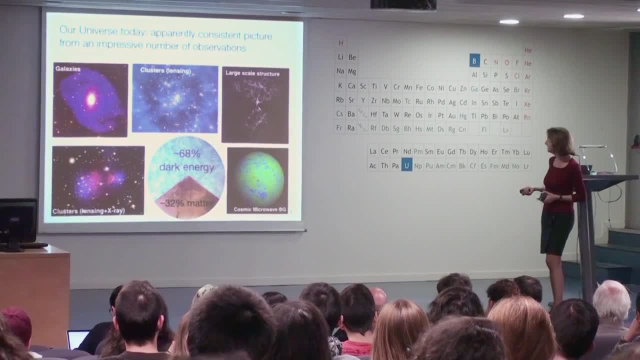 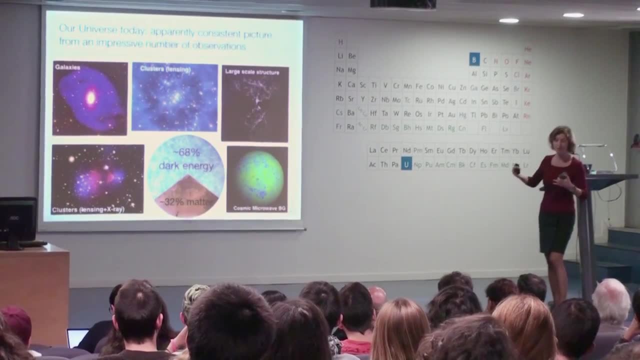 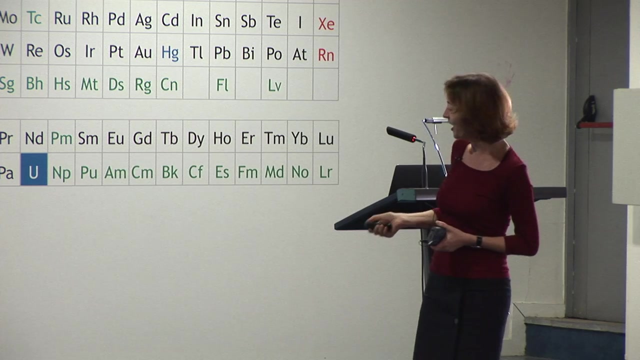 of the matter and energy content is made of dark energy and about 32 percent of matter- Coincidentally, this happens to be. this is the ratio of water and, you know, soil on Earth. There's, of course, nothing to do with this. I just found this picture, But obviously 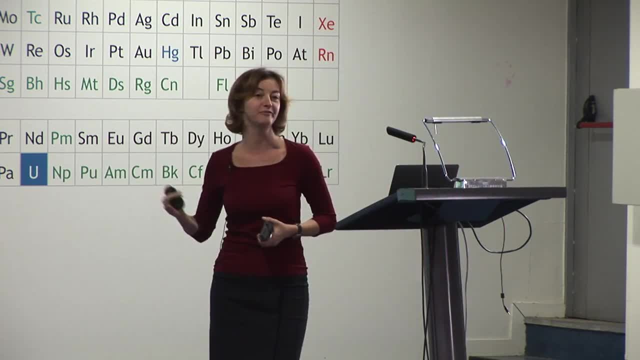 and out of matter. out of matter, you know you can't see it. You can't see it. You can't see the particles, You can't see the constituents of matter. Out of the matter, about 85 percent is dark matter, while the rest is luminous matter and even a fewer percent is stars. 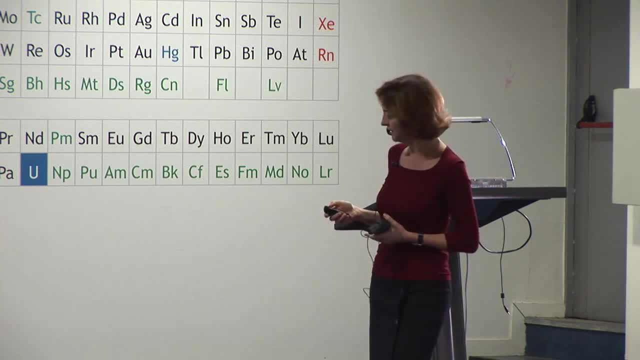 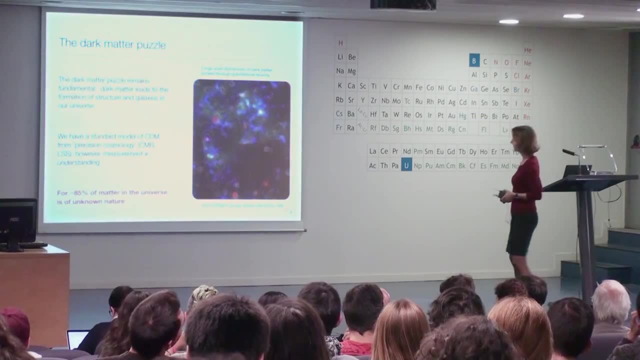 So, even though we do have this nice picture of the universe, the question is: what is what is? well, dark energy and dark matter. But today I will deal with a dark matter puzzle And in my view it is fundamental because we know that this dark matter leads. 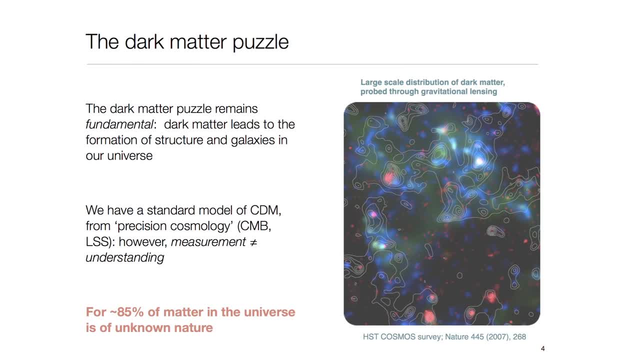 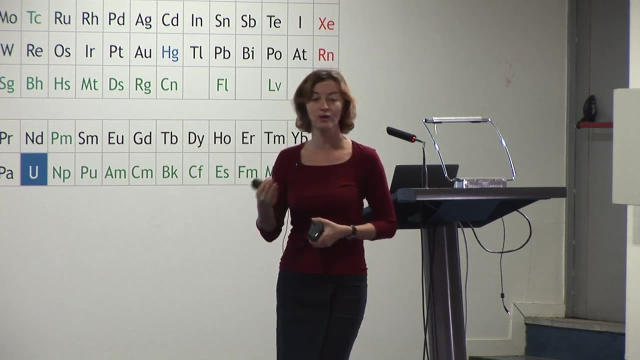 to the formation of structures in our universe And we can study these structures on the larger scales, scales, you know, through the influence of this dark matter. so the gravitational influence of the dark matter on the luminous matter. okay, And even though we have now what we call a standard model of cosmology of cold dark matter, 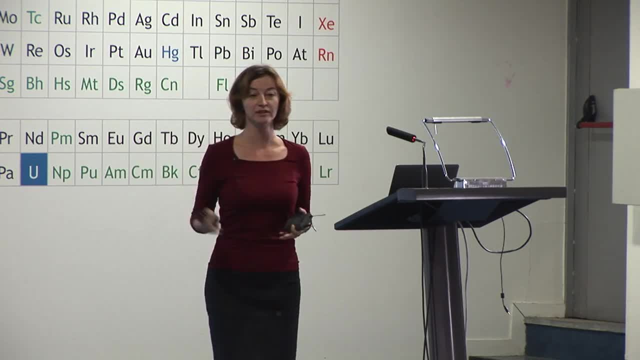 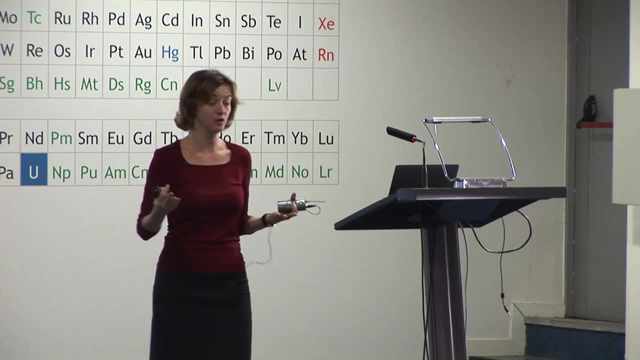 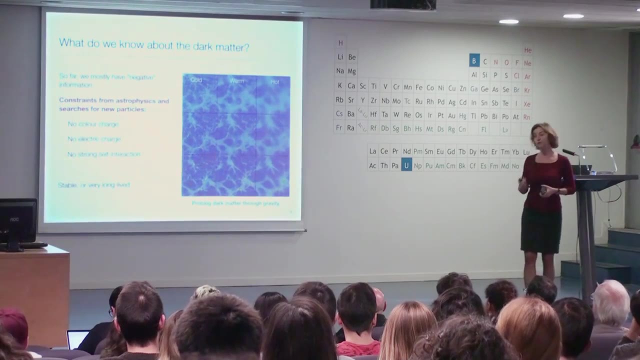 the lambda CDM model. you know, precision doesn't mean also understanding because, as I mentioned, you know, 85% of the matter in the universe is unknown. we have no clue what this dark matter is made of. So let's see first what do we actually know about it? 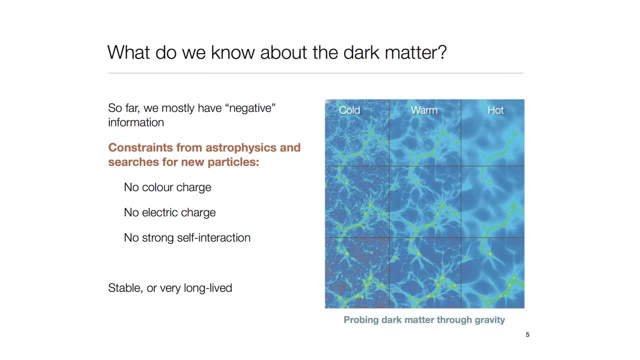 And I mentioned already, we can study, we can prove it through gravity, but what else? So we have a lot of constraints from astrophysics on the one hand and, on the other hand, from searches, from various searches that I will mention. 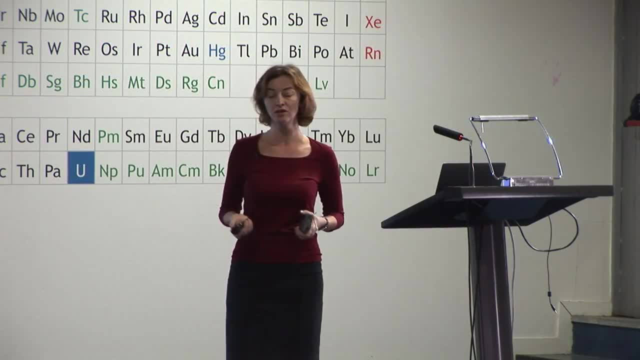 So it does not have any color charge, it doesn't have any electric charge and it might have some self-interaction. Okay, So it might have some self-interaction that we don't really know, but it doesn't seem to be very strong and those constraints are actually also coming from astrophysics, from. 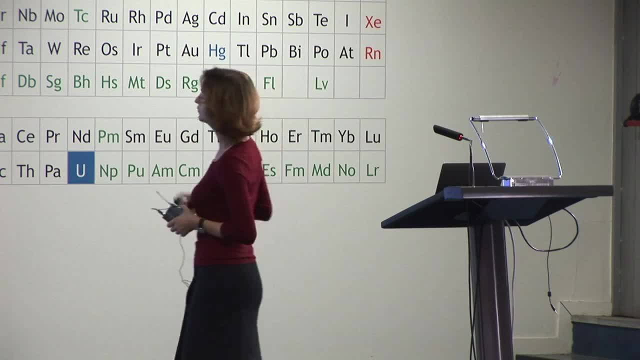 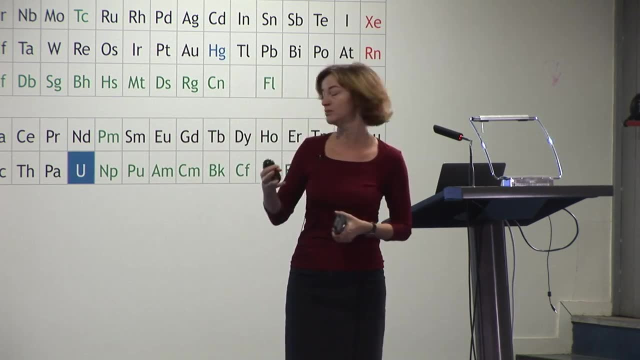 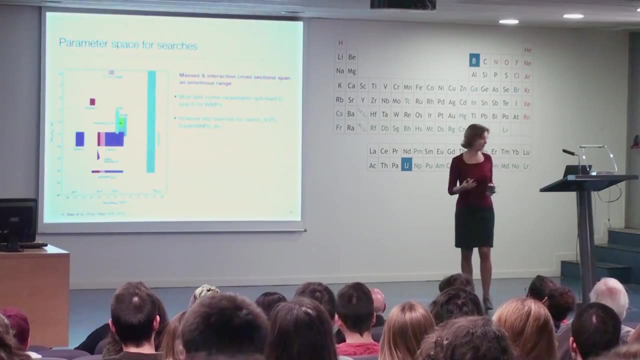 something like the bullet clusters, for instance, And in order to be the dark matter in our universe, it has to be either stable or, if it decays, then it has to be very long-lived, obviously, Now. so I said we don't know what the dark matter is made of, but we do have a lot of 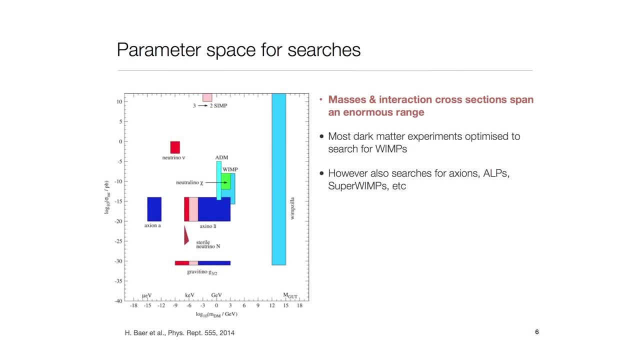 ideas, or should I say the theorists have a lot of ideas. This parameter space here that is just a cross-section of the dark matter particle. we are assuming now that it's made out of a new particle with normal matter, normalized here to low-energy. 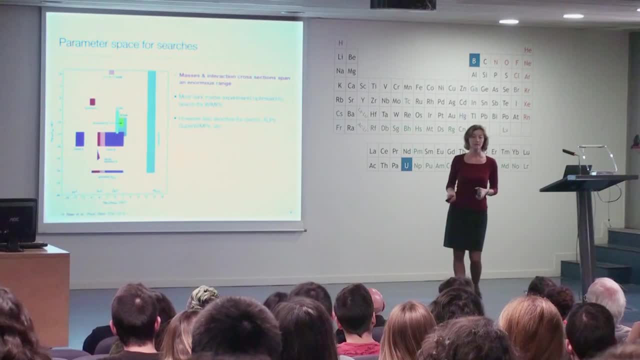 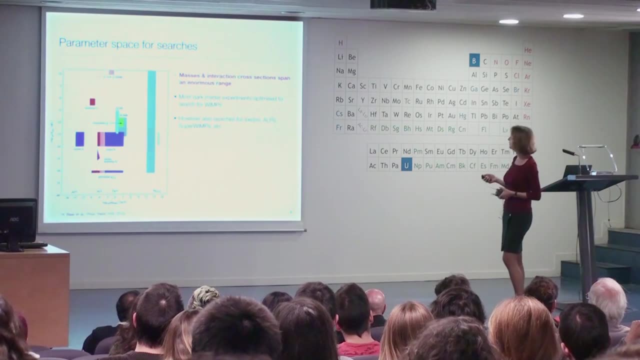 neutrino cross-sections as a function of the mass. okay, this spans about 80 orders or so in magnitude and most searches actually are optimized, as I will show you, to search here: for this region, for WIMPs, for weakly interactive massive particle. looks like a. 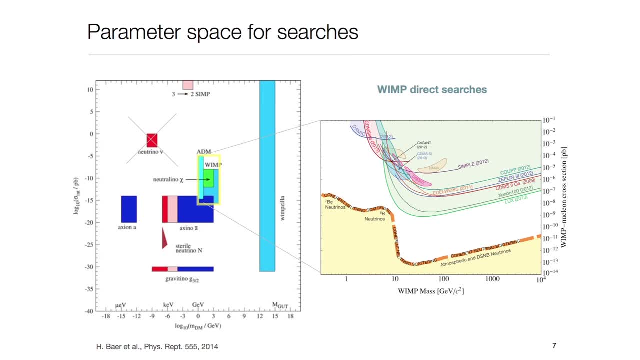 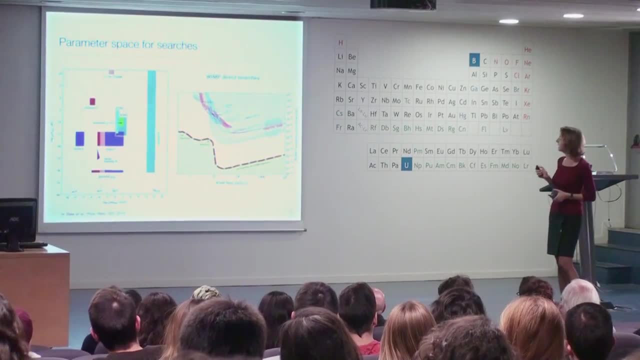 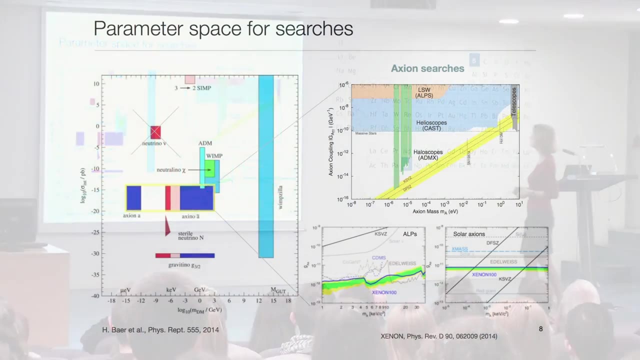 small region In this immense parameter space, but actually it is not so small, as I will show you in more detail later on, And even though I will not really talk about this today, I also would like to mention that this parameter space here is also being searched for with the so-called axion searches. okay, 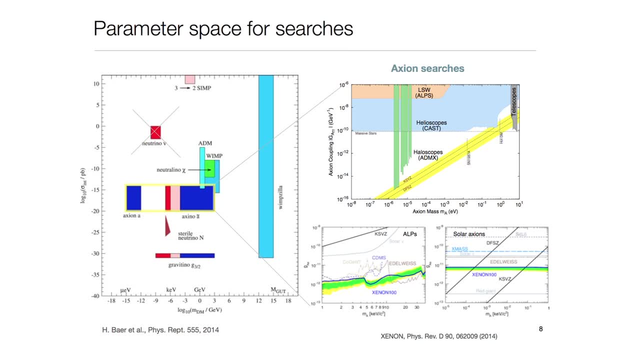 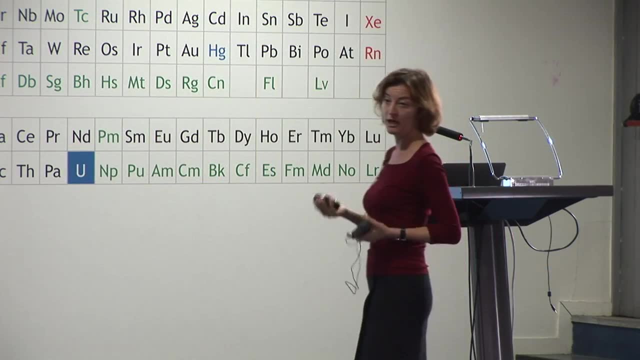 So we have the axion dark matter experiment that is looking and will actually cover here a relevant part of the parameter space for the standard QCD axion. And then we have other type of searches that look for so-called axion-like particles, such 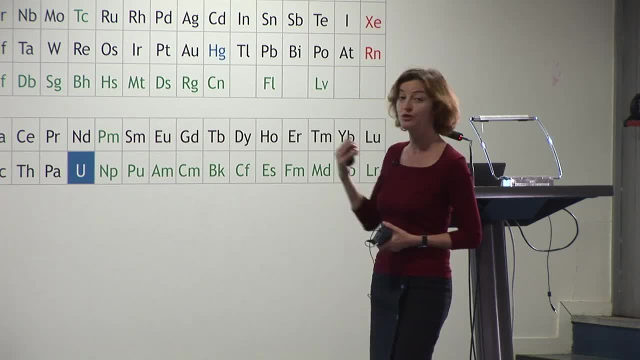 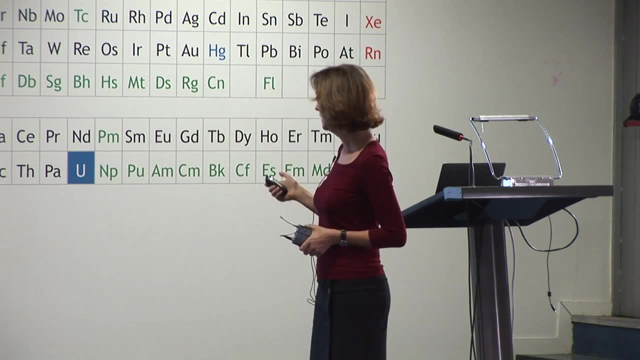 as these light shining through wall experiments, or so-called helioscopes, so like the CAST helioscope at CERN, looking for axions coming from the sun. And another remark: the experiments that I will talk about here today are, in fact also. 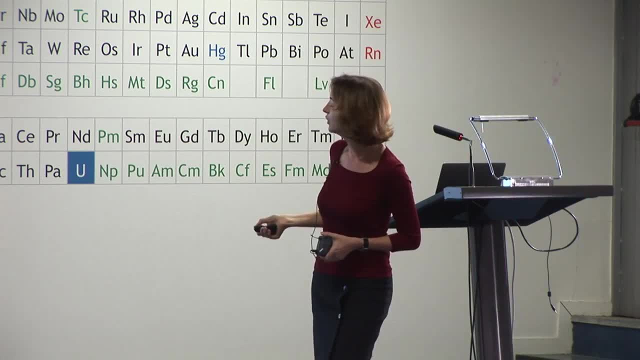 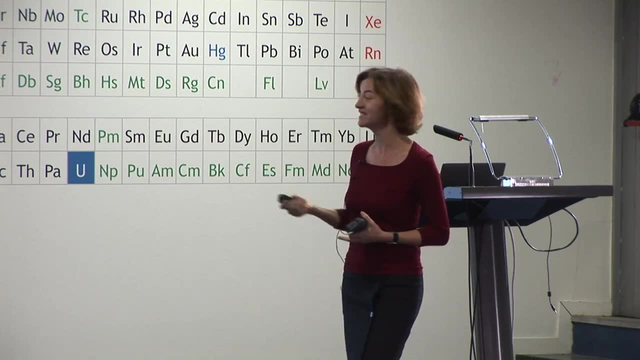 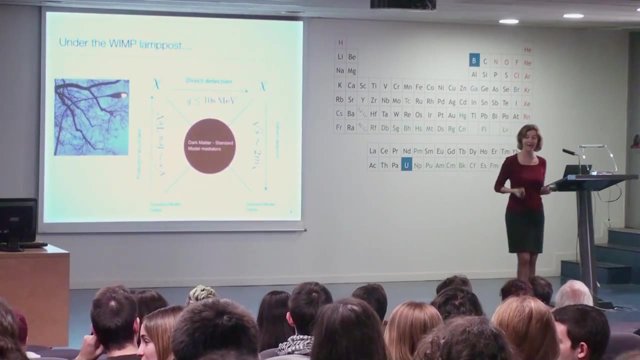 starting to set at least constraints on axion-like particles, but also on solar axions. However, maybe you can ask me later- you know, at 3.30, because I won't have time to really go into this here. So now, let us assume that we are under the so-called WIMP lamppost and we are assuming. 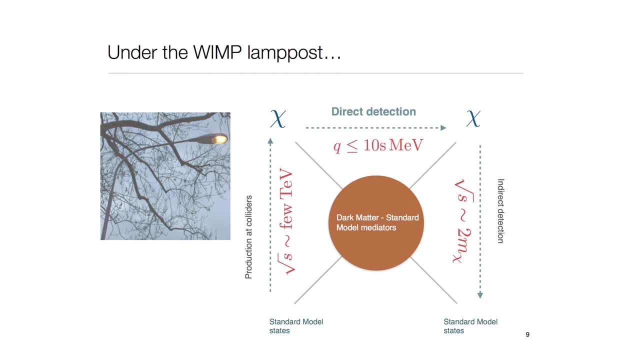 that our dark matter candidate is a so-called weakly-interacting massive particle. that is just a very generic name, for you know, for classes of dark matter candidates from theories that go beyond the standard model of particle physics, such as supersymmetry or universalism. 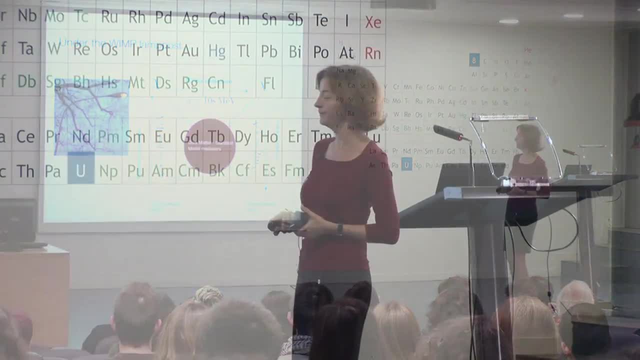 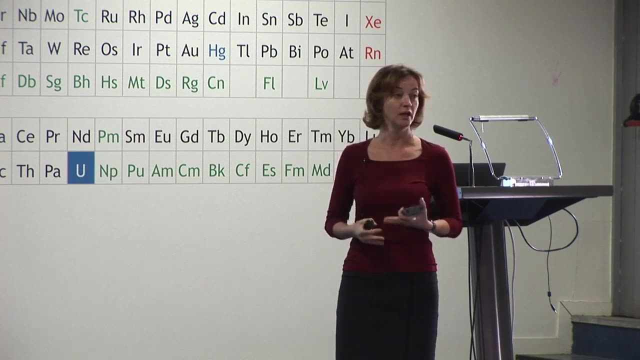 Okay, Universal extra dimensions and so on. So we assume that because this particle annihilated in the early universe, it has some kind of interaction, apart from gravitational interaction with baryons, with normal matter, so with some sort of mediator. We will come back to this later on. 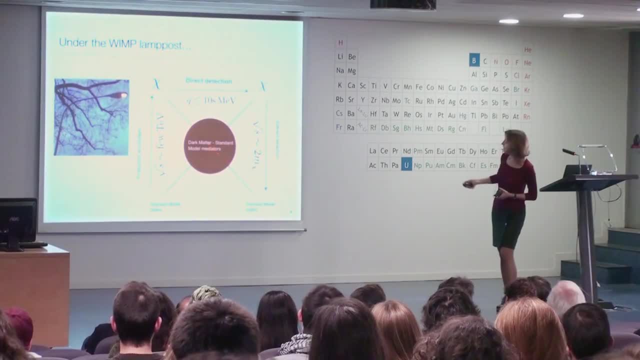 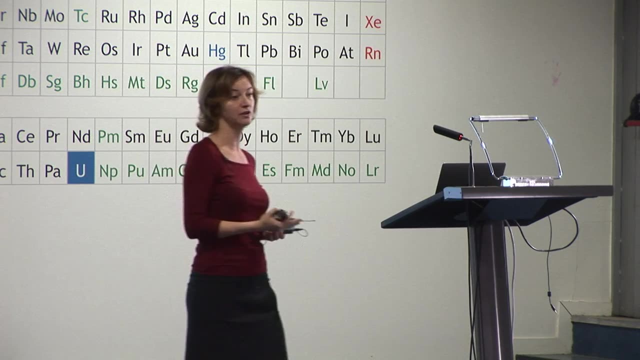 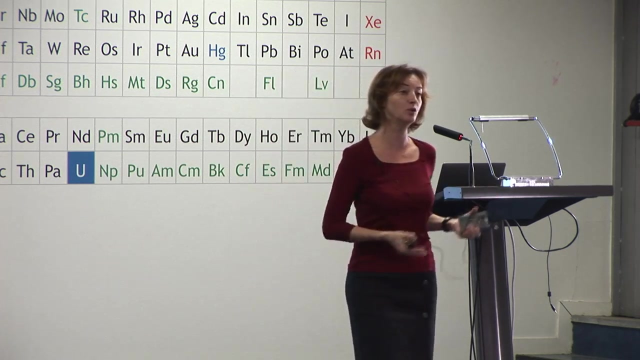 And then you can try to produce this particle at colliders. so you collide whatever protons with protons and you produce some dark matter states that, of course, will not interact in your detector. So you have to use- you know, you have to use missing energy momentum in order to look. 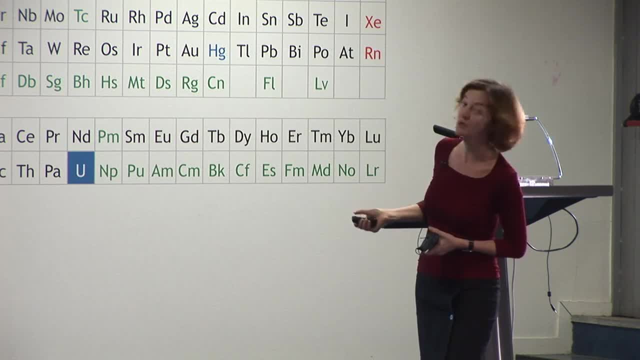 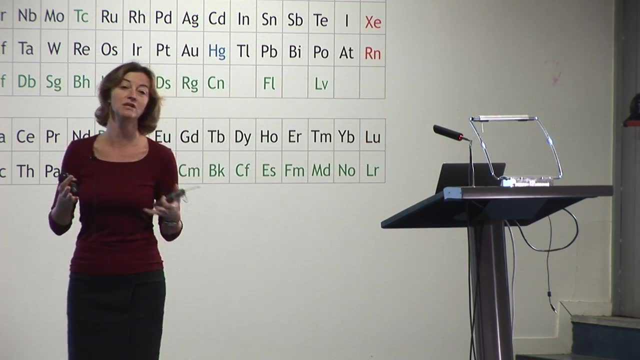 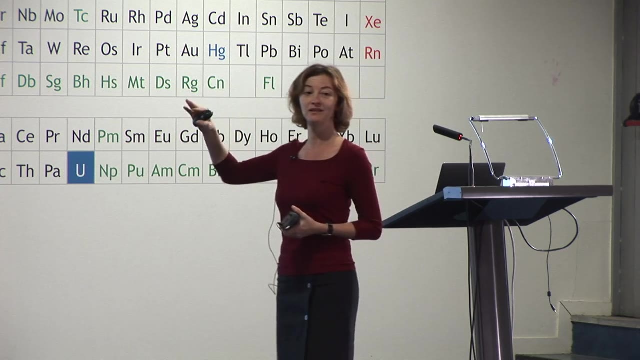 for it. On the other hand, you can still have annihilation of these dark matter particles in regions in our universe, for instance in the galactic centers or around it, or in the sun or wherever, producing all sorts of standard model particles that then decay, producing, for instance, 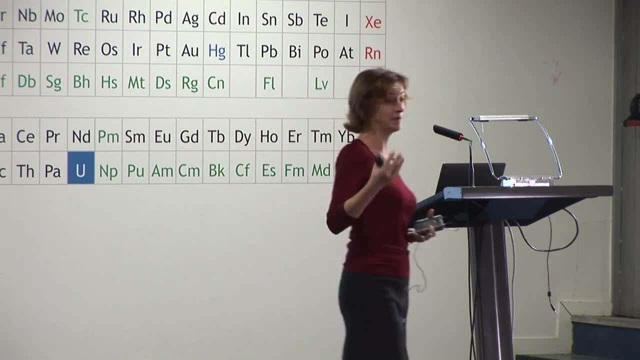 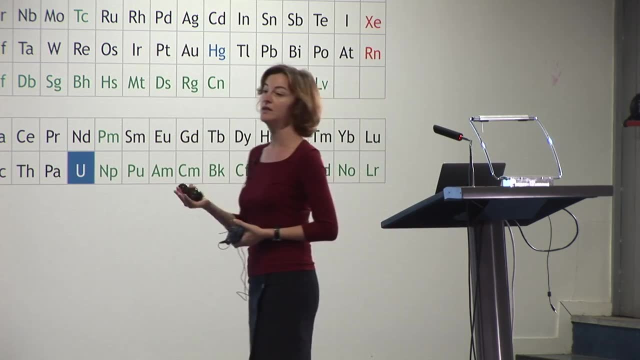 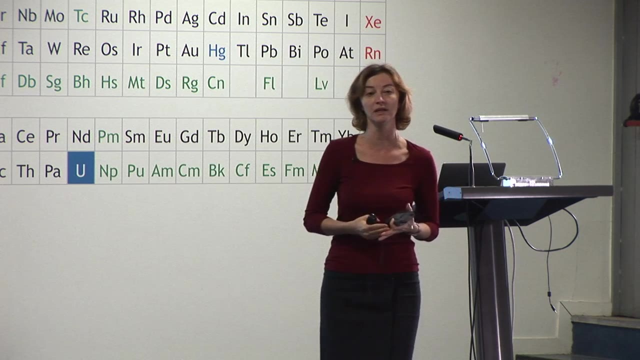 high-energy gammas or neutrinos Or positrons or antiprotons, and this is the signatures that the so-called indirect detection experiments are looking for. basically for this standard model particles above some astrophysical background, And this is quite model independent in some way, because it depends on the annihilation. 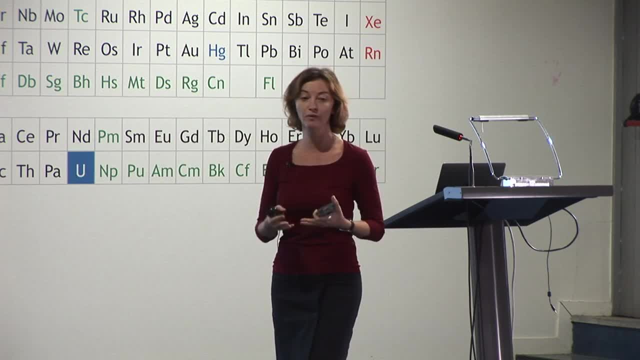 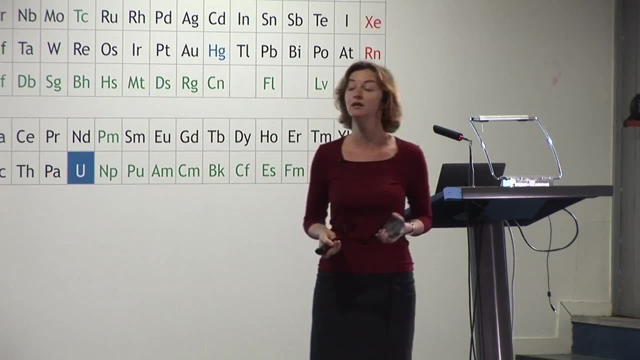 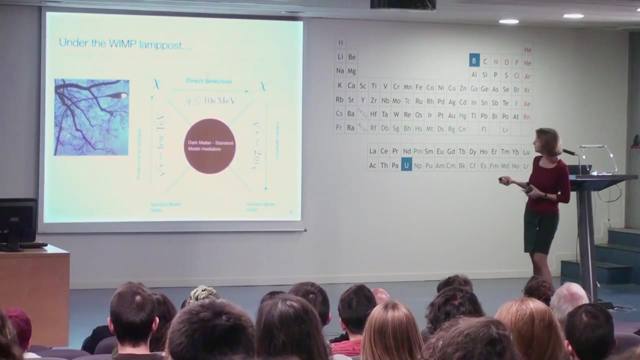 channel, and then it also depends. well then, you have to know very well the astrophysics backgrounds, You have to model the propagation of these particles in the galaxy, and so on, especially for the charged ones. Well, And then, finally, you can have the direct detection, and I will talk more about this. 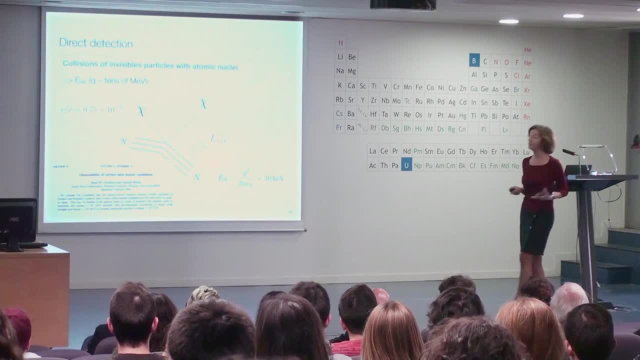 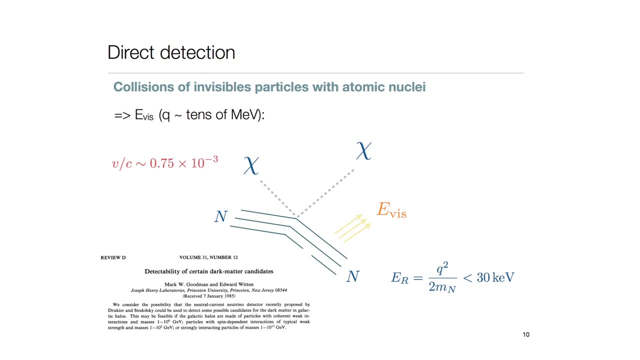 here. This direct detection method actually looks for collision of these invisible particles with atomic nuclei. okay, So the idea is very simple. You have a WIMP and an incoming WIMP that then just scatters in a certain material, mostly elastically of an entire nucleus. 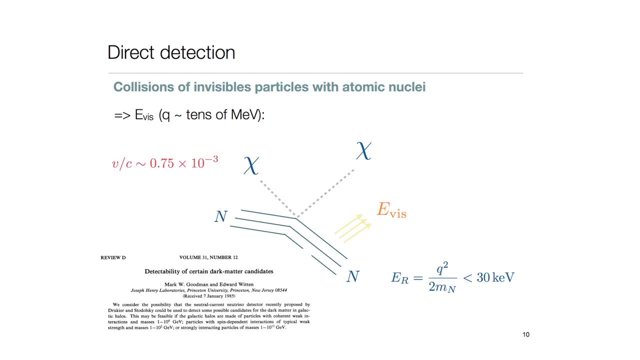 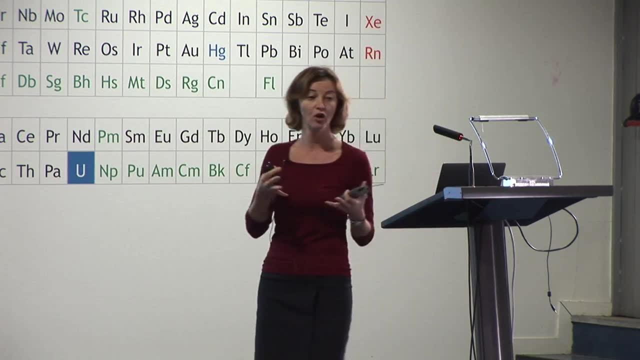 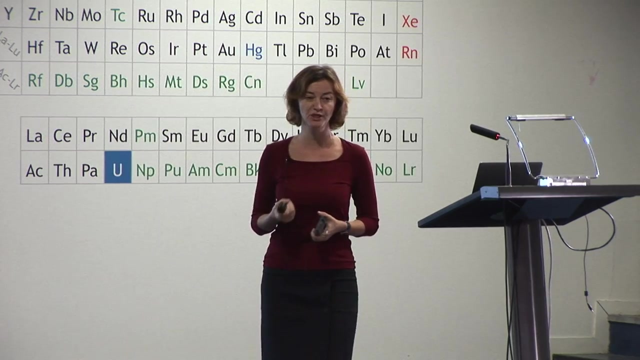 And then leaves again, leaves the detector unobserved. However, what you observe, what you can observe, is a small nuclear recoil, energy that is transferred onto this atomic nucleus. okay, And because, as we shall see, we know from astrophysics this has been actually proposed. 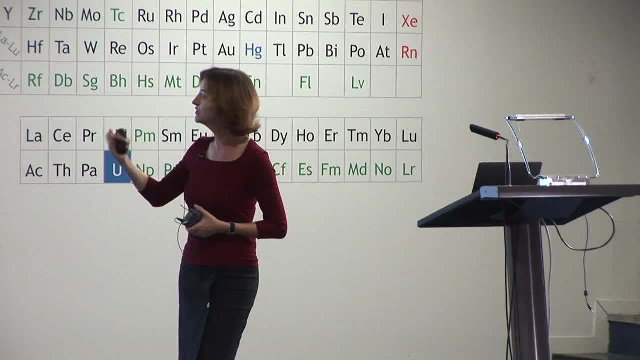 here already in the mid-'80s and obviously I will show you. there's been a lot of progress since then. But because these particles move very slowly in the Milky Way. So you can see that the particles move very slowly in the Milky Way. 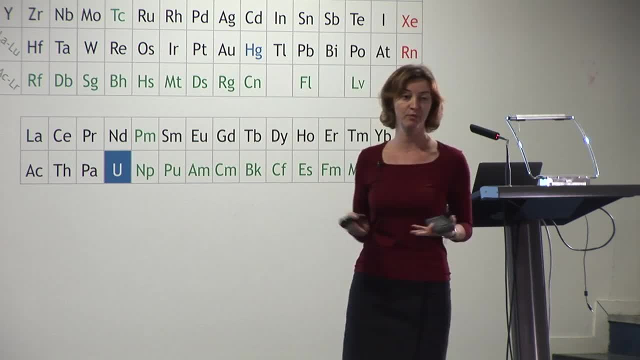 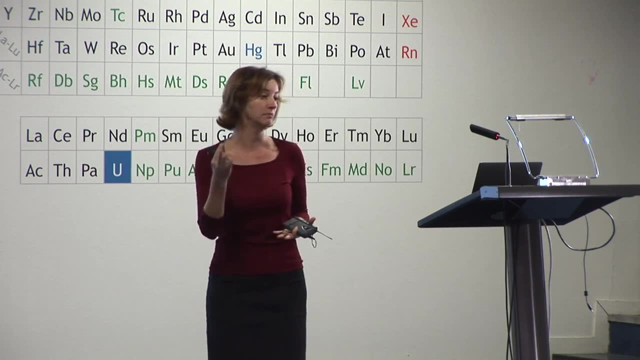 So you can see that the particles move very slowly in the Milky Way. So you can see that the particles move very slowly in the Milky Way, So with about 220 kilometers per second, that's just our velocity around the galactic center. they have low momenta, you know, maybe tens, maybe 100 MeV or so. 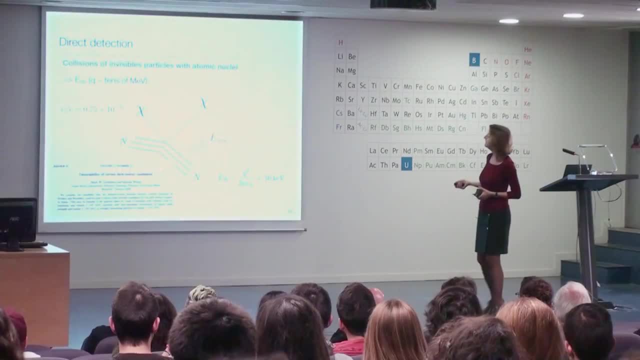 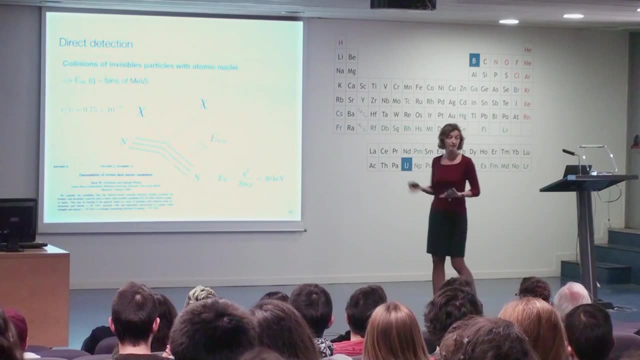 So the scattering will happen in the deep, non-relativistic regime and you will have a nuclear recoil. energy that's from a few kV, as we shall see, depends on the mass of the WIMPs, on where it's in the velocity distribution, to maybe up to 30 or 50 kV or so. 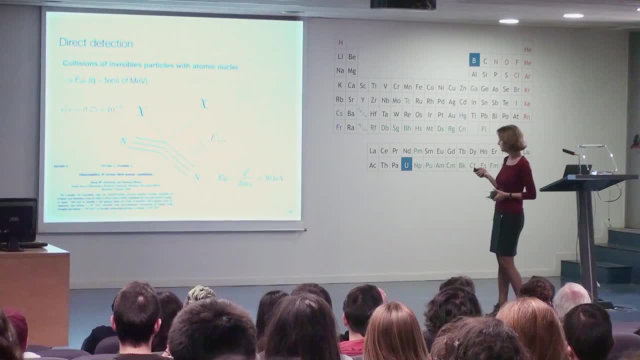 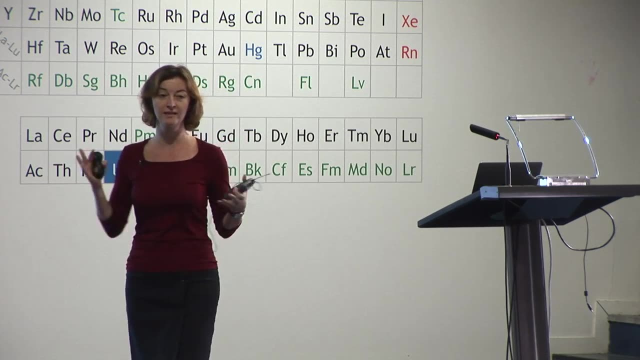 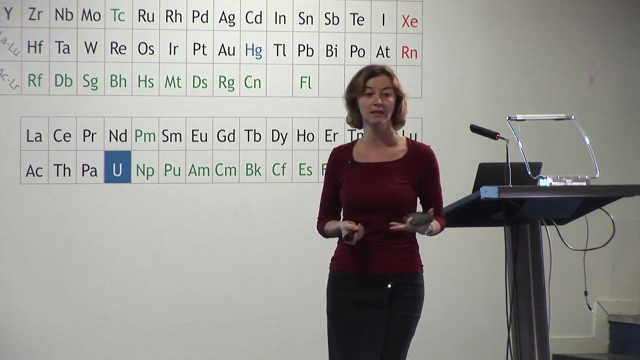 Okay, So very low energy transfer. Now, if you want to build a detector to look for this type of particles that supposedly make up the halo, the dark matter halo of our galaxy, then you need to estimate: what do you expect in such a detector? okay, 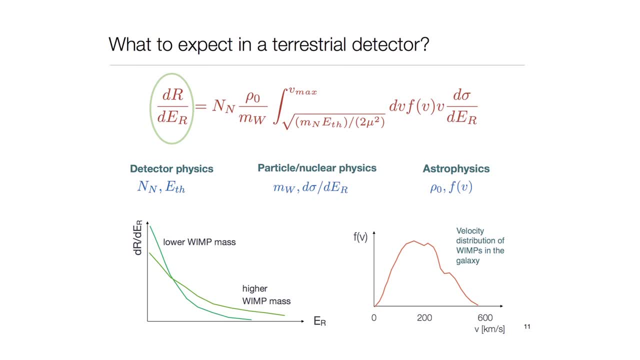 And here on the left side is what we try to measure. It's a differential nuclear recoil rate as a function of this recoil energy And as I will show you it is, it looks pretty boring because it's quite featureless. There's no real peak or something. that is like a you know dark matter. signature. 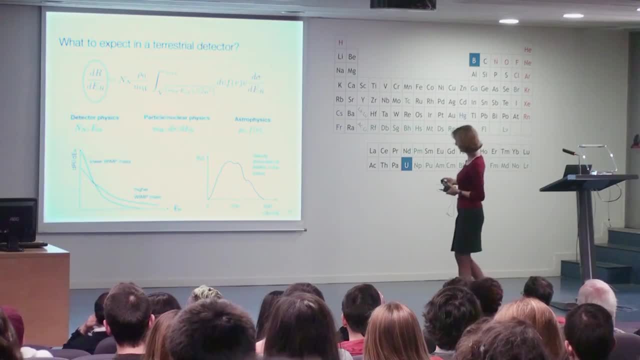 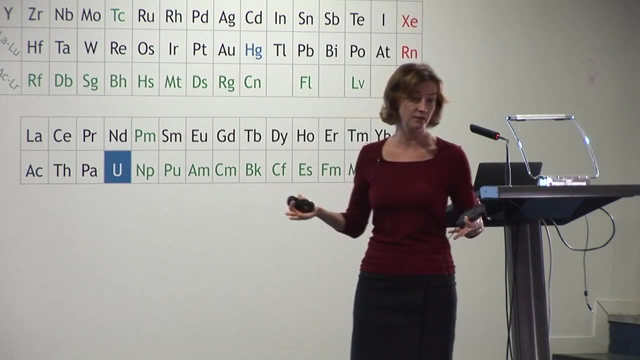 But this then will depend on the number of quantities here from, for instance, from detector physics, obviously on the number of nuclei that you have available for the scattering in your detector. It will depend here on the number density that's given by the local, local dark matter. 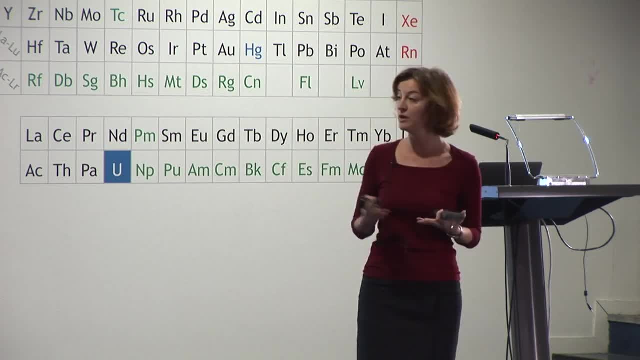 density, So the dark matter density in the vicinity of the, you know, Earth or sun divided by the mass of the WIMP. Then we have here the scattering cross section And here is the integral from some minimum velocity that will depend actually on the. 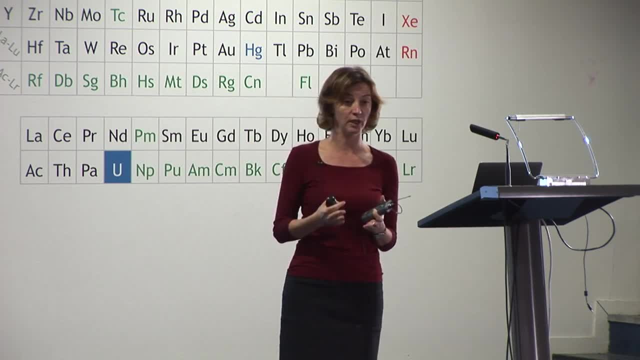 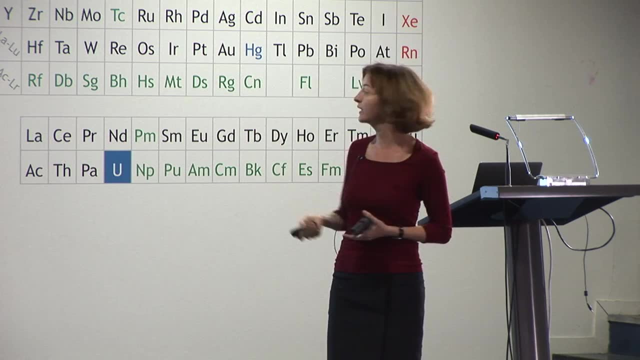 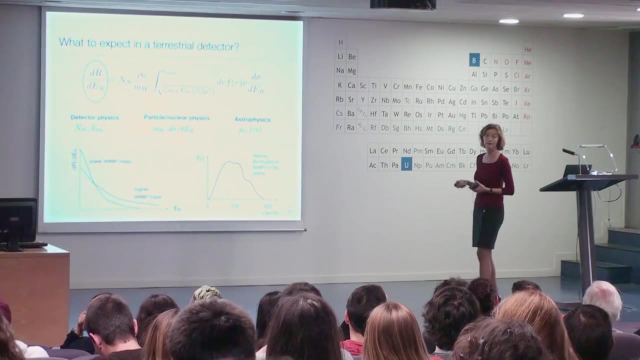 energy threshold of your detector. So the minimum velocity that you can probe of this WIMP up to some maximum velocity that's related to the escape velocity of WIMPs from our galaxy And here the velocity distribution. Okay, So we have from particle physics. ideally we'd like to know the mass of the WIMP and 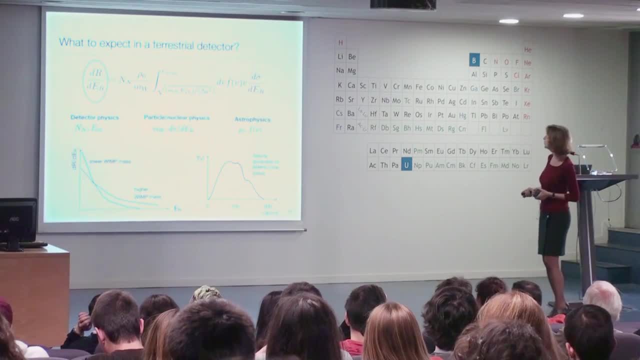 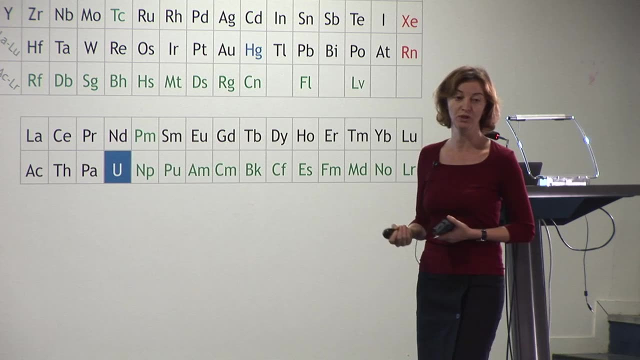 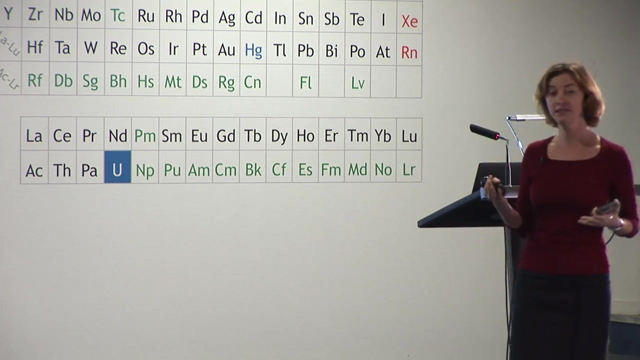 the scattering cross section. So we have only predictions, as I will show you. And then from astrophysics we'd like to know the local density and the velocity distribution. And the velocity distribution, we cannot yet measure it actually directly, But we know it roughly from, and body simulations of galaxy formation. Okay, So it is mostly Maxwellian. However, There seem to be some departures, at least seen in, you know, older simulations: dark matter, only dark matter, only simulations. These days, the simulations have quite evolved and also include baryonic matter. 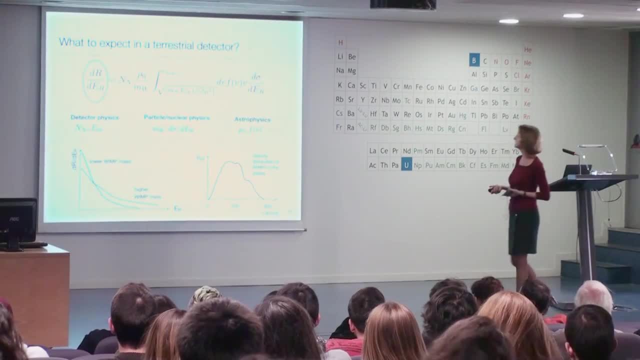 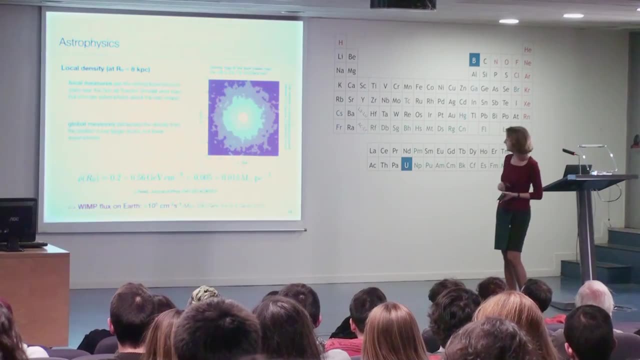 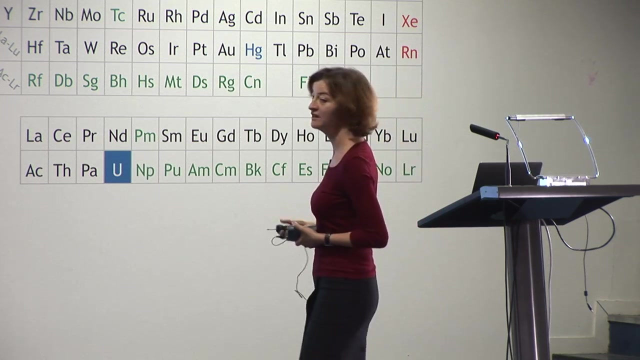 But these deviations are actually quite small and so far are not really significant for direct detection experiments. So we will just briefly now go through this. So from astrophysics there are different ways to measure the local density. Density here at a distance of 8 kiloparsec from the galactic center. 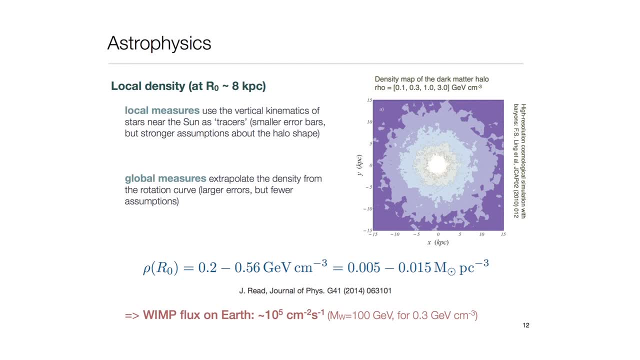 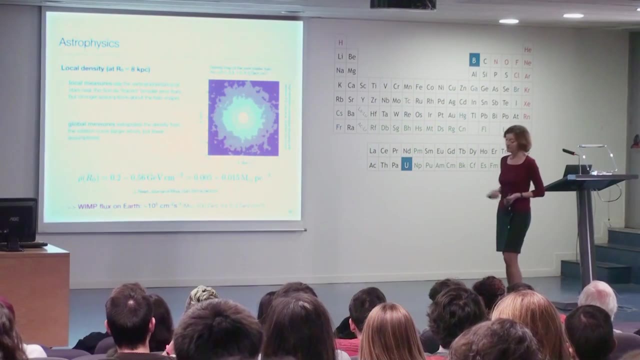 So on the one hand, we have the so-called local measures that use the vertical kinematics of stars near the sun, so groups of stars, as tracers of the overall potential. Well, there are some strong assumptions there about the shape of the halo and so on. 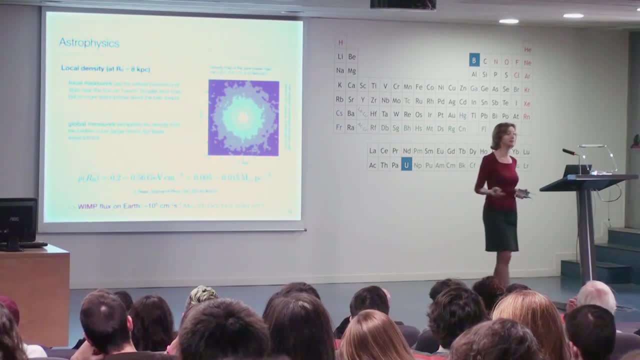 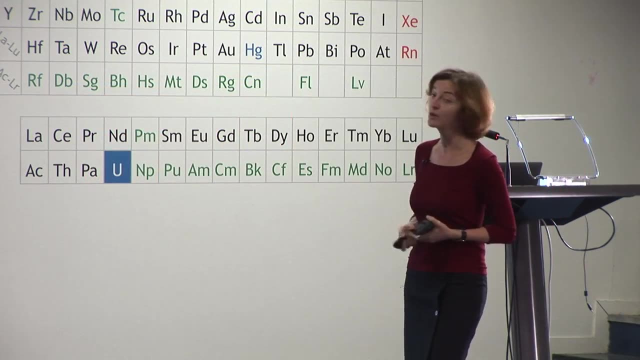 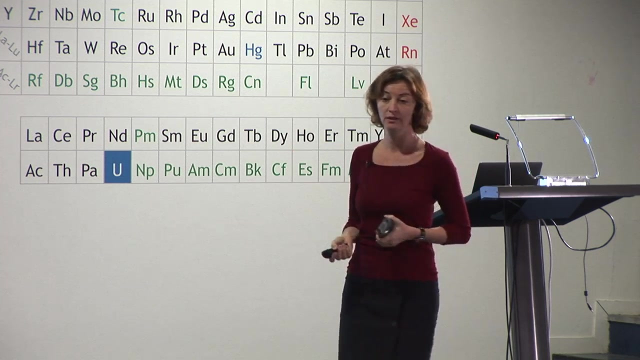 And well, I think now with the first Gaia data, there will be quite some progress in the next few years. Okay, To get a better handle on this, on this local density, from, you know, from the measurement of the position and velocity of millions and millions of stars. 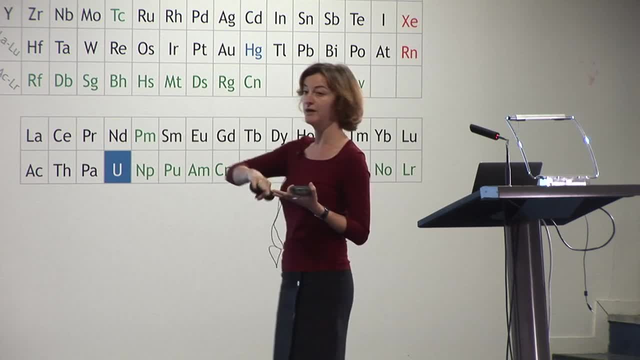 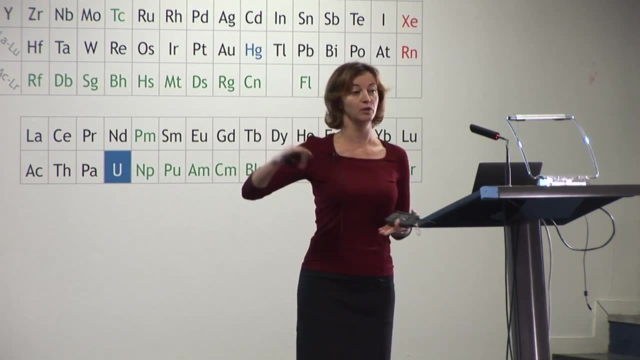 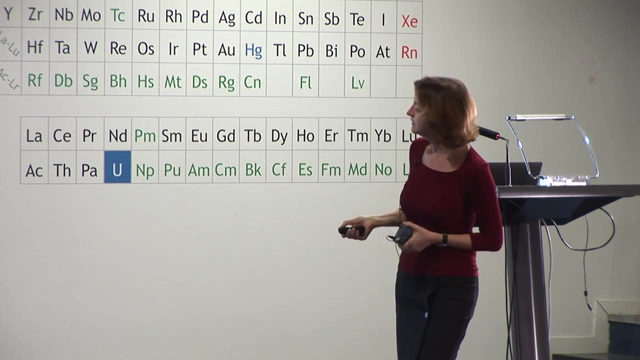 Okay. Then we have also global measures where what is measured is the rotation curve of the Milky Way, And of course we have to model. you have to model everything, the dark component, but especially the baryonic component, And that is not trivial. 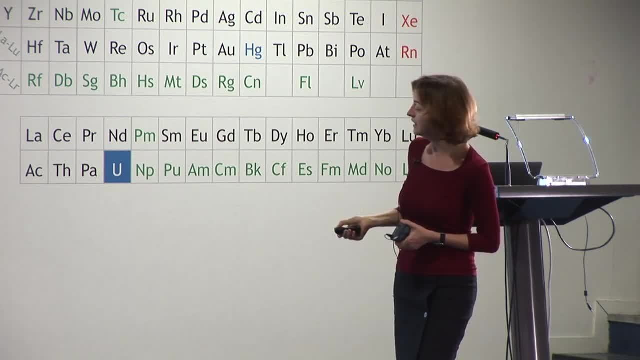 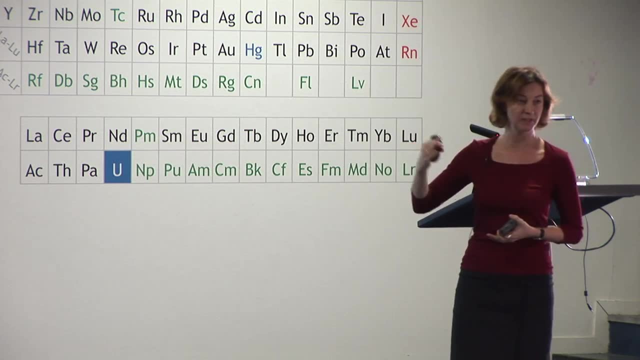 And this is why, For this local density, the errors are still quite large. so, about a factor of two, It is somewhere, even though there are quite a lot of papers and a lot of groups pretending they can give a much more precise value. 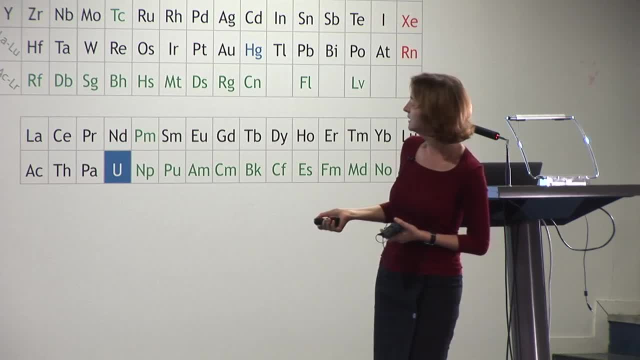 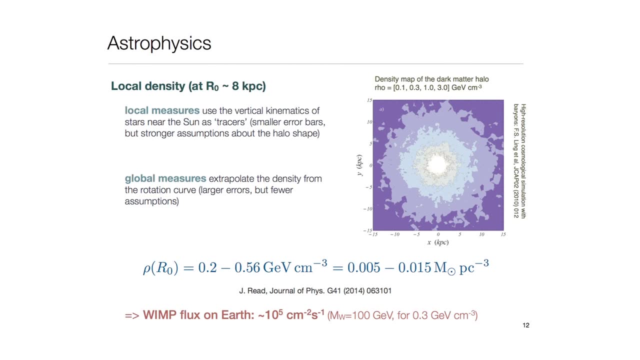 This is, by the way, a review here by Justin Reed from last year, So it's a very nice survey of this field. So you have about 0.2 to 0.6 or so GV per cubic centimeters, or, if you're an astrophysicist- 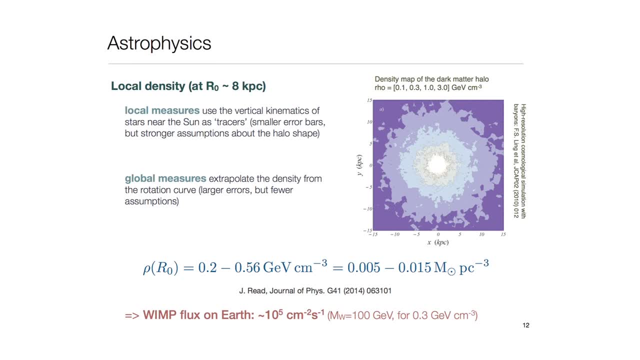 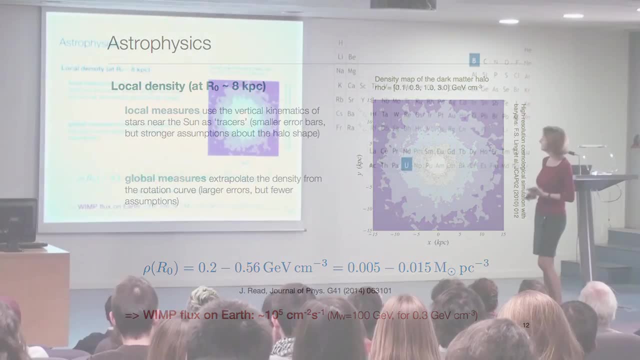 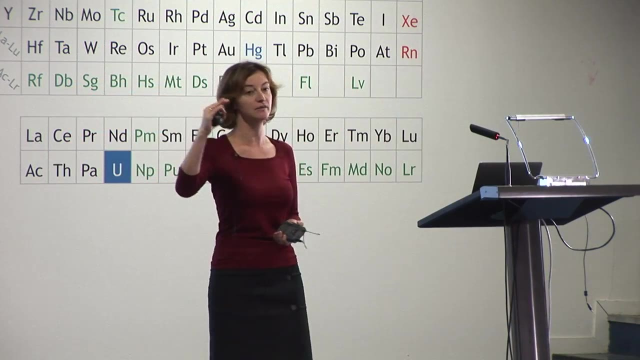 you probably prefer solar massive per masses per cubic particle. Okay, Okay, So this is the promo 터 seg. So now the question is: what does this tell us? What does this number tell us as a particle physicist? Well, so if you now assume some central value here, that we all take a sort of canonical, 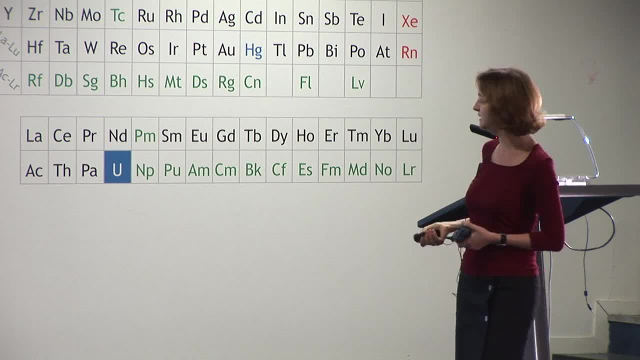 value to compare the results of areas, experiments and give actually some number on the cross section, because what we measure is a rate. as I already mentioned here, We don't actually measure the cross-section, but we measure a rate and if you make some, 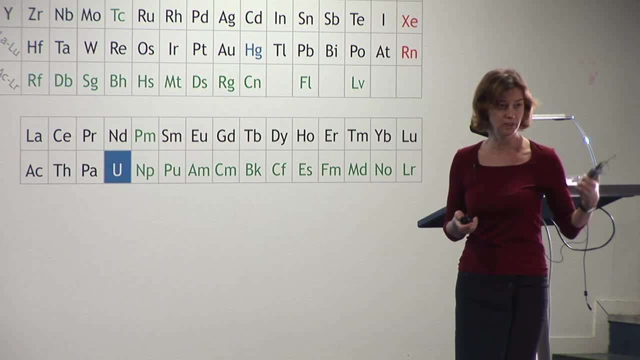 assumption about the local density, then we can give some constraints later on on the cross section. So if you take now the central value and the WIMP mass of 100 GeV, then I calculated this- You get about 10 to the 500,000 WIMPs. 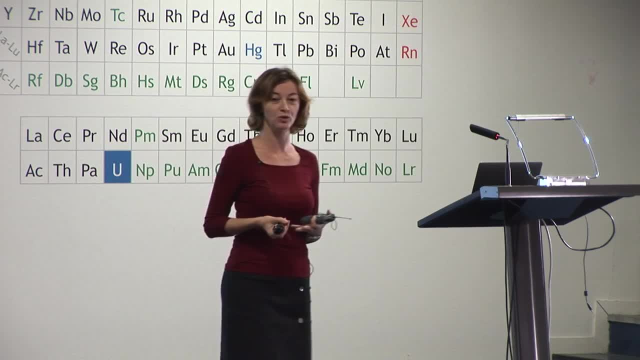 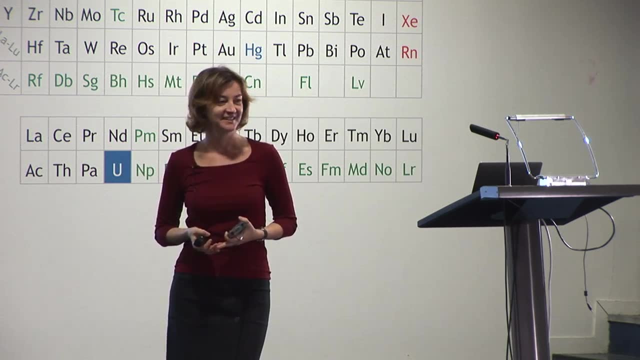 per every square centimeters and per second flying through you. So now does this seem like a big number or a small number? Big, Small? I will compare it with neutrinos. Yeah, Maybe you can compare with neutrinos. So what is the flux of PP, neutrinos? 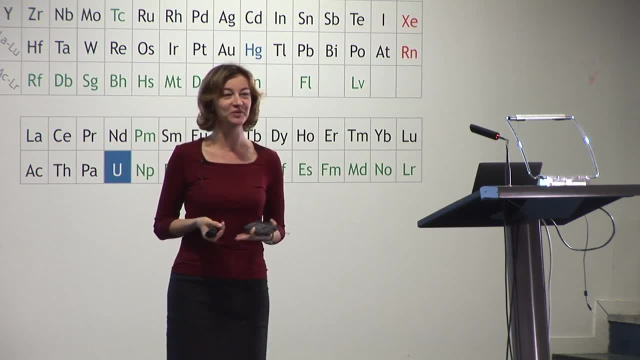 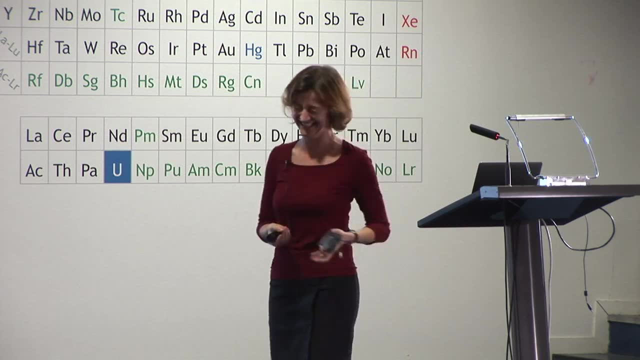 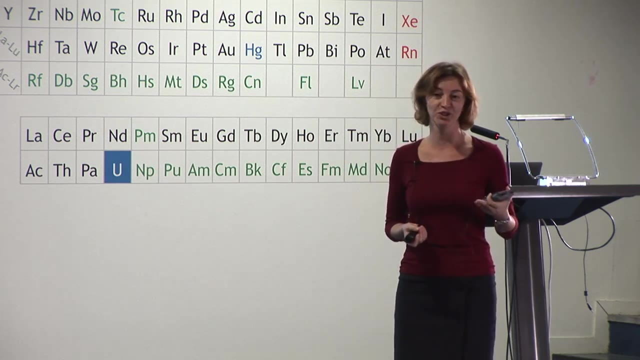 I have no idea. So does anyone know the flux? These are the PP neutrinos in the first reaction in the sun, I think Yeah, So it's 65 billions per square centimeters. and second, And as you know, those neutrinos are really hard to measure. 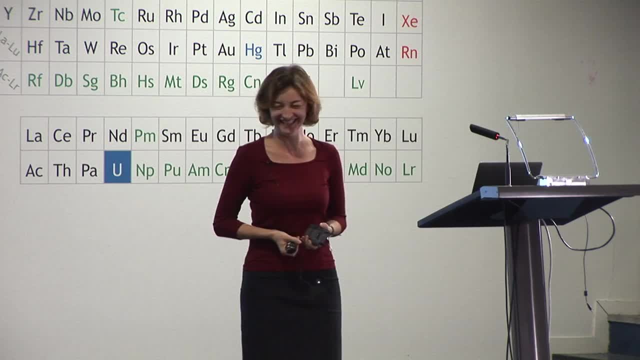 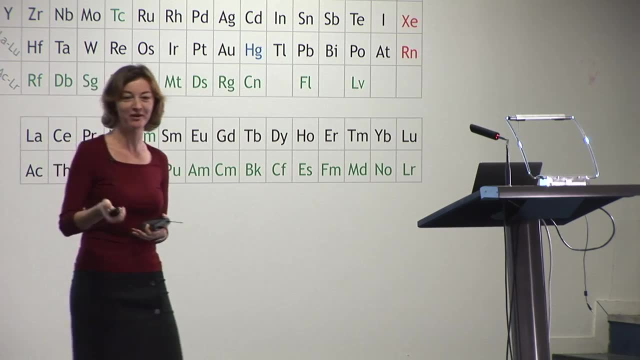 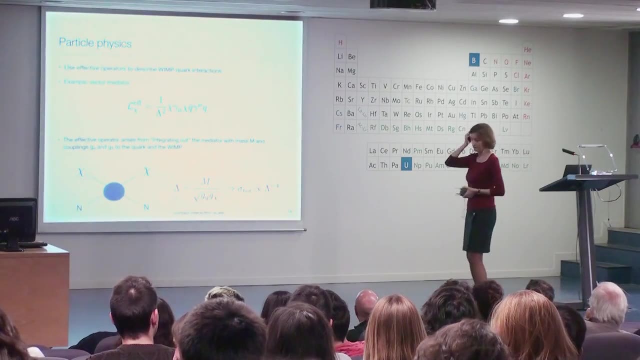 And this: This is a much smaller flux, but it's not zero, hopefully. And now, depending of course on the cross section, there is also a non-zero probability that we might observe these particles in the laboratory. So from particle physics, so for direct detection in general. 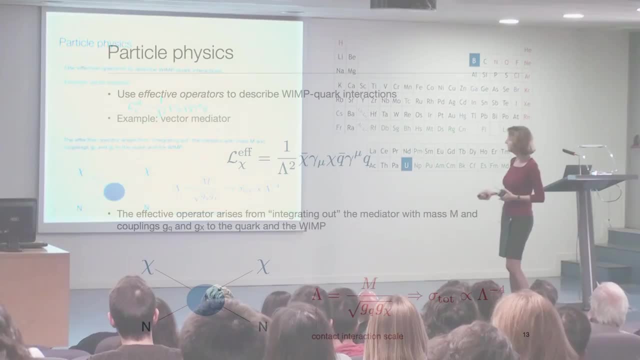 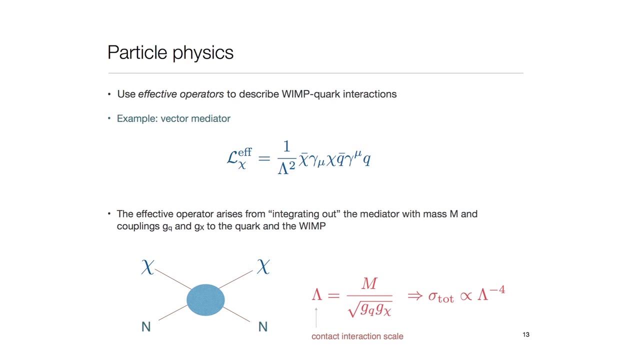 we use so-called effective operators to describe the WIMP quark interactions. For instance, you can have a vector mediator or axial vector mediator and so on. And this is here. This is just an effective Lagrangian where, just like in Fermi theory, you 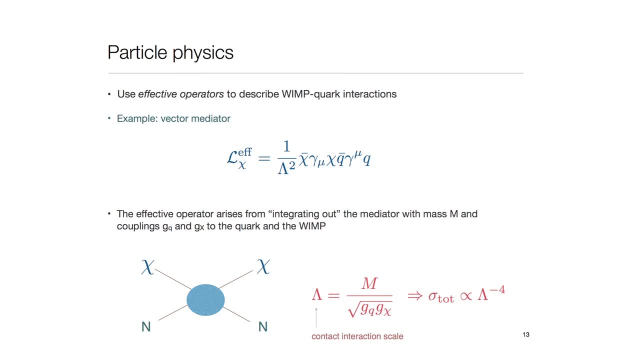 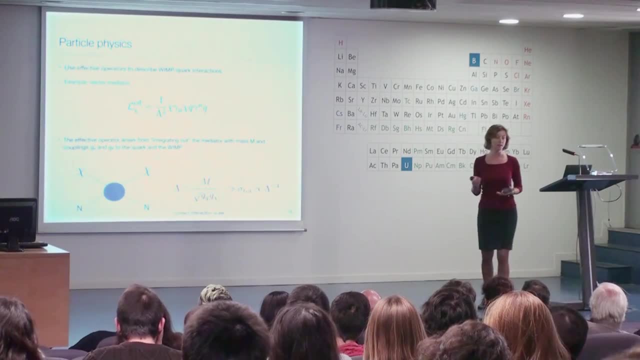 have this effector operator that arises from integrating out this mediator that you don't really know but that you can assume that has a certain mass and a certain coupling, on the one hand to the quarks and on the other hand to the WIMP. 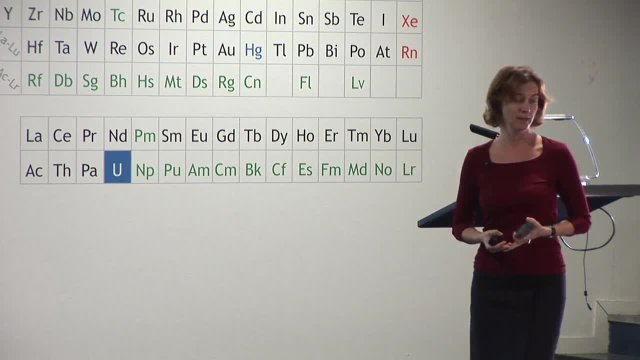 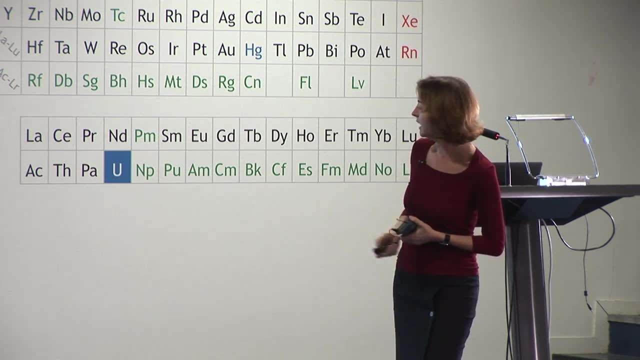 And this will be this contact interaction scale, just like the Fermi scale in weak interactions, where here again you have the mass of the mediator and these are the couplings, And then the total cross section will actually scale as 1 over this scale to the fourth power. 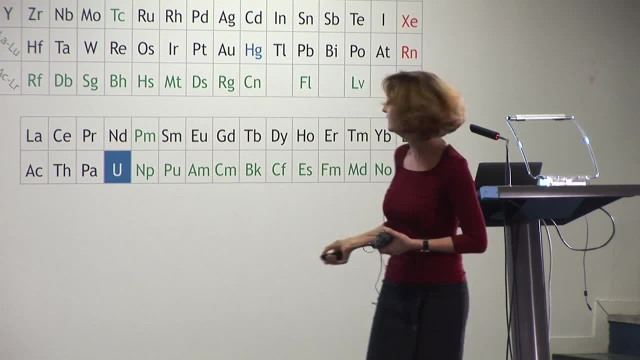 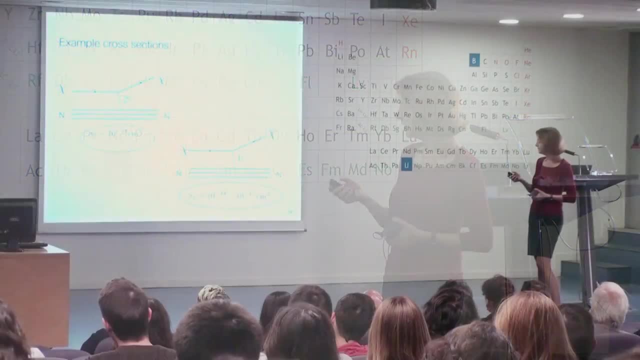 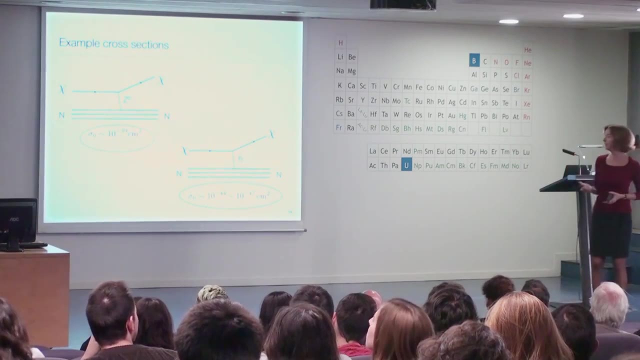 So you can see that, a cross section. you don't expect it to be large if this is somewhere around a TV or so Now just an example actually. So of course, very early in this field, the simplest idea would have been that such a particle just 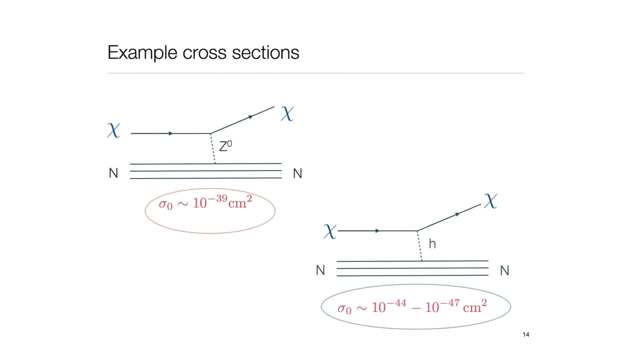 you know it's a particle. It's a particle that interacts via Z boson exchange. But then you can immediately calculate the cross section and it turns around to be 10 to the minus 39 or so square centimeters, And this is something that direct detection experiments. 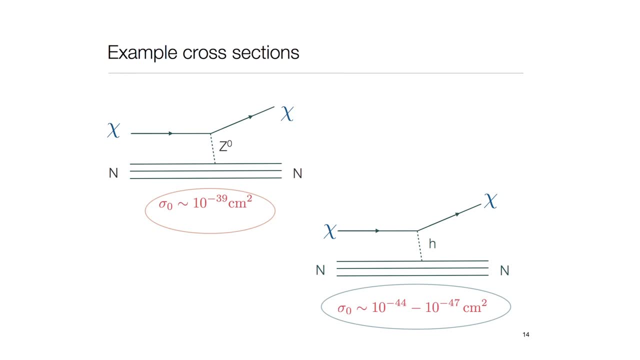 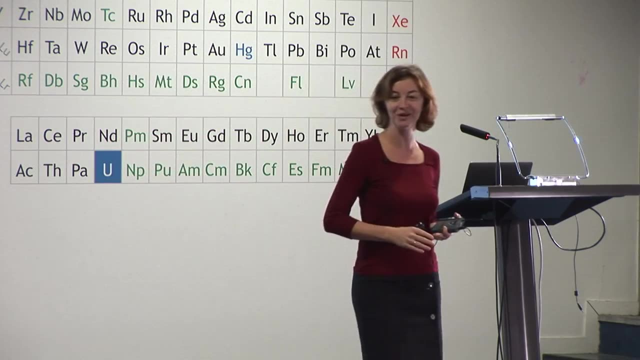 have excluded since many years Now. on the other hand, when you have something like Higgs exchange- and maybe you know there are all these so-called Higgs Porter dark matter models now, but they're roughly the cross sections that you predict- 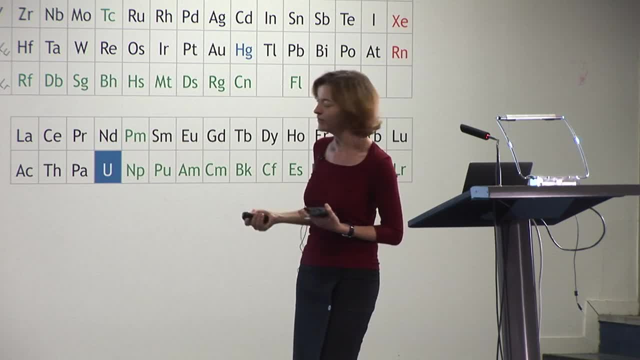 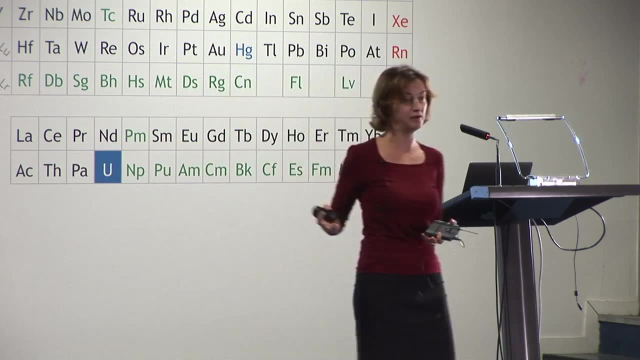 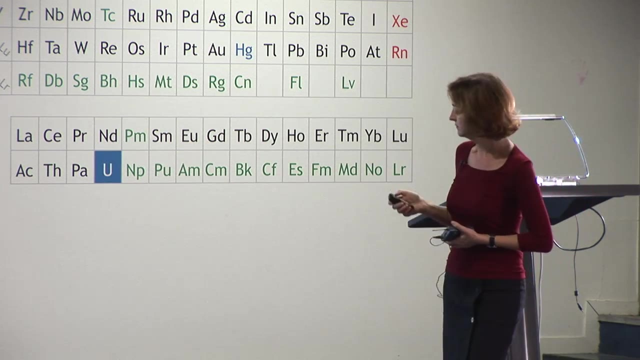 or that the theorists predict are in this range- 10 to the minus 44 or 10 to the minus 47 square centimeters- And this is actually good news, because this is the range that can be covered by experiments that are either already operating or will soon operate, you know. 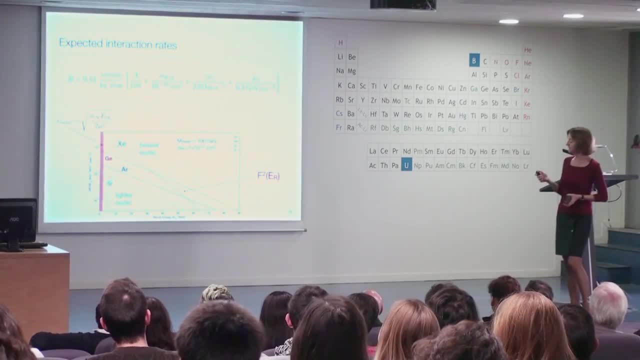 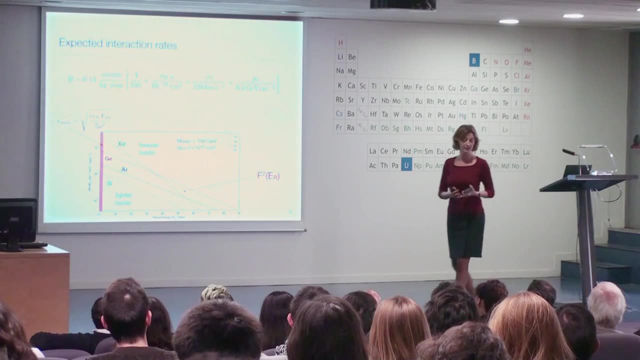 OK, so now if we integrate over all that we know, then what do we get for the total rate? It's about 0.1 events per kilogram of your detector material and per year. So again 0.1.. Again, it's a very small number. 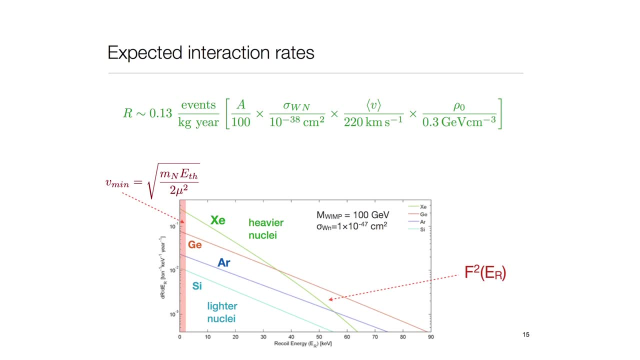 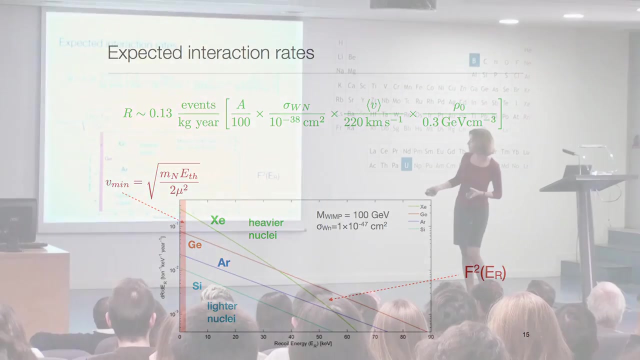 Modulo, all of these, You know, mass number of 100, this cross section, which is obviously smaller than the mean velocity of the WIMP, and here the local density. And what I'm showing here is now this differential rate as a function of the recall energy. 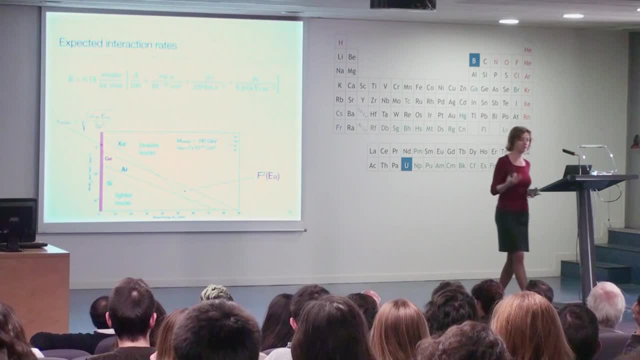 So this is a logarithmic scale for several materials that are used in this field, So the detectors that are made, for instance, of xenon, germanium, argon, silicon and so on. So you have some enhancement here because of the heavy nucleus on the one hand. 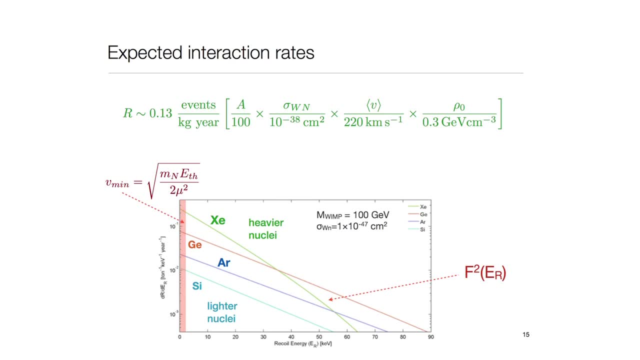 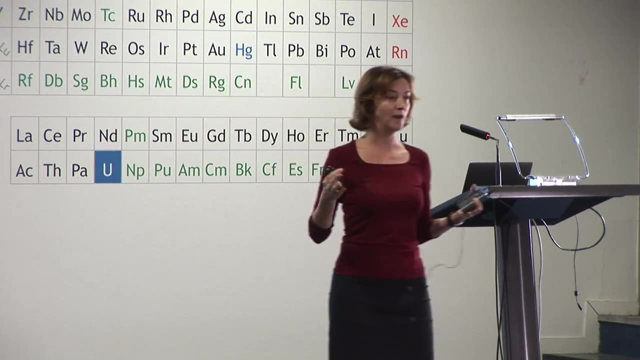 On the other hand, as I'll show you, you also will have to deal with form factor corrections, Because the WIMP doesn't scatter on quarks, but it actually scatters on the entire nucleus. However, for WIMPs in the high velocity, 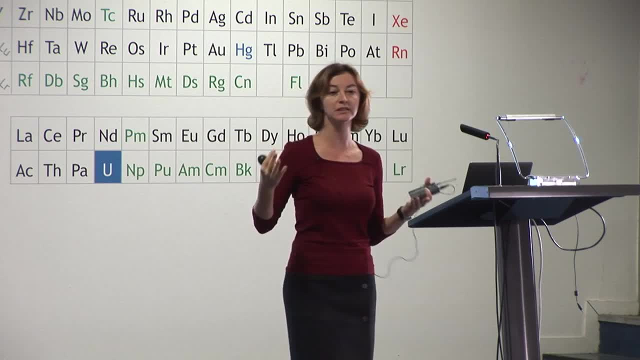 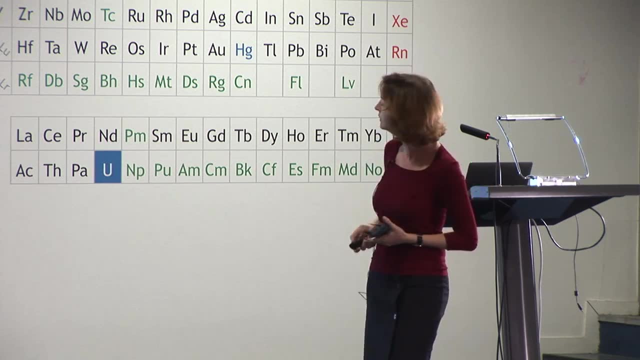 tail of the distribution and also for larger nuclei, you can start to resolve individual nucleons. OK, So these form factors will actually play a role And luckily, oh, I actually meant to say something. maybe I'm not sure if it comes, but I'd just 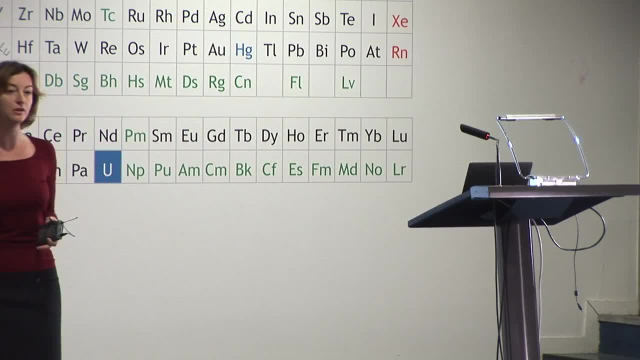 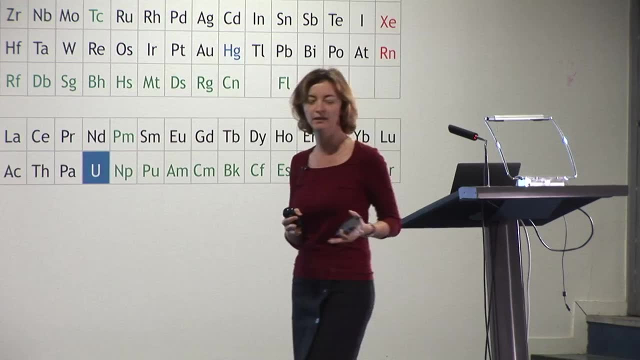 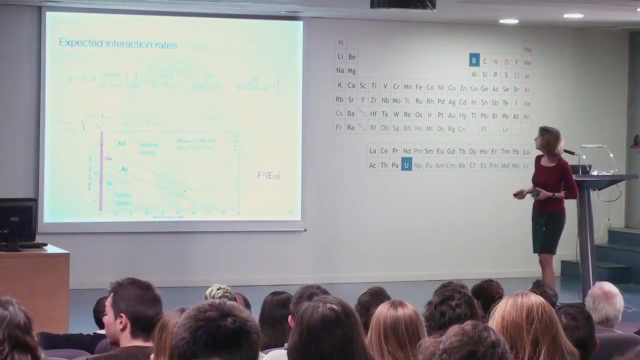 like to say that there are quite a lot of nuclear theory groups now that look again at these form factors and actually calculated them both for spin-dependent and also for spin-independent scattering, for actually all the nuclei that are relevant in direct detection. OK, so now there's quite a zoo. 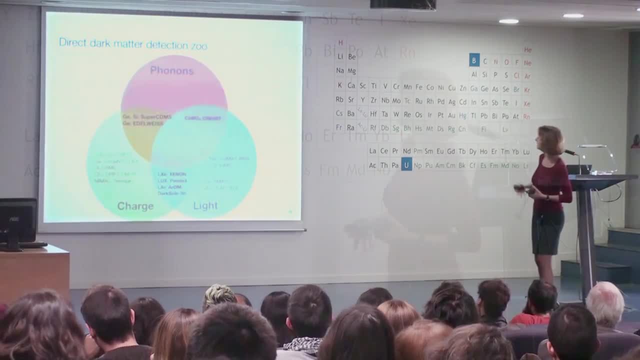 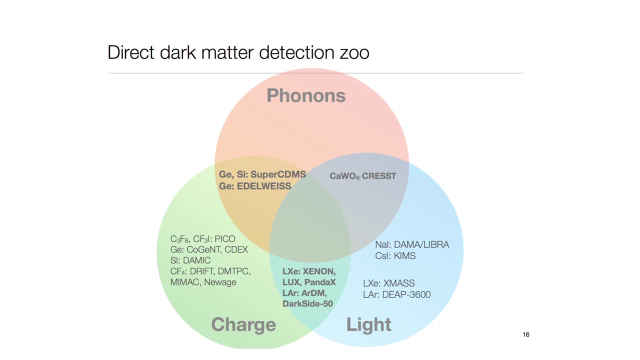 There's a lot of experiments because, as you can imagine, it's a very hot field. So we have this recall energy somewhere that is very small that we are trying to detect, And then we use experiments that are based on phonon readouts. 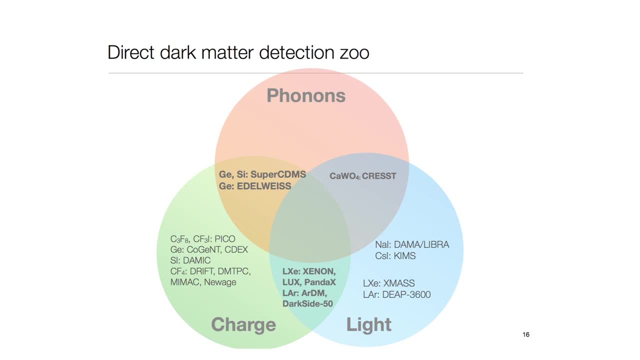 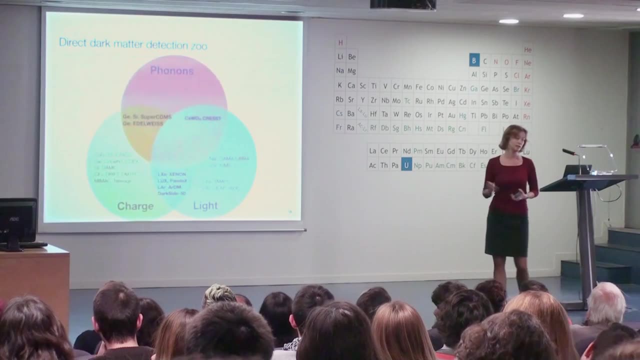 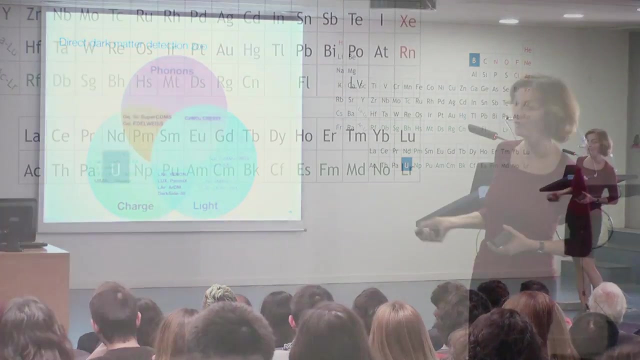 or lattice, vibrations or charge readout. These are ionization-based experiments or light, namely scintillation experiments, And many of the modern detectors try to detect, for instance, both phonon and charge, or charge and light, or phonons and light. 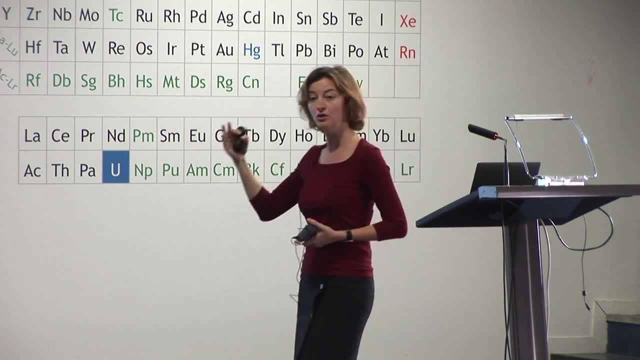 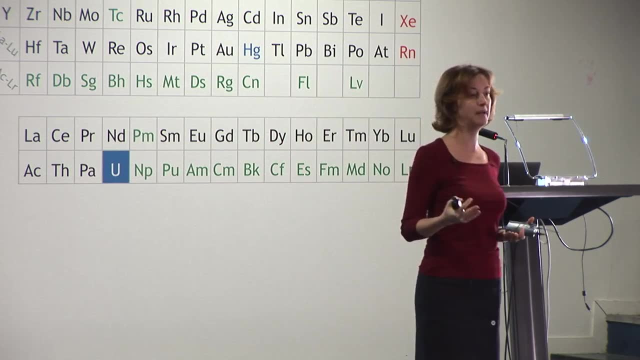 And why? Because the ratio of these two quantities, for instance, will depend on the ionization density on the e over the x, And that again will depend on the type of particle interaction in your detector. So that will allow you to reject a large part. 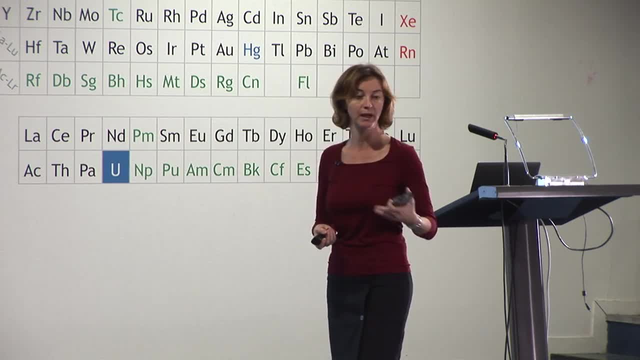 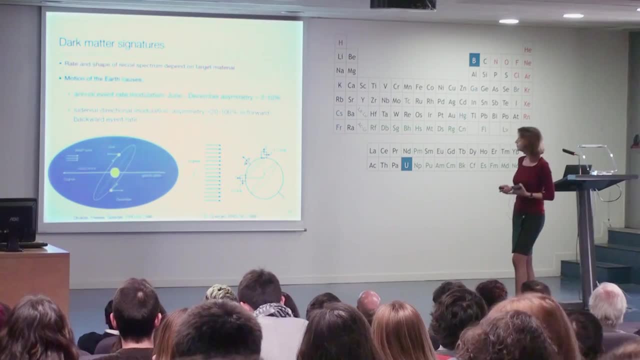 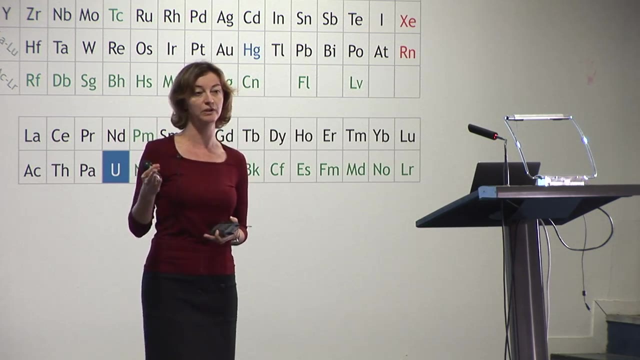 of the background that is mostly of electromagnetic origin, so gammas, betas and so on. Obviously, I cannot go through all of these detectors, OK, But I should mention that, apart from this, what I've shown you, that is rate and also the shape of the recoil spectrum. 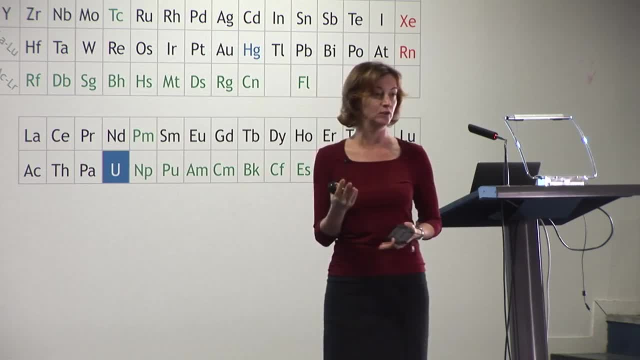 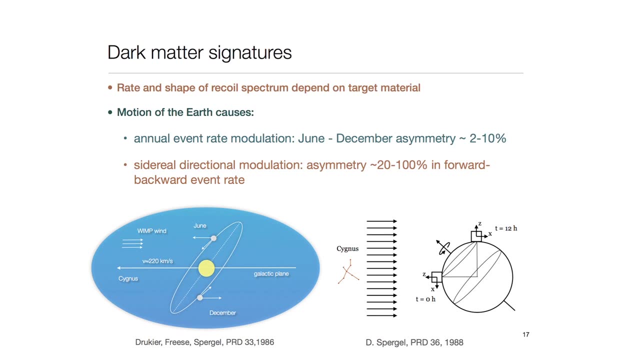 depends on the one hand on the detector material, on the other hand also on the WIMP mass. I haven't actually shown that. We'll come to that later. We also have some specific signatures for a dark matter particle that is in the halo of our galaxy. 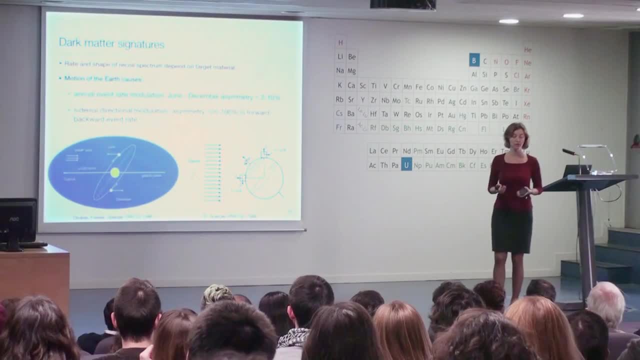 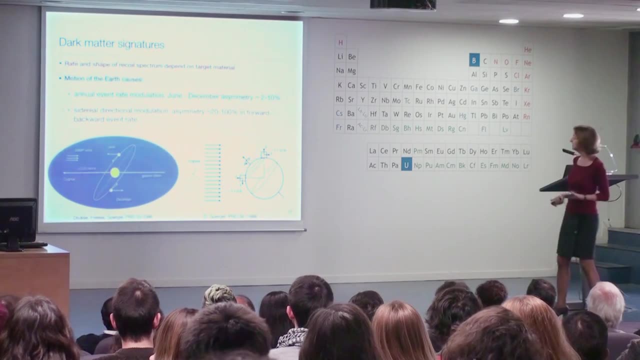 And that is, on the one hand, an annual event rate modulation. So you can imagine this. So you have an asymmetry And you can see it in the rate between summer and winter. And this comes from the fact that, on the one hand, 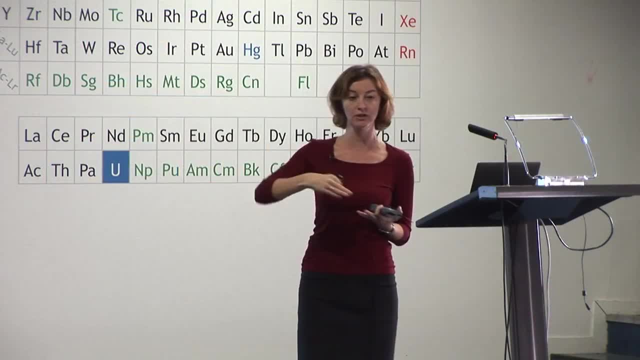 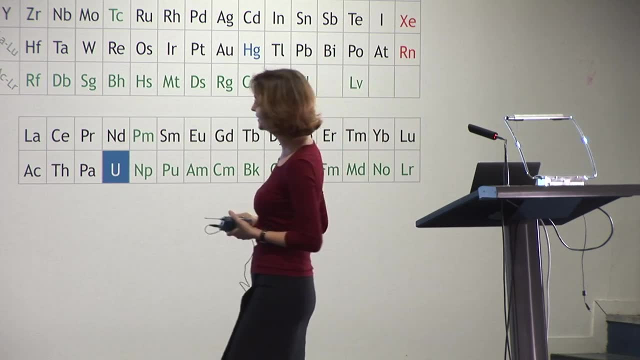 we are moving together with the sun Towers. here are constellation signals, So we are moving around the galactic center, But also the Earth is actually moving around the sun, as we know, And in June the two velocities are mostly aligned, so parallel. 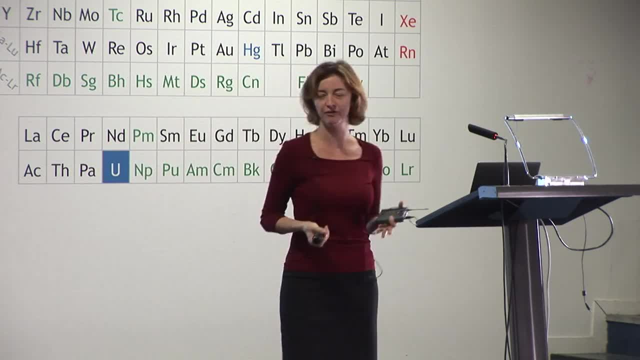 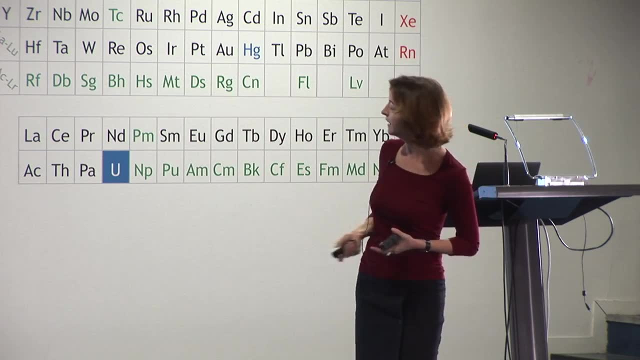 while in December they are anti-parallel. However, it's a very small effect, because here the Earth moves only with around 30 kph And then also this plane is inclined. So you can take about 15 divided by 220 or so. 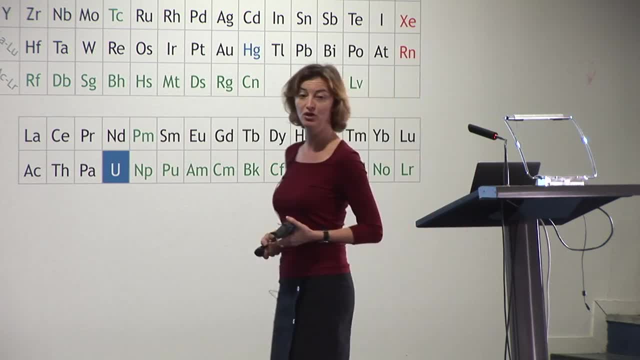 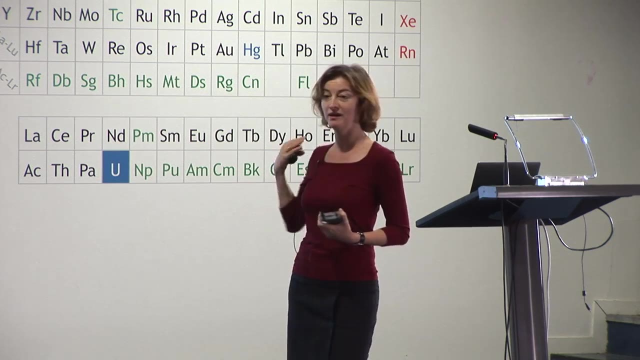 So it's only a very small effect, But that is potentially observable And actually there is one experiment that claims that they have seen this effect. On the other hand, because the Earth rotates on its axis and again we move here together with the Earth, 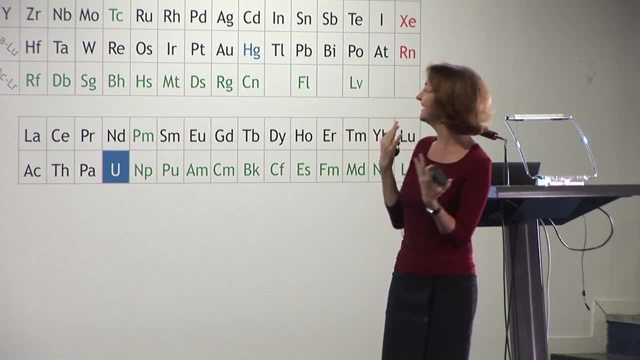 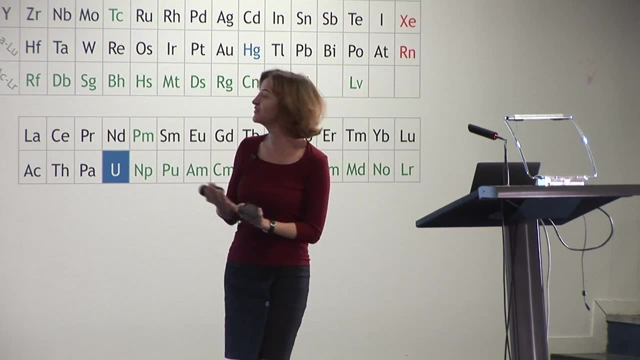 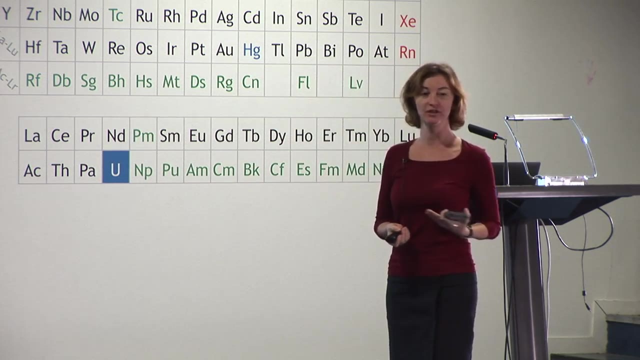 we feel this WIMP-WIMP- I guess you feel it too, And at least I feel it all the time- Then we can also look at a symmetry in the forward-backward direction of this incoming WIMP, And this is a much larger effect on the one hand. 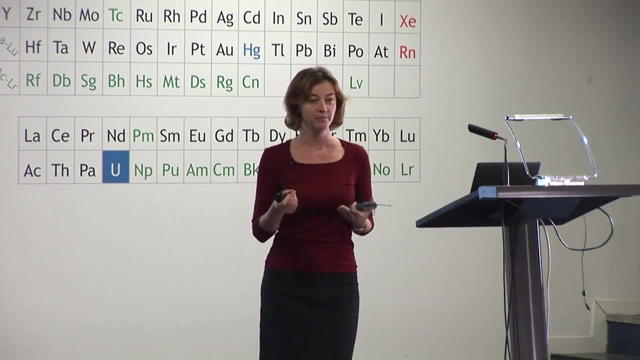 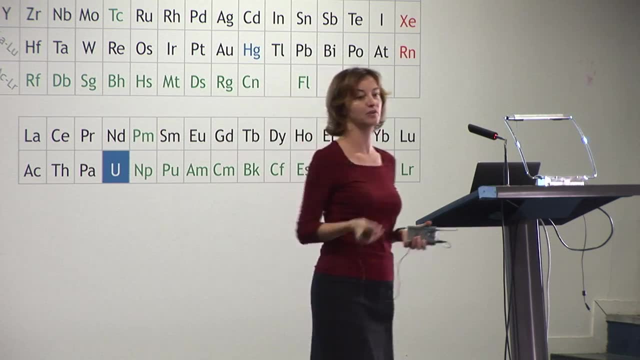 But on the other hand it's a very hard effect to measure because you have a very low energy nuclear recoil And the track will be in a solid or in a liquid. the track will not be measurable, So you have to have low-pressure gas. And if you have a lot of energy, you have to have a lot of mass in order to be able to measure that. That is conflicting with the fact that you need a lot of nuclei, a lot of mass, to get your event rate to some reasonable number. 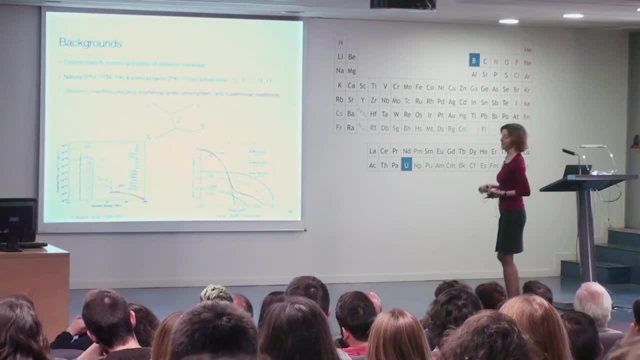 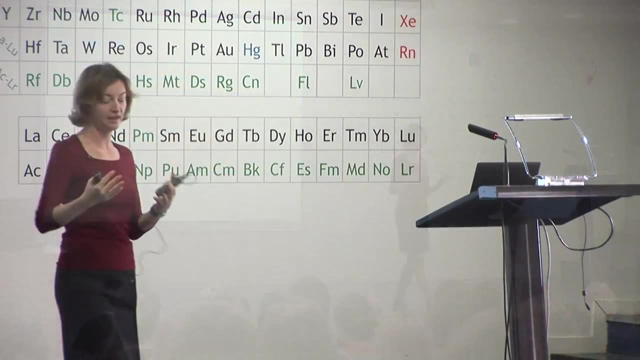 like one a year at least. But anyway, these signatures are there And we might look for them, But then we have a lot of background. So in astrophysics, of course you also have a lot of foregrounds, backgrounds and also 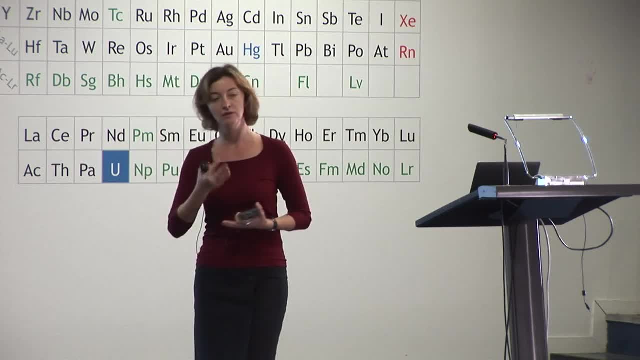 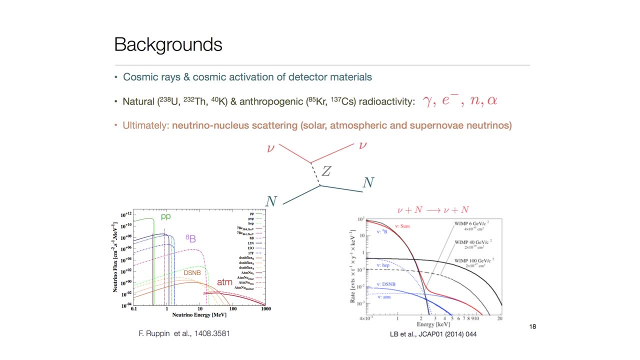 in particle physics experiments And we also have to deal with them. We have to deal with the activation of the detector materials by cosmic rays, And to deal with cosmic rays we go deep underground, as you will see. Then we have radioactivity. 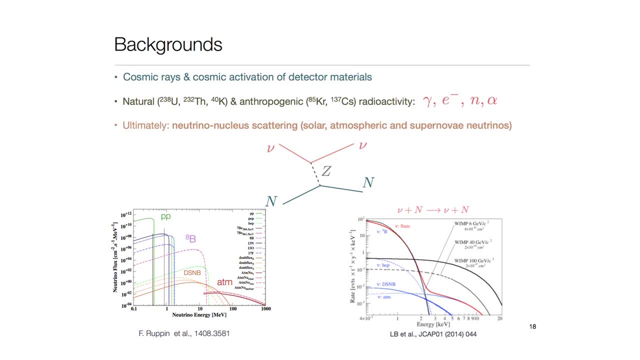 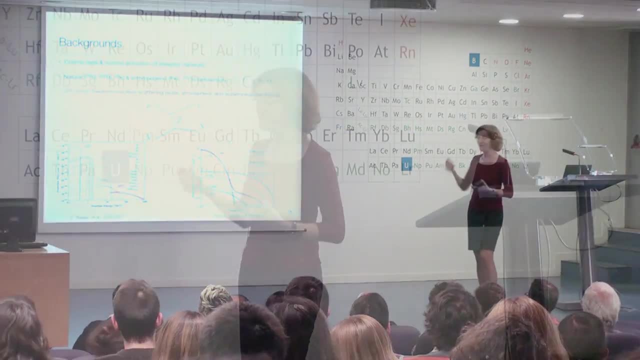 We have the natural radioactivity that's just everywhere, So uranium, thorium, potassium, and then man-made radioactivity. that is also lots of it up there in terms of krypton in the air. That's a big problem, for instance. 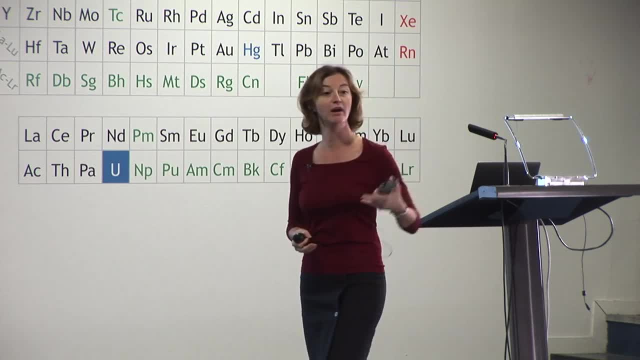 for xenon-based experiments That comes from Fukushima, from nuclear bomb tests and so on, but also cesium, And these give you gammas, betas, neutrons, alphas, everything And the most dangerous for dark matter, at least for WIMP dark. 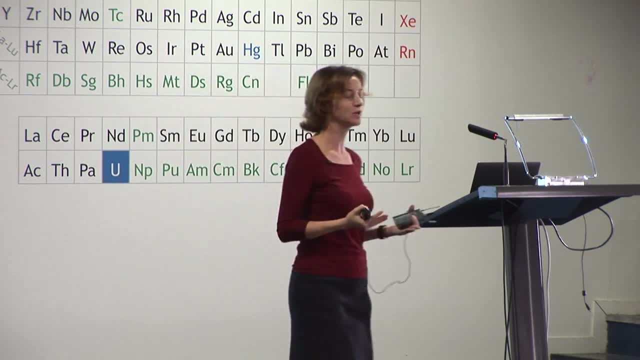 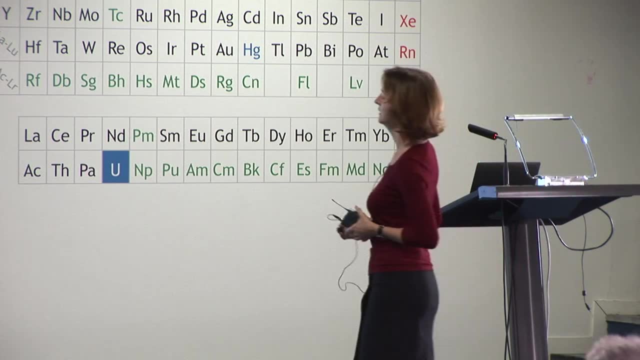 matter searches are neutrons, because fast neutrons will also give you nuclear recalls in the same energy range where you are looking for a WIMP. However, ultimately, and when I started in this field, which, as you can imagine, was a very long time ago, 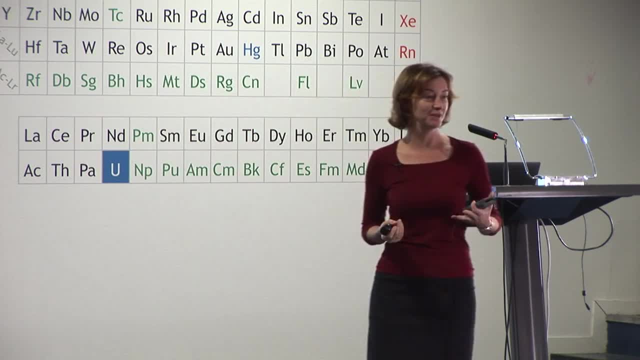 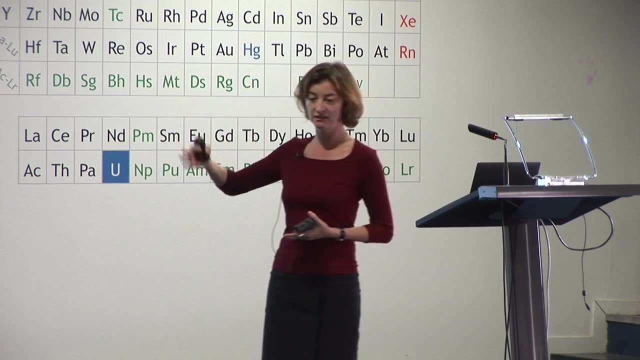 I didn't think that neutrinos would be our ultimate goal, Right Right, Our ultimate background. So we have to deal first of all- I'm not showing it here- we will have to deal with neutrino, electron scatters from the PP, neutrinos. I told you already that the flux is very high And even though most experiments can discriminate between interactions from electrons and or electronic recalls in your detector, on nuclear recalls, the discrimination is not perfect. There's nothing 100% in physics, so you have a certain efficiency. 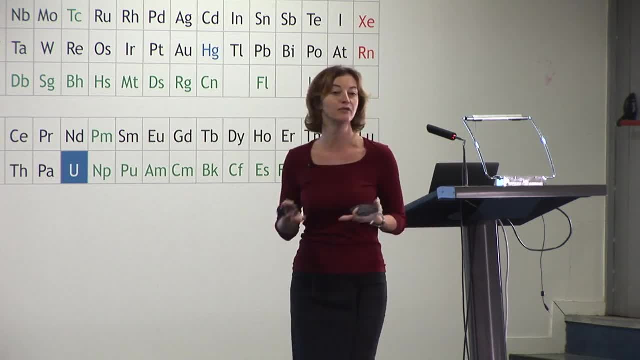 and you can misidentify, for instance, a neutrino electron scatter for a nuclear recall. But ultimately this is again the neutrinos that are measured from the PP neutrinos to 8, beryllium, atmospheric and so on. 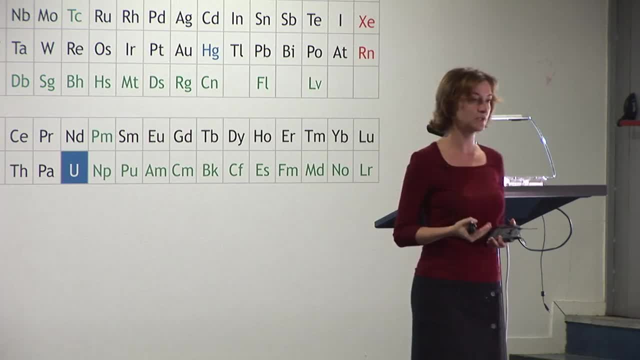 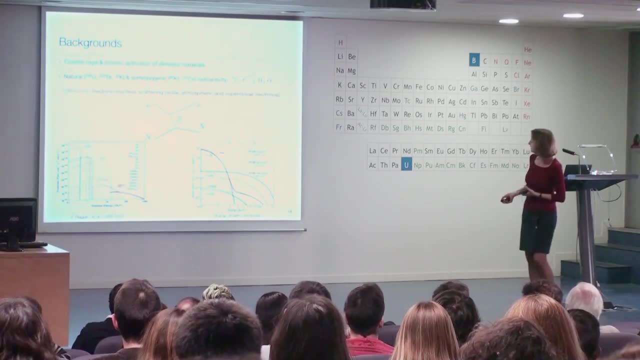 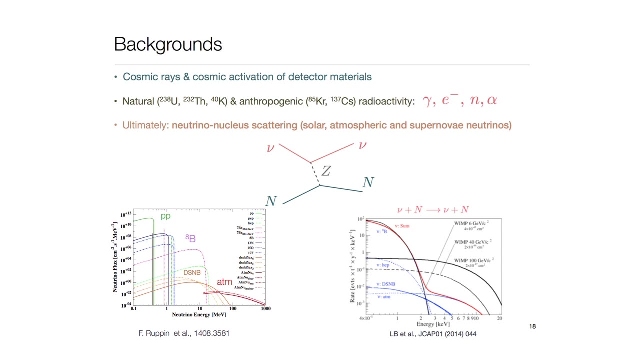 Ultimately we will have coherent neutrino nucleus, scattering that is. you know, it's a standard model process, even though it wasn't observed yet in an experiment. And if you look here, so, for instance, the solar bore 8 neutrino will just look like a 6 GV WIMP or so, and pretty soon. 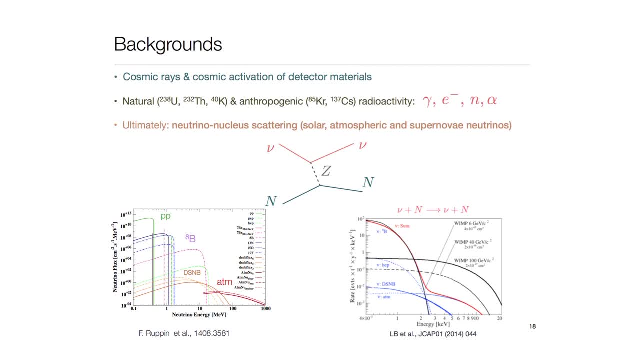 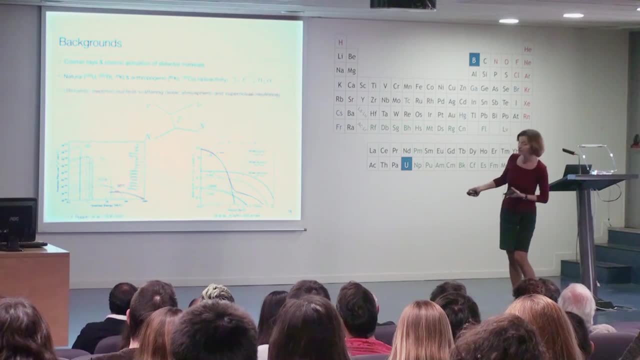 already at the cross-sections of around 10 to the minus 45 or so square centimeters, while as you go to higher here in energy, you will have the atmospheric neutrinos and also the neutrinos from the diffuse supernova neutrino background. 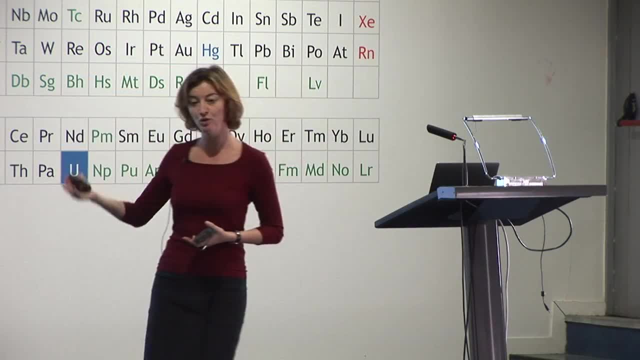 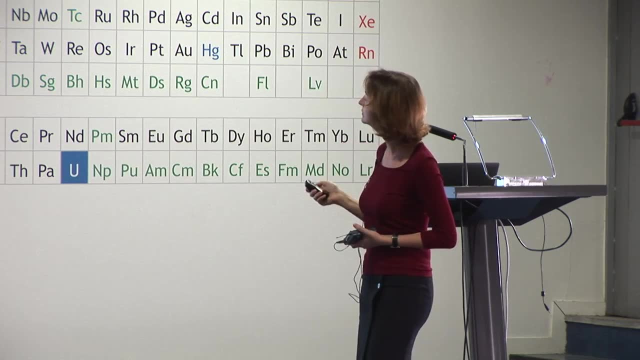 That could mimic, for instance, higher mass WIMPs. But, as I will show you later on, there we have about from today, let's say, about four orders of magnitude to go until we hit that background. OK, so how do we deal with the background? 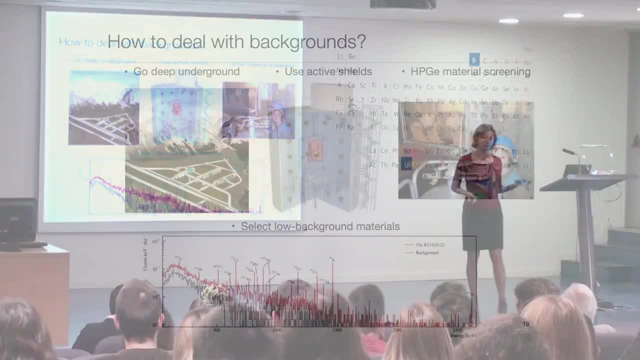 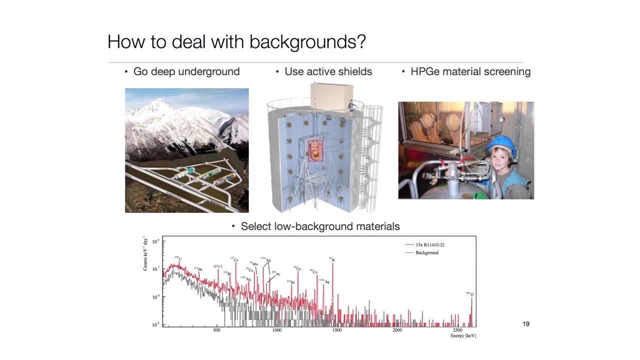 I already told you that we have to go deep underground, and there are many underground laboratories in the world. I work here in Gran Sasso, which is in Italy, but there is also an underground lab here in Spain, the Camp Frank Laboratory. 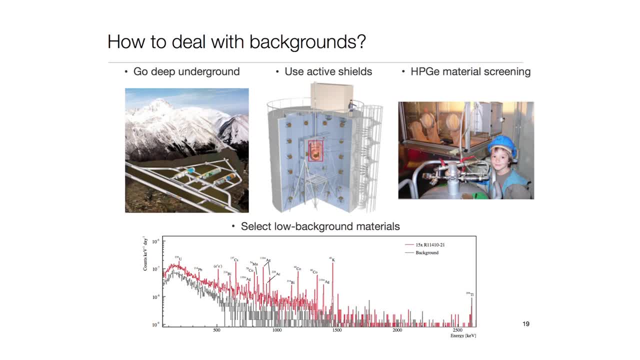 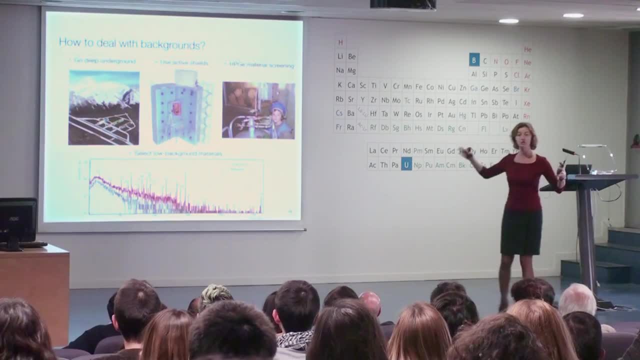 We have to use active shields even though we go underground, because the walls of the lab, the concrete, the rocks, and so they provide a lot of radioactivity. And most modern detectors use now large water Cherenkov shields, because the standard shield you cannot. you know. 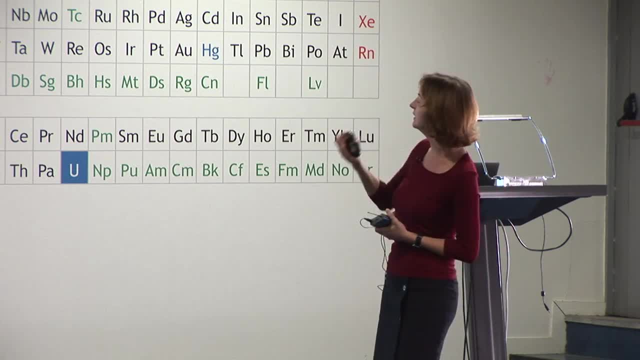 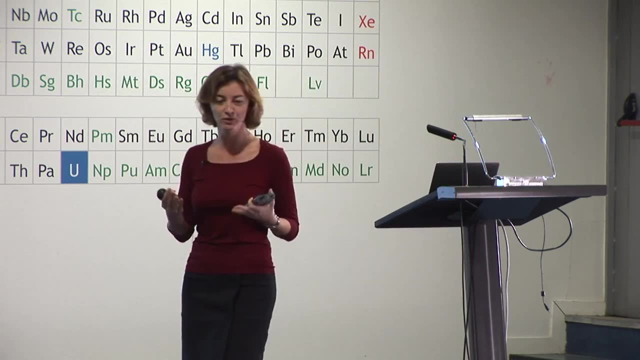 they become too heavy, Too expensive to use- lead and poly and copper and so on, And we also have to screen a lot, basically every single material that we are using in our detector. This was here my son, many years ago. 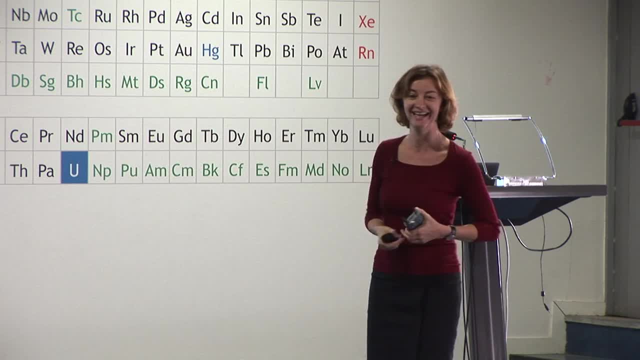 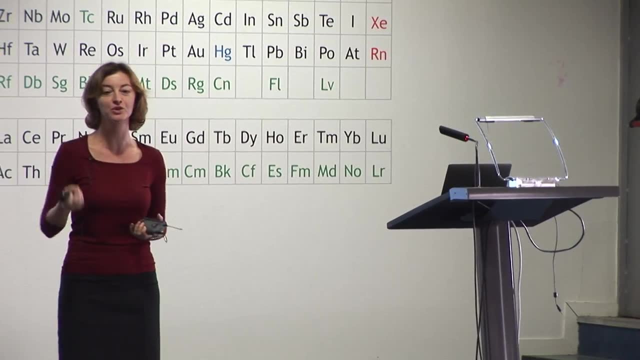 So he had to help because there is actually a lot of screening work to be done in any of these experiments You can imagine- I will show you later the Xenon-1 tone detector- but we had to screen every little screw that is in that experiment. 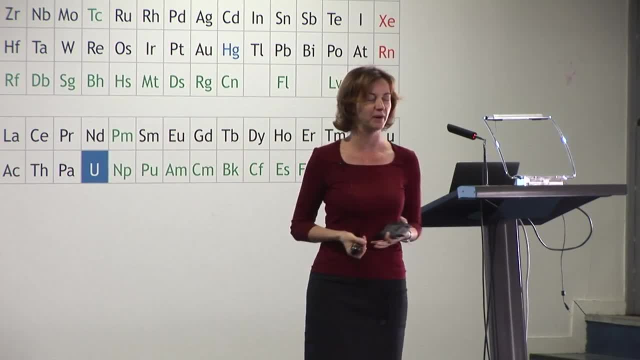 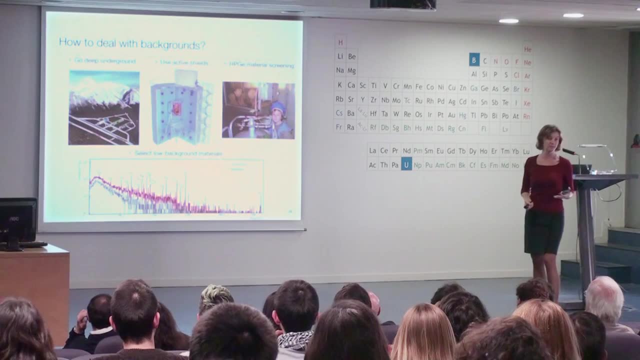 And even only the inner detector has more than 1,000 parts. So we have to select very low background materials. I'm showing you here just the germanium spectrum. We use germanium detectors because they have very low intrinsic background, But also they have a very high energy resolution. 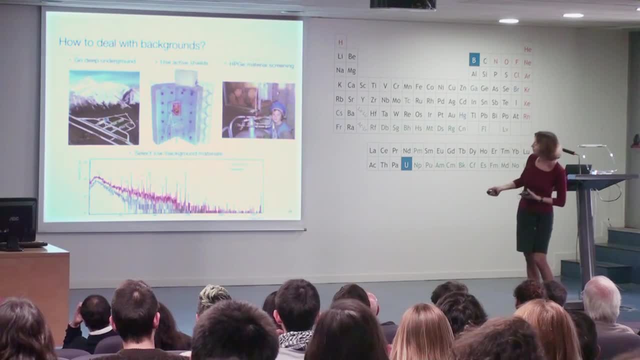 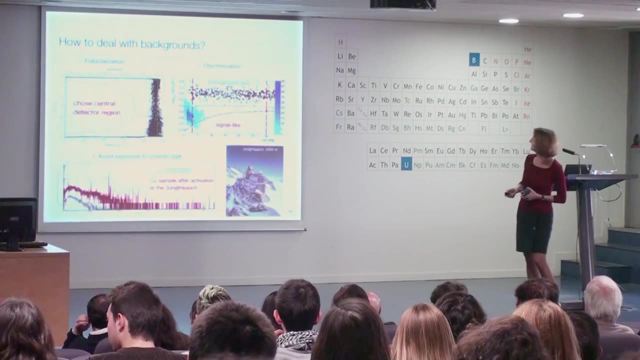 that allows us to identify all these lines. These are 15 photo detectors in Xenon-1 tone, So you see a lot of these lines there. So, anyway, you have to deal with them Now. also, how else do we deal with backgrounds? 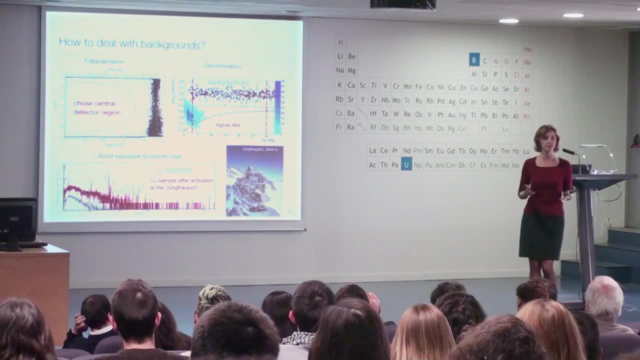 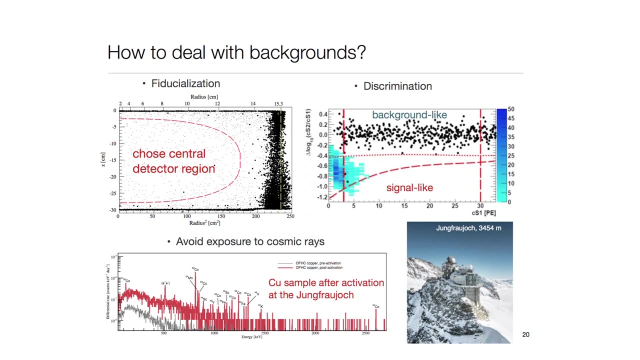 Well, we have what we call fiducialization, Very similar to neutrino physics. A lot of our background events will be here, at the outer regions of the detector, So you can define an inner region, an inner fiducial region that is hopefully close to background free. 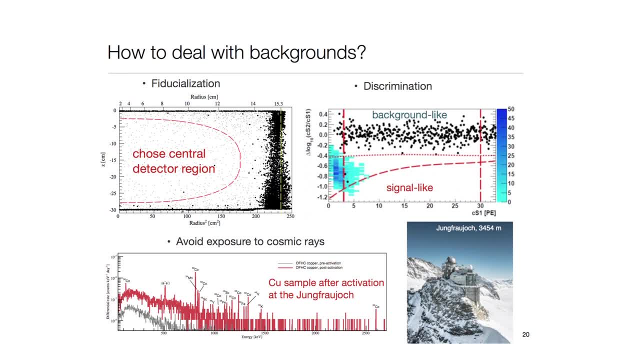 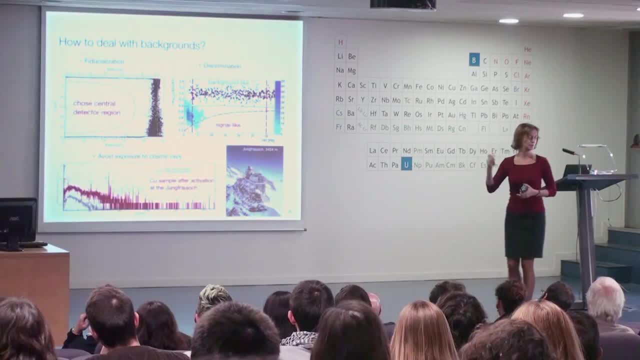 This is here just data from the Xenon-100 detector. We use discrimination. This is what I mentioned In this case. here, what we show is the ratio of a light- sorry of charge- to light in a detector. So you have a population. 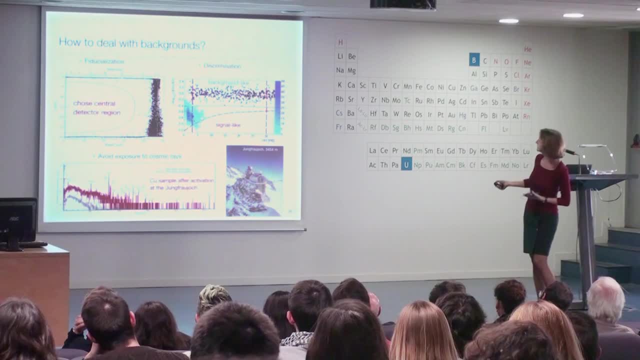 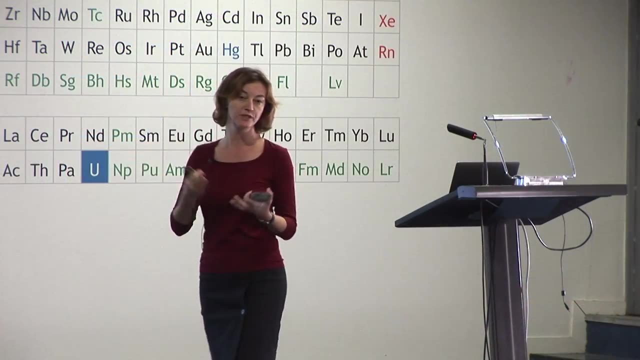 You have a population that you define as background-like events, For instance here electronic decoys And here signal-like, And also, as I mentioned, you have to avoid to expose, in fact, your detector materials to cosmic rays. 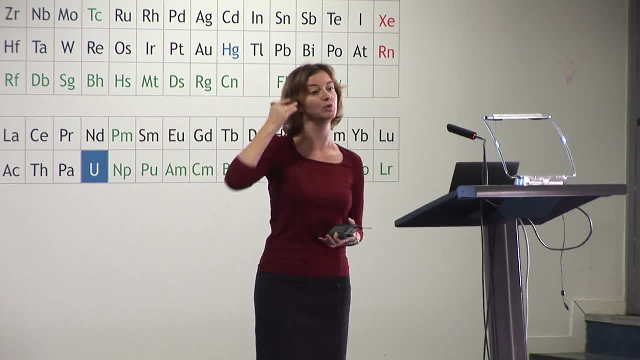 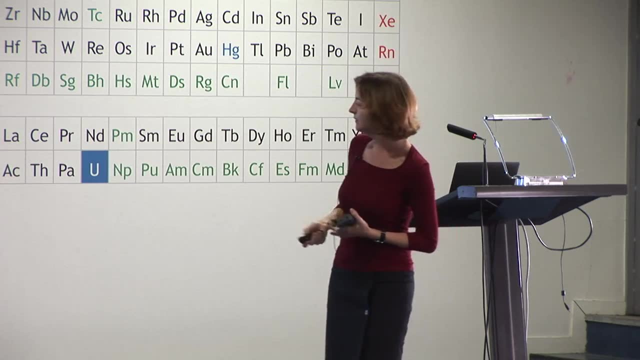 Because palation reactions by high energy protons, neutrons, will produce, among other things, also nuclei with very long half-lives. And here, for instance, just an example: we brought some Xenon to the Jungfraujoch. 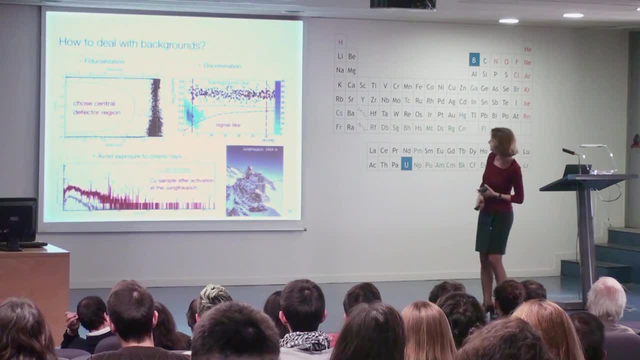 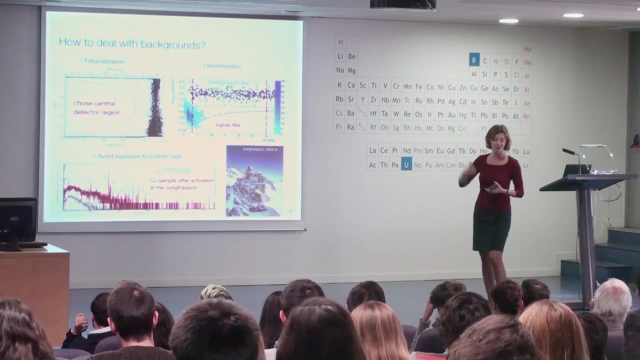 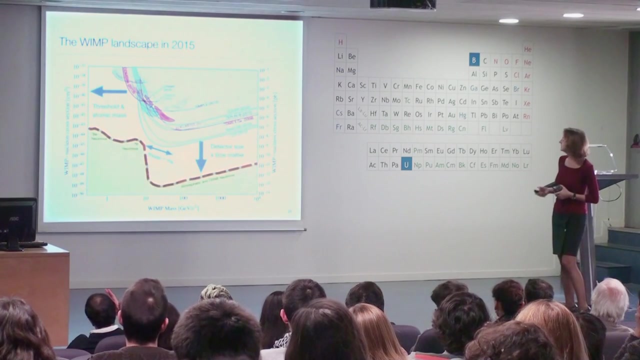 That's at 3.5 kilometers. But we also brought some copper. So you see here the copper before it was exposed to cosmic rays and then after it was exposed. So you produce a lot of stuff And that's why you really have to minimize the exposure. 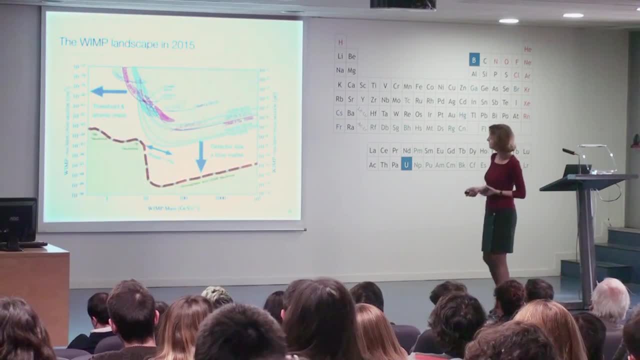 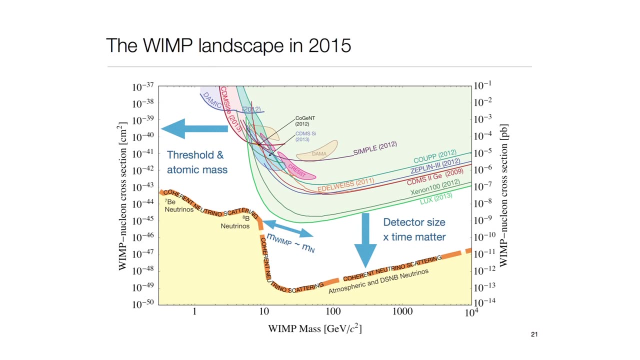 So what is actually this so-called WIMP landscape today? So what I'm showing here is a cross-section that is, however, normalized to a nucleon Again, so that we can compare different type of experiments using different type of nuclei, So normalized to a proton or to a neutron. 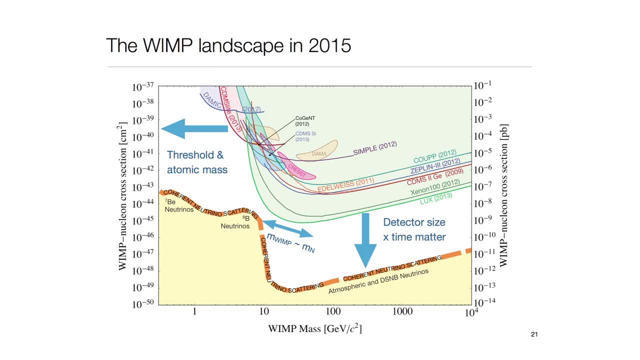 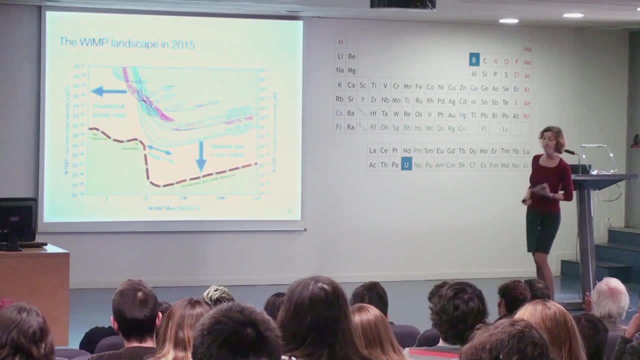 as a function of the mass of the WIMP And this region here. all of this is excluded by the current generation of experiments. This will be probed by detectors that have a very low energy threshold, Because for low mass WIMPs the nuclear energy 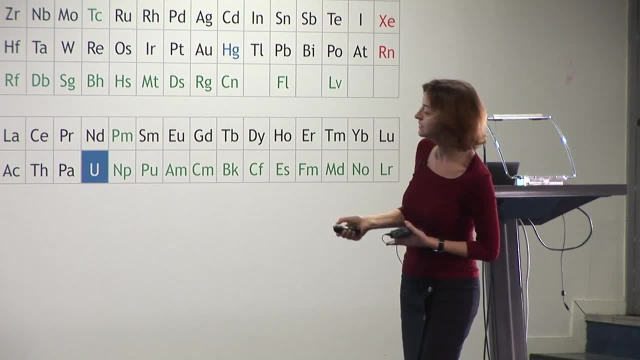 will also be much smaller. So you need that in order to address this region, While here it's mostly larger detectors where the size, but also the time, So the total Exposure will be important And because you might ask me, you see. 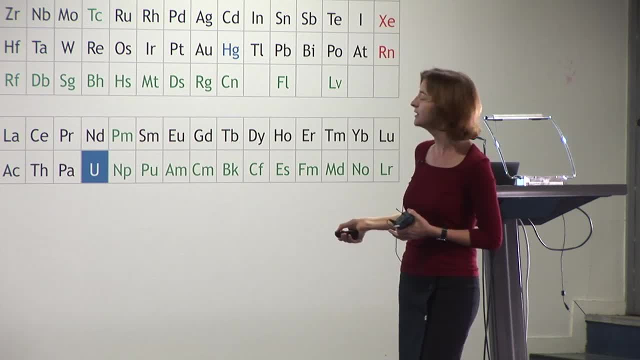 I'm not showing here any predictions. What I'm showing here is the region where at some point your rate will be dominated by neutrinos. But you may want to ask: well, what are actual predictions? And I'm showing here two from SUSY just as an example. 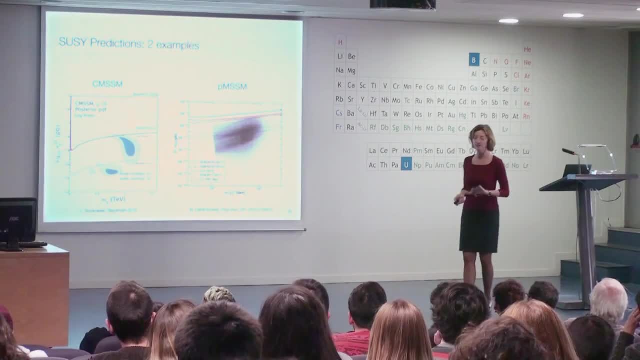 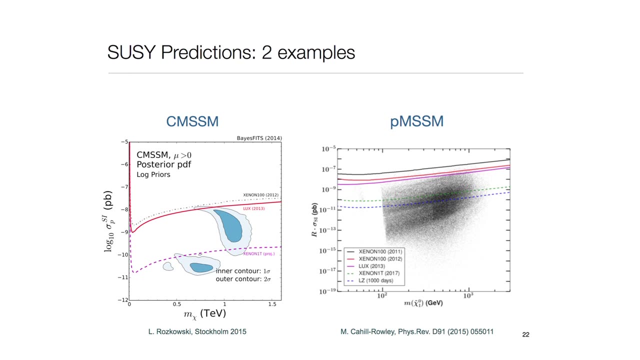 because there are zillions out there And this is a very constrained model, the constrained MSSM, And you see here, this was in 2014.. Well, after the last LHC data from the last run, you have here this region and also this region. 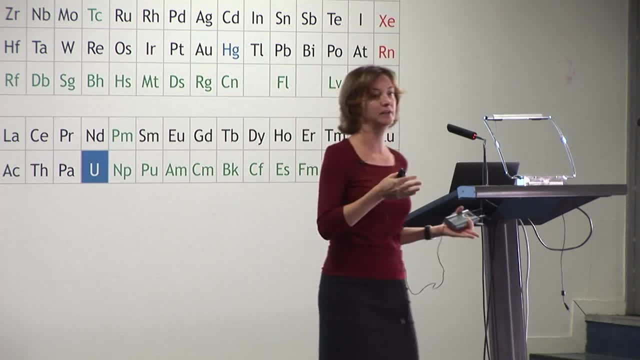 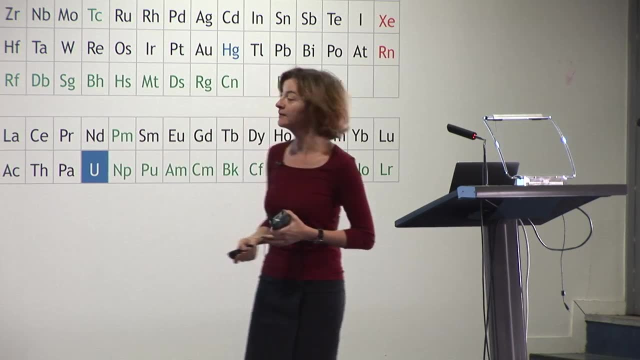 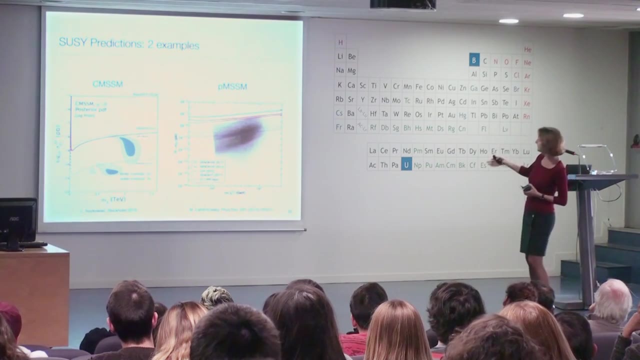 I should say that these regions, of course, with more data from direct detection experiments, but also from the LHC, over the years kept moving to the right and downwards, obviously, On the other hand, here from a paper dealing with a phenomenological MSSM, I think with 15 here. 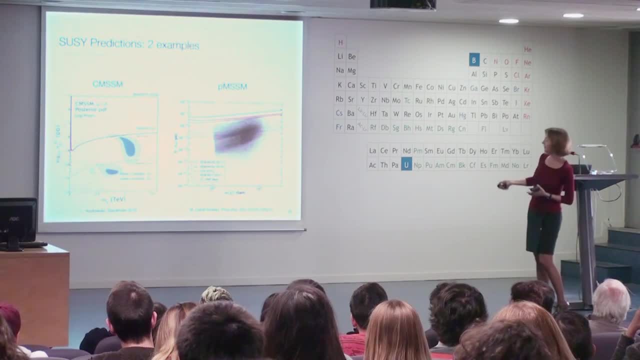 or 19 free parameters, where, of course, a much, much lower range. So you can see that This is a much larger space of the parameter space than opens up just because you have a lot of free parameters. So these are just some predictions. 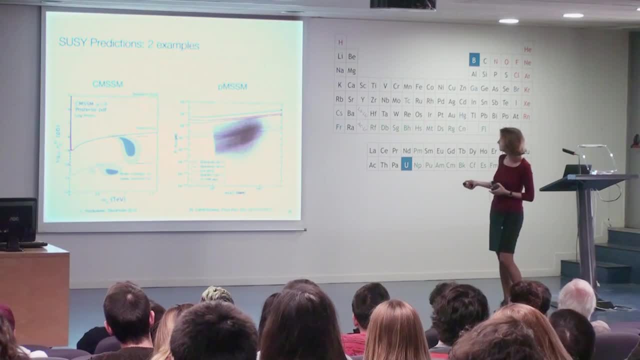 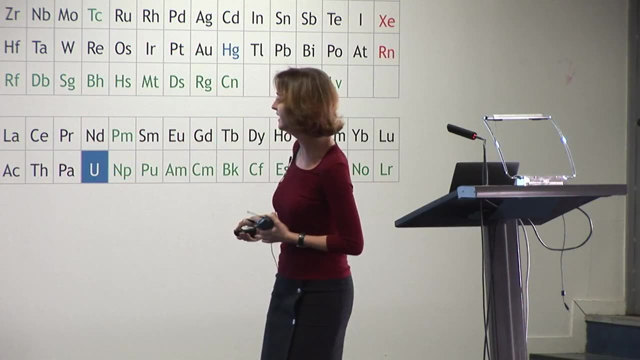 But I guess the point that I want to make here is that of course, there is a region of parameter space predicted where this next generation of detectors we'll look at, But on the other hand, it can also be much below, so even much below this background here from neutrinos. 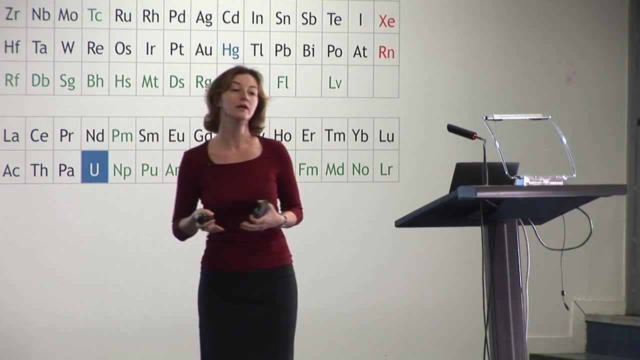 So I mentioned that there is one experiment, that's the Dama Libra experiment. So this is the Dama Libra experiment in Gran Sasso that actually has seen annual modulation. Where it comes from, it's, of course, another story. 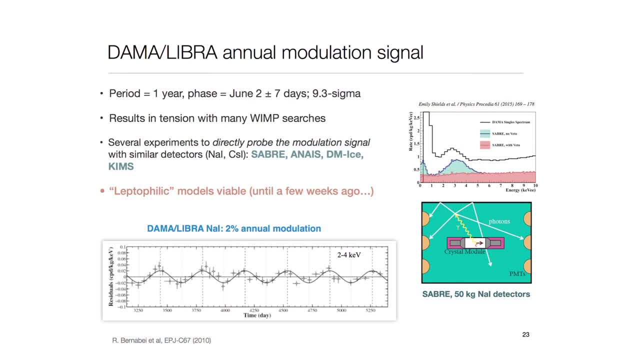 But this is their data over many years now, I think eight or nine years. So the statistical significance that they see such modulation is very high. It also has a correct period and phase. However, if you interpret it as due to WIMP dark matter, 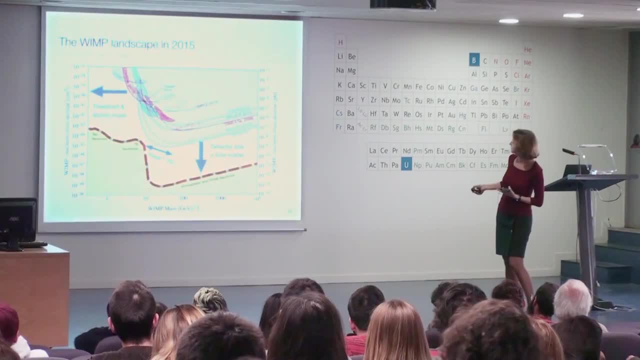 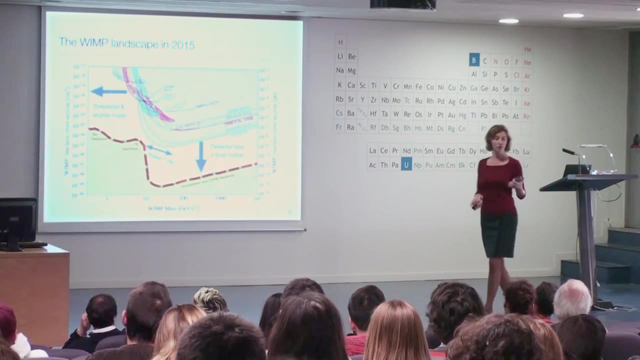 it's quite in conflict with a lot of other experiments. So these would be these Dama regions, And there are now many. They're not even all here. There are many other experiments that do not see a signal. should the cross-section and mass be as predicted by this Dama? 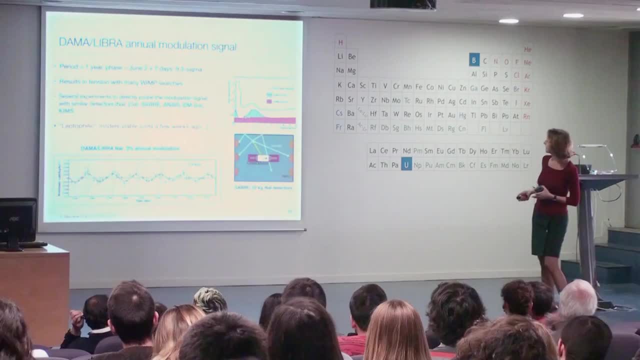 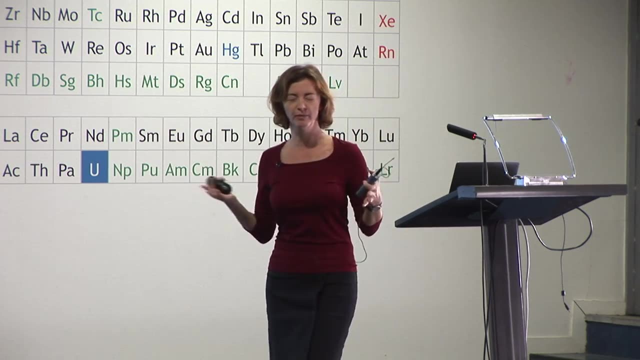 on the one hand. On the other hand, there are still quite a few projects that are building detectors that are made of the same type of material. So really, sodium iodide detectors. these are crystals that are seen by photomultipliers. 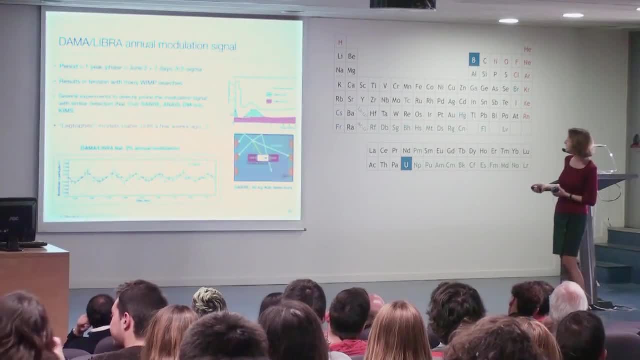 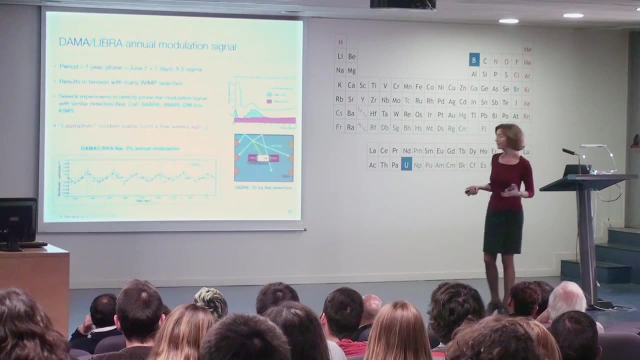 where you just measure the scintillation light. So there is Sabre. there is here in Spain, Anais DMIs KIMS. Just an example: Sabre, they are planning to use this type of crystals in a liquid scintillator. 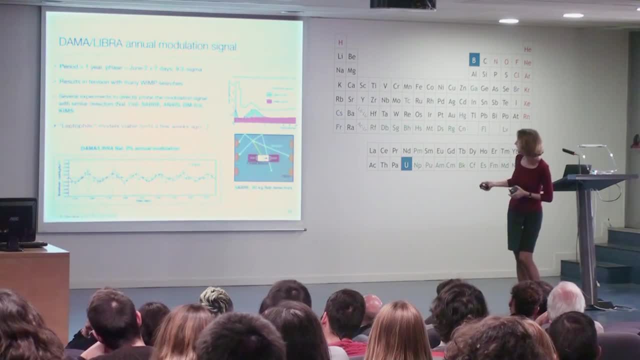 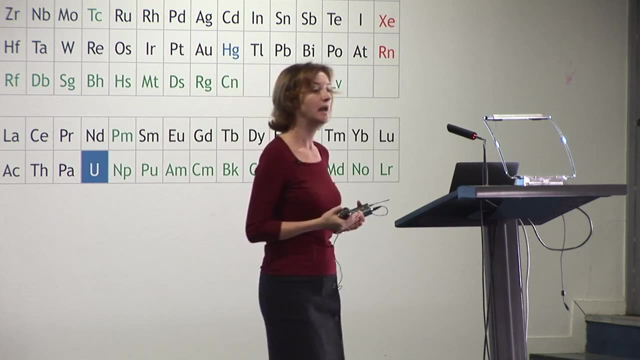 This is a Princeton-based experiment, And here they would like to tag: Well, OK, so they have crystals that support, or they will have crystals that have a lower background than the Dama ones, And also by tagging events that are in coincidence with an event. 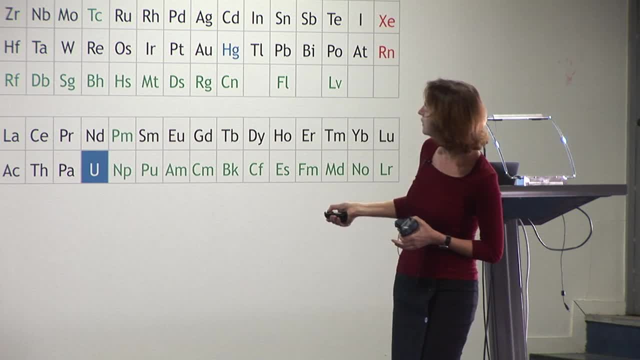 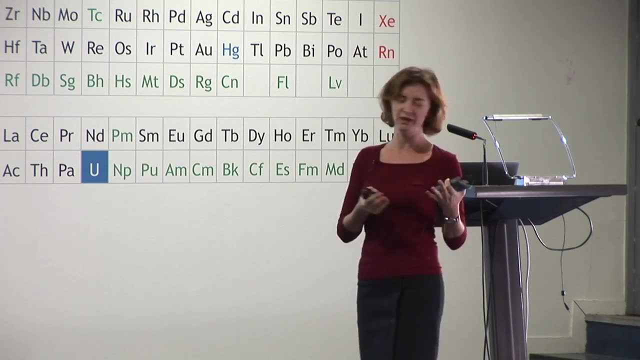 in the scintillator around this crystal, they might get to this very low background. So this would be here, the Dama signal that there is this bump there, a 3kV that could be due to potassium, for instance. 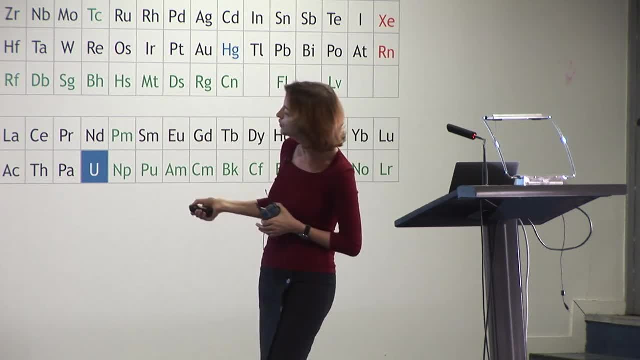 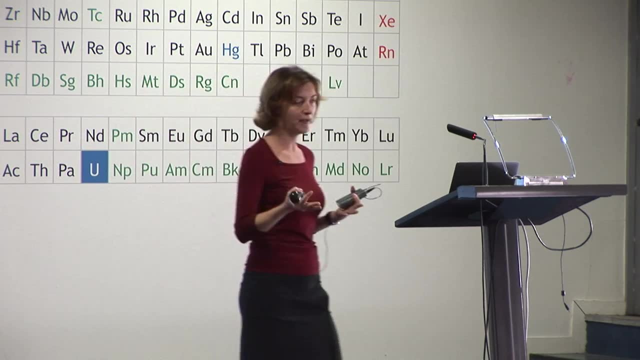 It's not clear, But in any case, they would like to probe that, as also the other experiments. Now there's also something else, So there are a lot of papers making the case. well, maybe what Dama sees is not nuclear recalls. 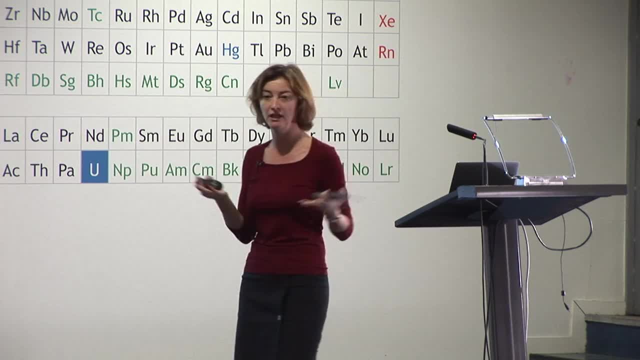 but actually some electronic recalls, because they have no discrimination whatsoever in their detection. They have no position, resolution or discrimination. So they're really a very simple type of detectors And these are so-called leptophilic models, where you have some dark matter that has some interaction. 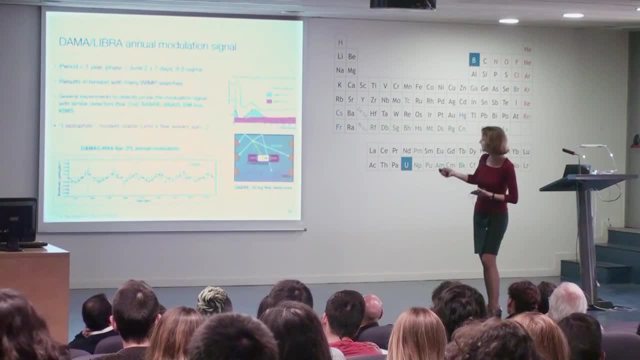 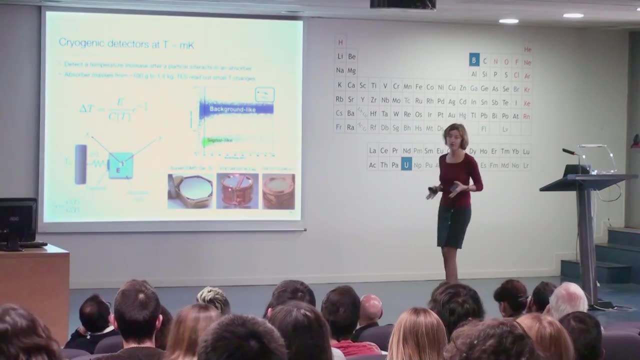 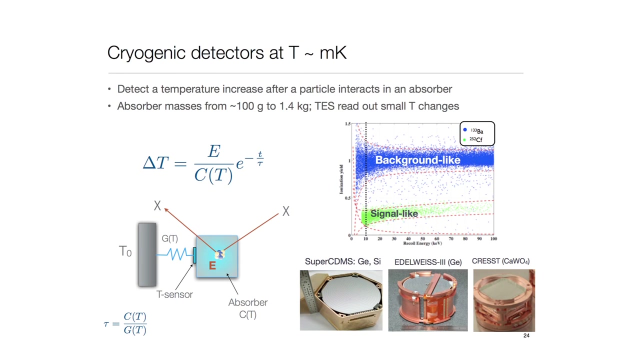 with electrons And these were viable, but recently- I will show you- have actually been excluded. But I will come to that Now. I mentioned that this low mass region will be tested by so-called phonon-based detectors, And they operate at temperatures of about a few tens. 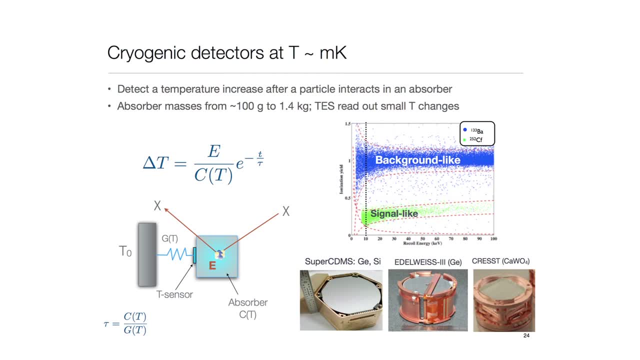 of millikelvin, And they would like to detect a temperature rise after a particle interacts in an absorber, typically a crystal that is connected here to a bath. You have the thermal link, And then the question is, of course, how do you measure very small temperature rises? 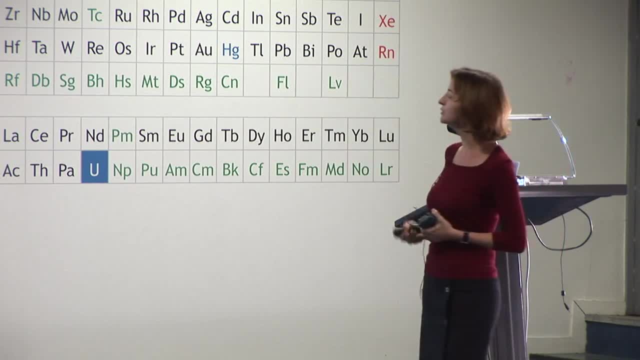 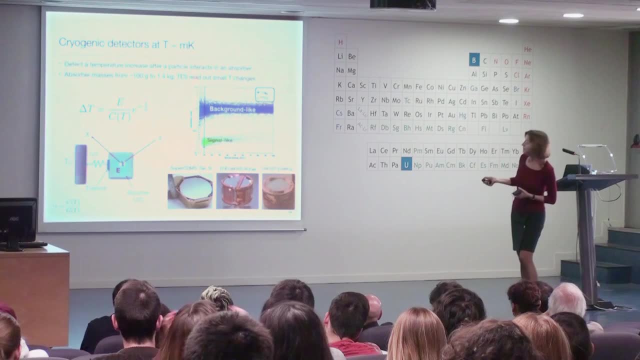 of the order of a few microkelvin or so, And there you use, for instance, transition edge sensors, just like in the CDMS, or also CREST experiment. And here again, if you look at the so-called ionization yield, 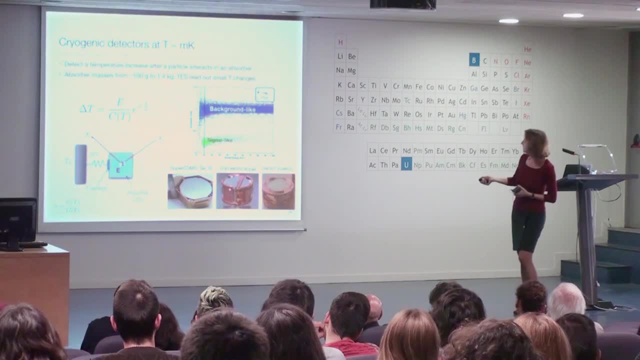 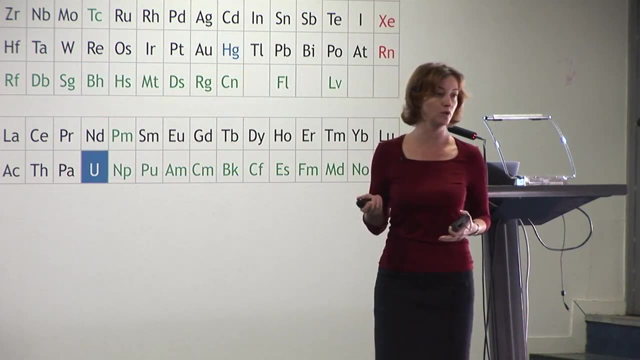 which is the ratio of charge, And you can see that the ionization yield is very similar to the charge to the phonon signal. You have here background-like events that are electronic recalls and a very nice separation with signal-like events that come from nuclear recalls. 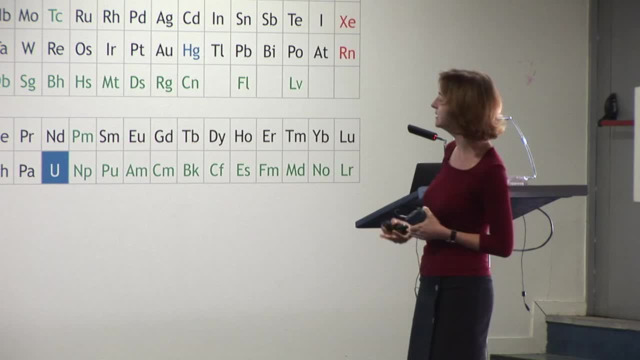 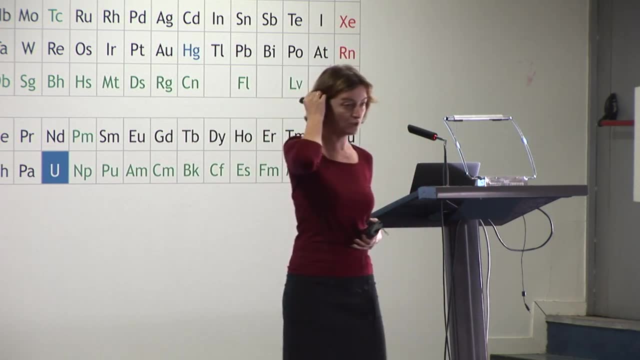 And you calibrate this with strong gamma sources here or with neutron sources, And this is done by all the experiments in the field. So we have the super CDMS experiment that has been approved to go to a larger phase at SNOLAB in the US. 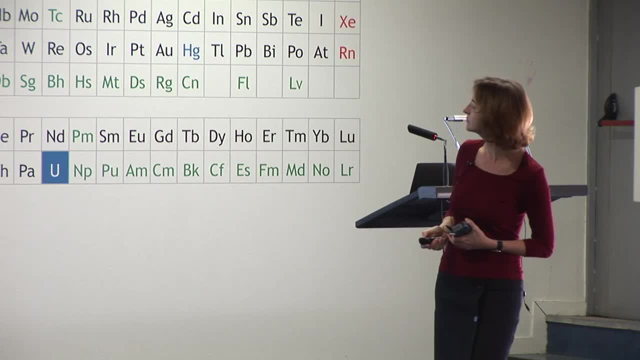 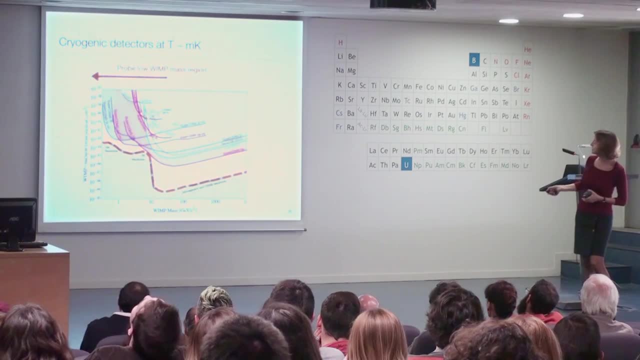 And in Europe we have Edelweiss in France and CREST, that is in Gran Sasso. So, as I mentioned already, these are just some predictions. They are now around here And these are the predictions where, for instance, 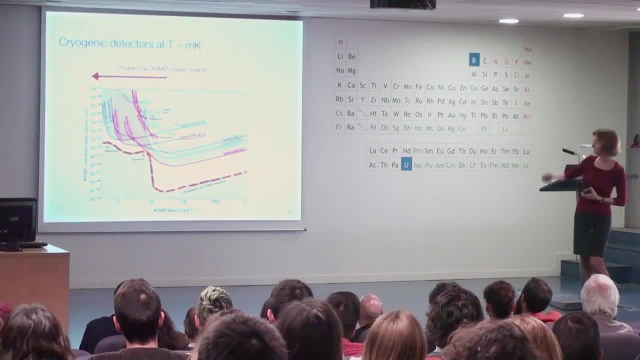 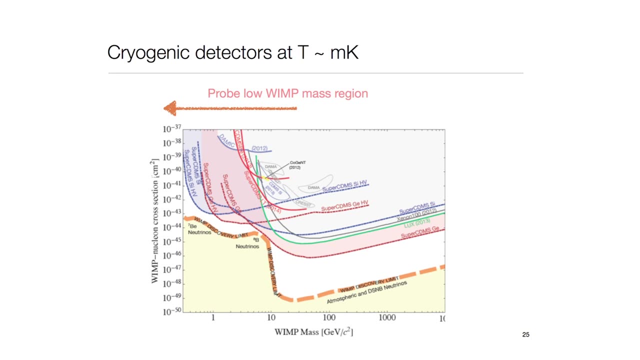 super CDMS might go in the future with these neurons at SNOLAB And they will test, of course, also here, part of this high mass region. I'm not showing the slide, but I would also like to mention that there is also a proposal. 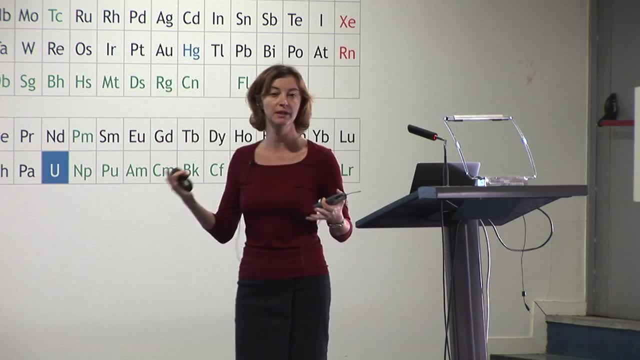 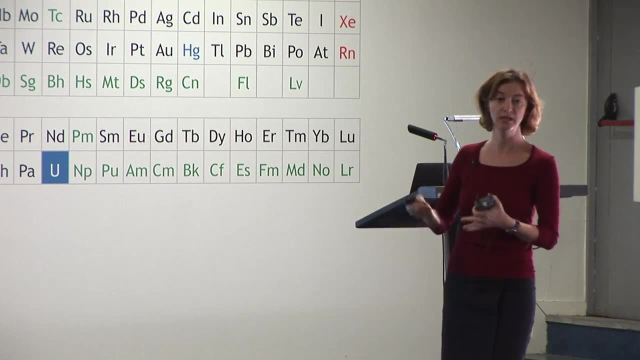 Well, there are the plans that they might join forces and build a much larger detector at SNOLAB. So there's a European Eureka project that is Edelweiss and CREST. So together with super CDMS they might go to 100 kilogram. 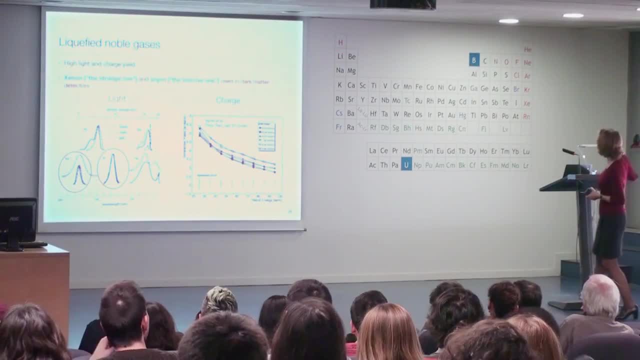 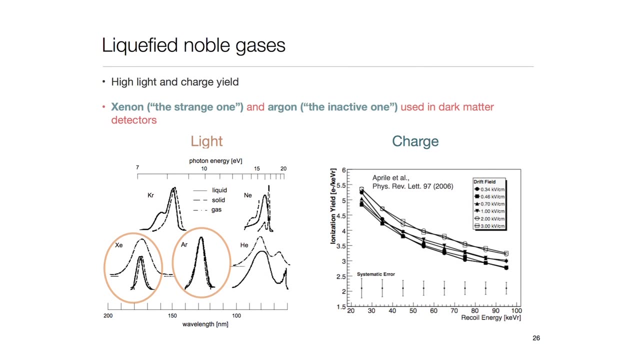 or so detector, So noble gases. so we come to this part here of the periodic table that we nicely have on the wall, And we will mostly deal here with xenon and with argon, even though radon and krypton are real troublemakers. 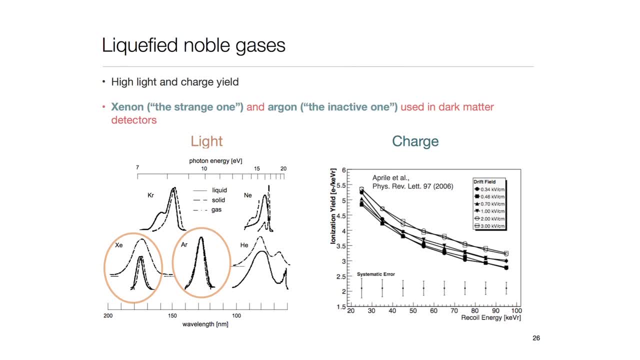 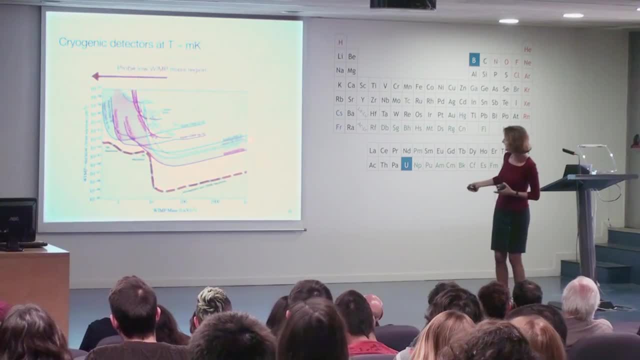 because they give us a lot of background that we don't want in the end. So Why are these materials? Maybe, before I go there, I should have mentioned that actually today, the best results, the best limits here come from xenon-based experiments. 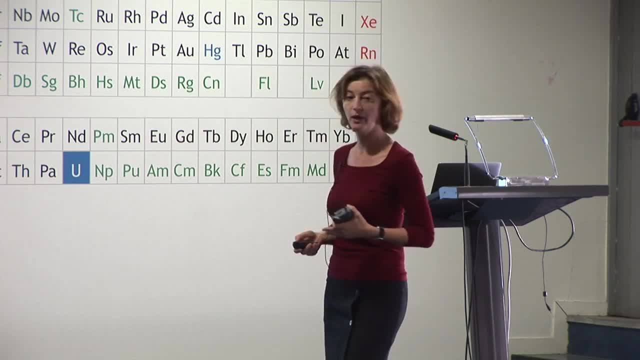 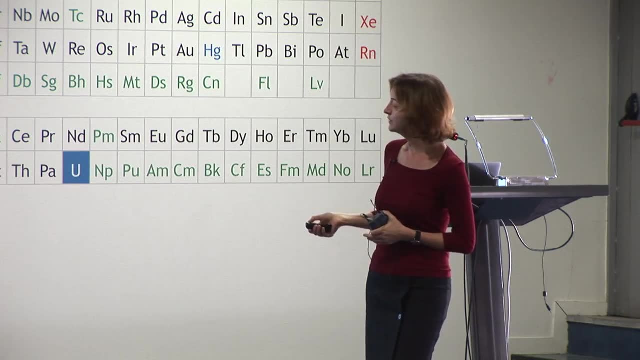 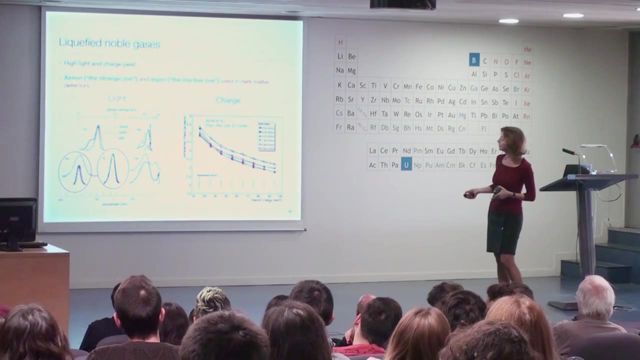 so experiments based on noble liquids, And this is why noble liquids are now in principle very interesting for dark matter detectors. So they have a very high light yield And they also have a high charge yield. You see here the light xenon argon. it's in the VUV. 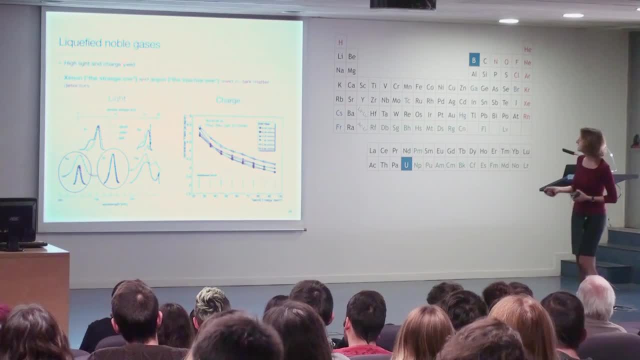 unfortunately, That's quite difficult to measure, And xenon also means a strange one, while argon is the inactive one. So these two are used in dark matter detectors And what we detect is, on the one hand, the scintillation. 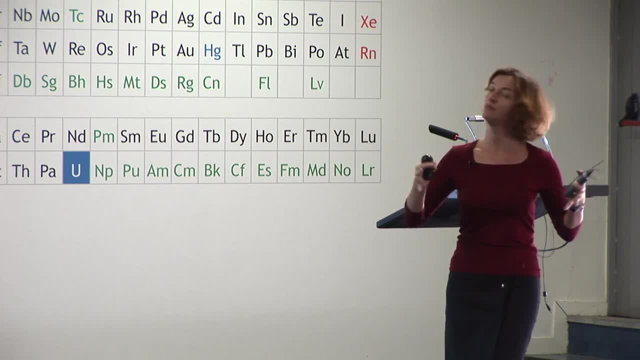 light after a particle scatters in a liquid- well, in a noble liquid detector. But on the other hand, as I will show you also the few free electrons that are produced in a collision. And there are two philosophies here. On the one hand, 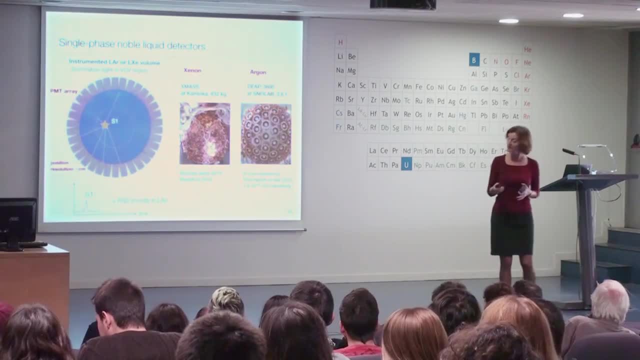 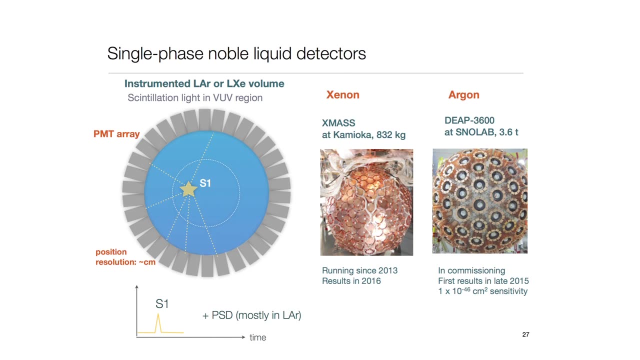 On the one hand, the so-called single-phase detector. Single-phase means you just have a large amount of liquid, let's say like xenon or argon, that you instrument all around it with photo detectors, photo sensors, And then you look at this very prompt, fast scintillation. 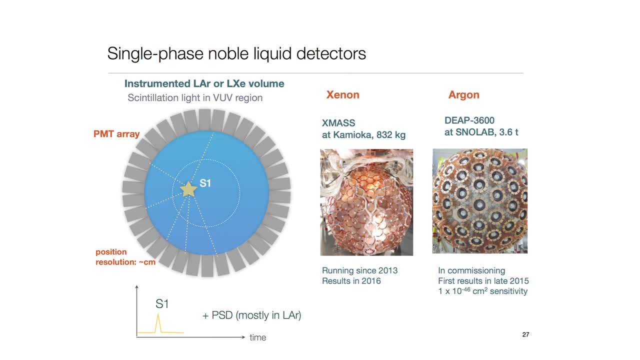 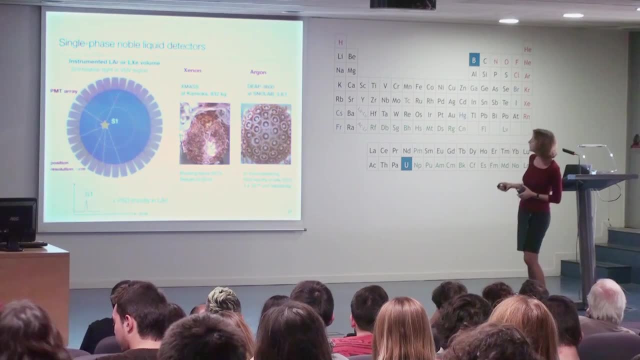 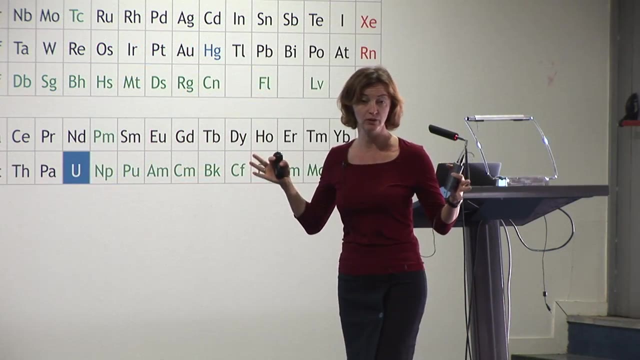 light that is being produced when a particle scatters here in your fiducial volume. And the two examples that are here are the XMAS detector, a xenon-based detector, in Japan in the Kamioka mine. They have about 800 kilograms of liquid xenon in total. 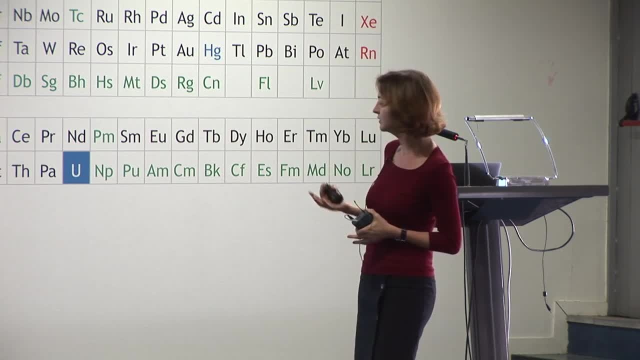 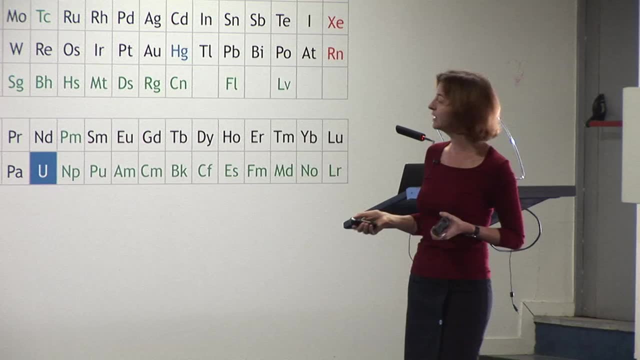 They have to fiducialize And they will use just the innermost 100 kilogram detectors. They had some issues with backgrounds And they have totally refurbished their detector And they are running again. The problem with background is here. For instance, they had some background in their PMTs. 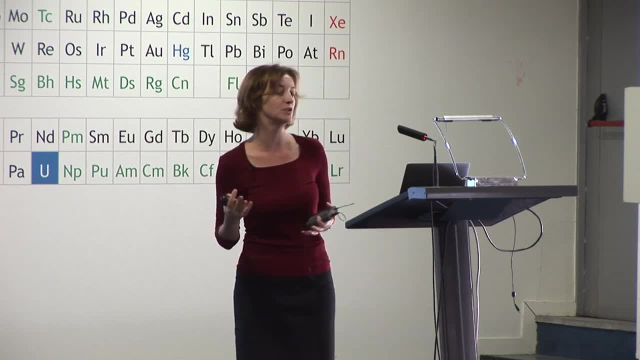 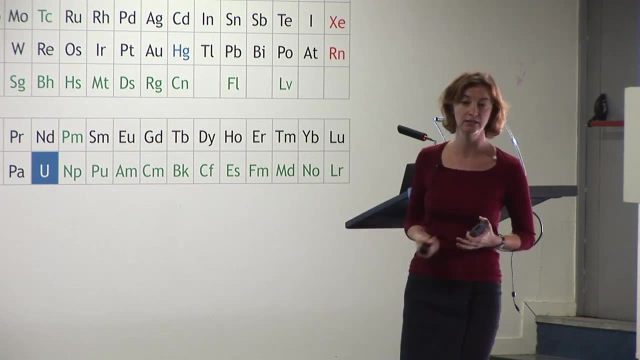 But because in the single-phase detectors their position resolution is actually not very good, then you can reconstruct events that are here at the edges And you can see that this is not really what you want. And then for argon, there's the DEEP 3600 experiment. 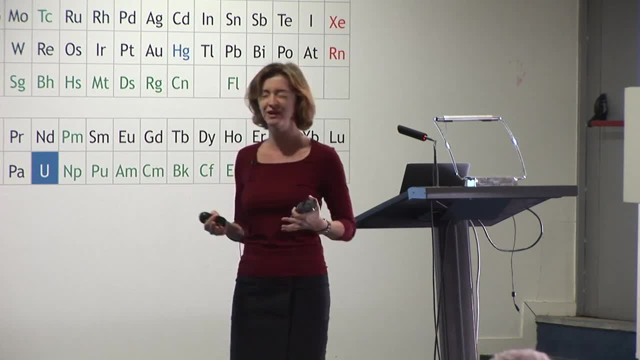 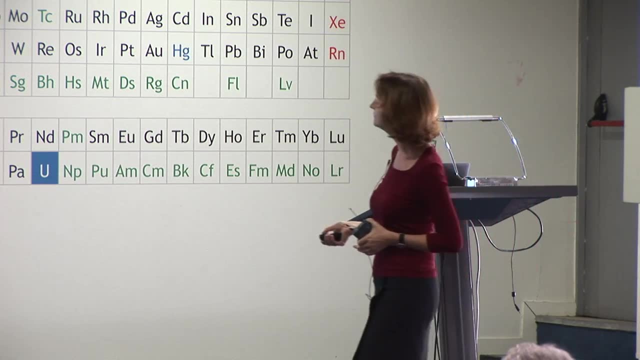 It's no lab. So we are all looking at DEEP because they are in commissioning And first result: so it's the largest argon detector now that's available. First results hopefully will be, well, I guess, late 2015.. 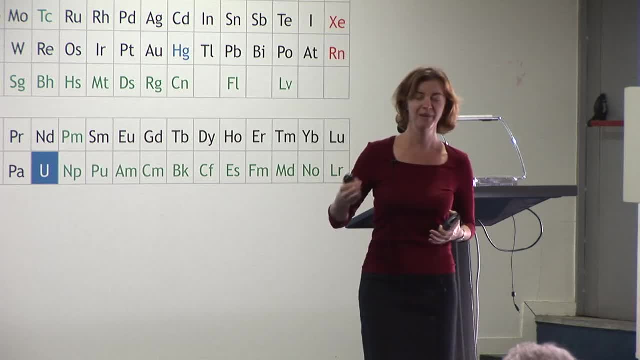 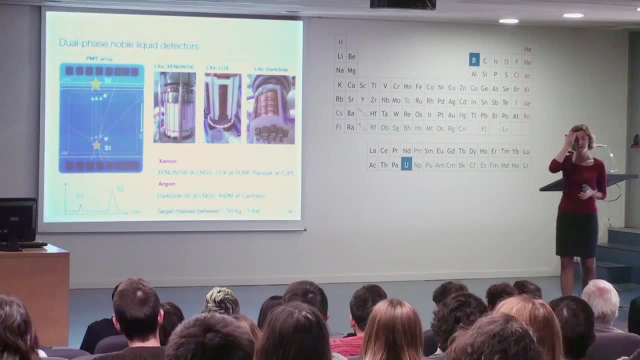 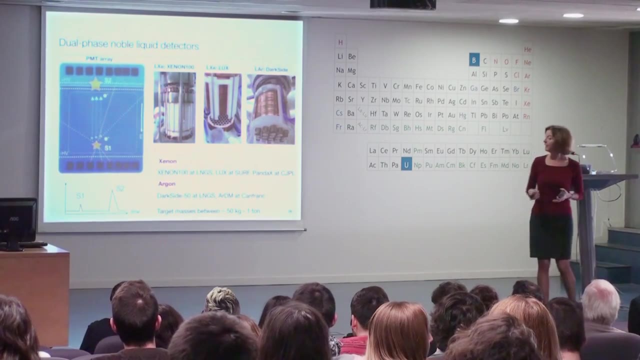 That's not really true. By now it will be 2016 or so. And then the so-called XMAS detector. So this is the XMAS detector- It's called dual-phase noble-liquid detectors- where you actually build a TPC time projection chamber. 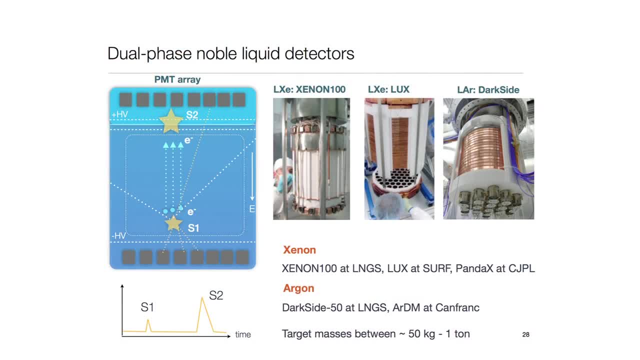 And what happens here is, again, you have a large amount of liquid, But on top you have the vapor phase that's in equilibrium with the liquid. So you have on the one hand, the prompt scintillation light signal that is observed by mostly the ray that's. 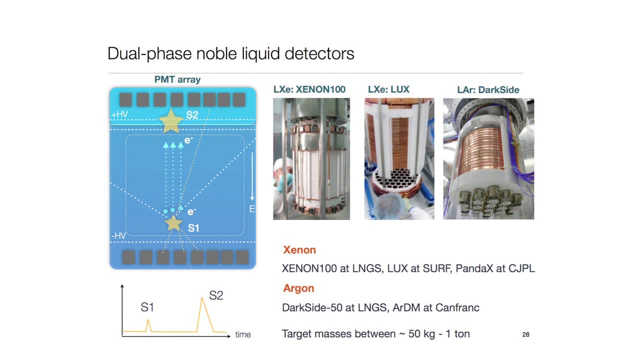 immersed in the liquid, but also by a top array, And then you have a few electrons that are liberated in the process And you apply a strong drift field, typically about 1 kilovolt per centimeter, then a much higher extraction. 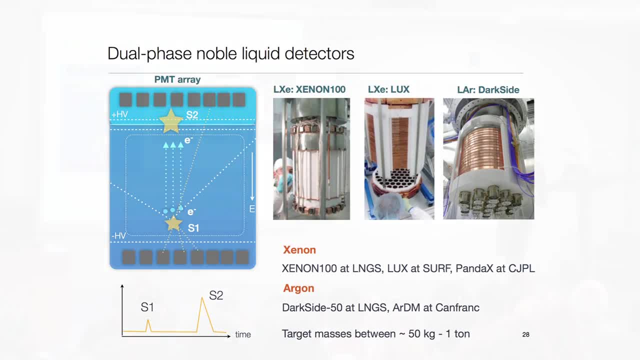 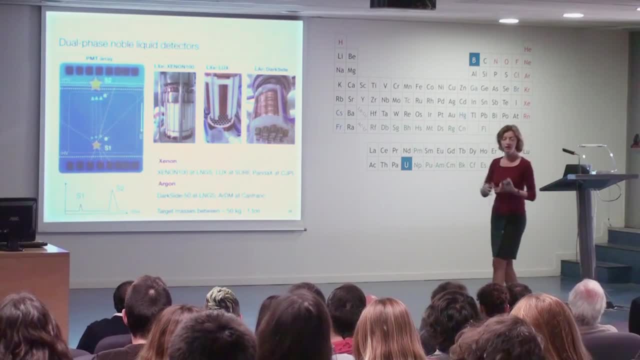 field, typically 10 kilovolts per centimeter or so, to extract them in the gas phase, where they again will collide with atoms and produce what we call proportional scintillation signals, So a larger scintillation light signal. 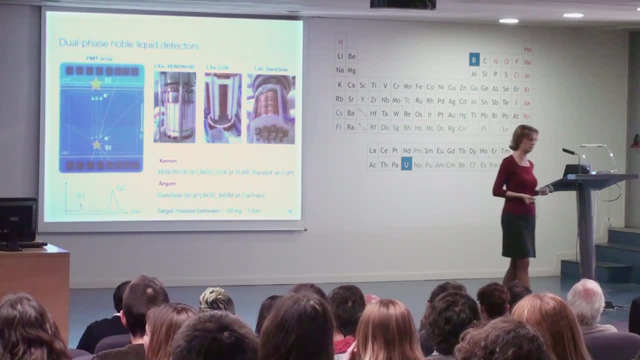 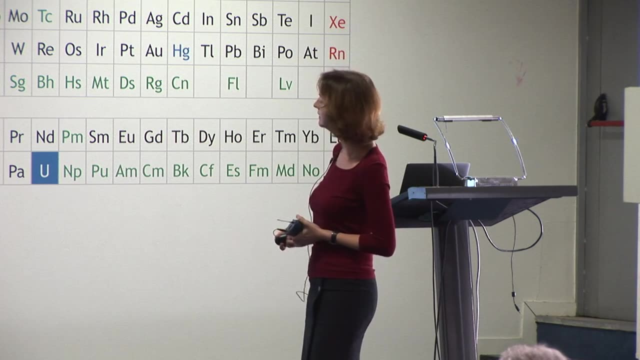 that is proportional to the actual energy deposited in the detector, And the ratio of the two will tell you whether you deal mostly with the signal light or a background-like event. But most importantly, the time difference gives you quite precisely, with some millimeter precision. 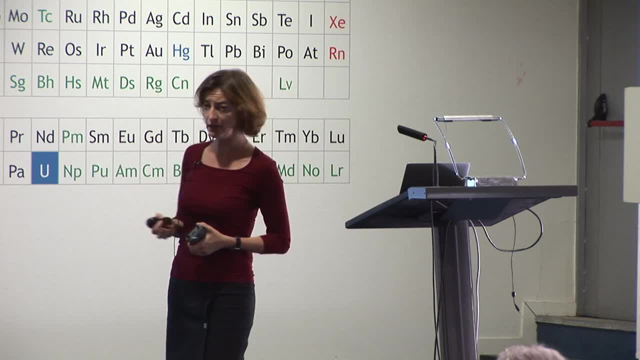 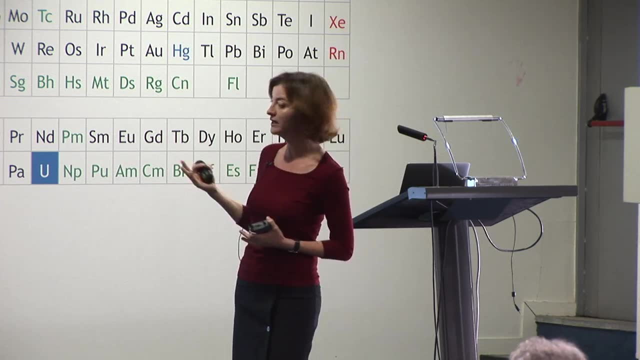 the z-position of your interaction And the distribution of the light in the top photosensor ray, because this light here- the S2 light as we call it, is very localized- will give you the xy-position, So you have a very good 3D position reconstruction. 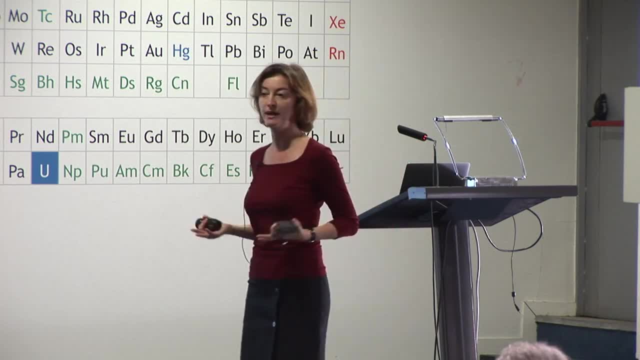 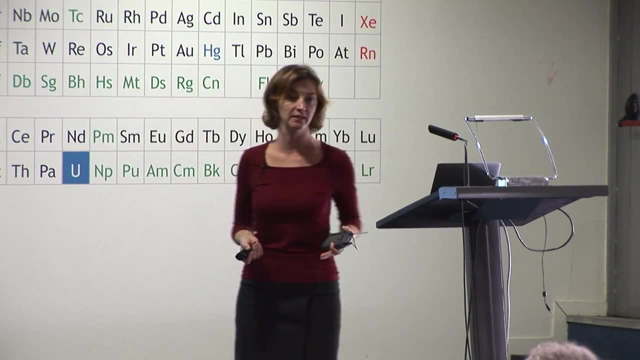 of where the event happens And that helps you to reject a lot of the background. Also, a lot of neutrons, Because neutrons, as we know, are strongly interacting particles and they tend to multiple scatter. So we have the Xenon-Hunder detector still operating. 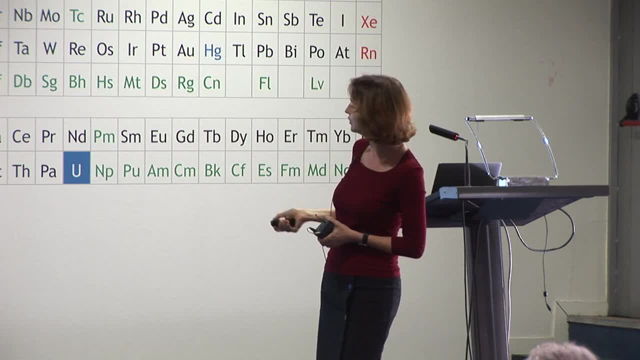 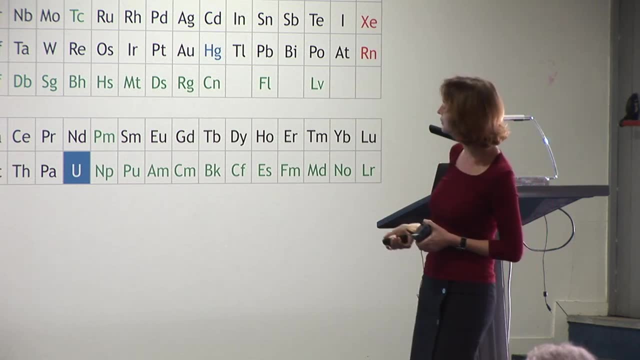 in Gran Sasso, mostly now doing calibration measurements for one ton, The LUX experiment in the US that has now the best limit for WIMS, as I've shown you, And also in Gran Sasso, a liquid argon-based experiment. 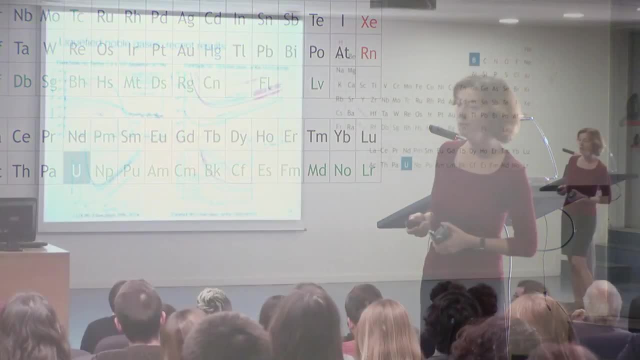 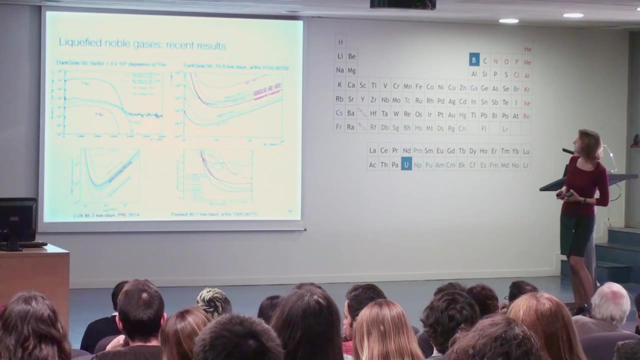 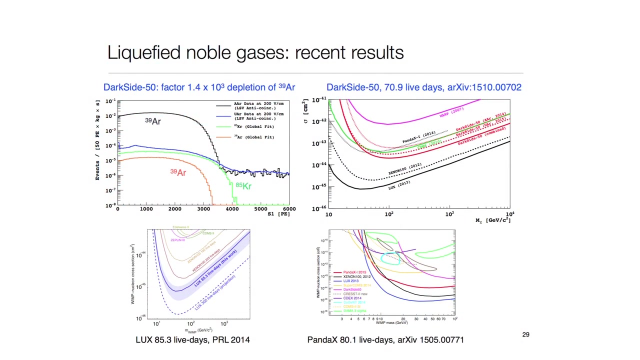 namely the dark side detector, And I won't go into the details of these detectors, maybe I'll just show you some very well recent results. So dark side 50, they just, I think in October they published a limit. 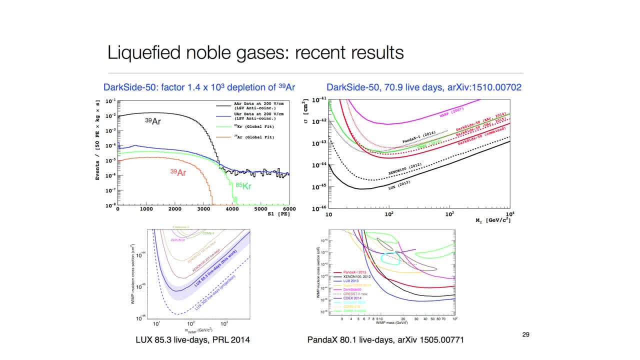 They're not really competitive with LUX or Xenon-Hunder, so they're here. on the one hand Also, it's a much smaller detector, But on the other hand, what I've shown is that they could reach a depletion of about a factor. 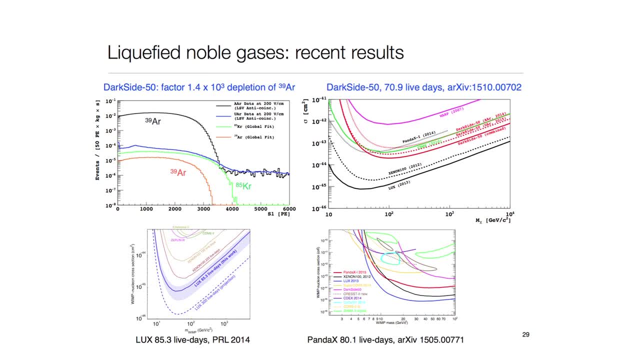 of 1,000 in this argon-39.. So in argon you have a problem of the cosmogenically produced argon-39. That comes from the atmosphere And that gives you a lot of beta decays in your detector. 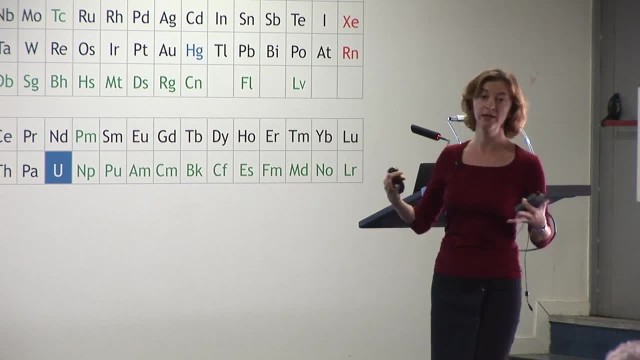 So you need argon Here. they take it from underground sources. that is depleted to 1,000, but maybe even more. There's also another detector, but it's in China. It's called Panda-X. It's also a dual-phase liquid Xenon. 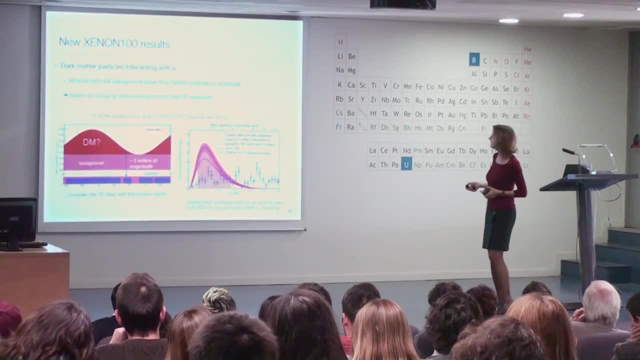 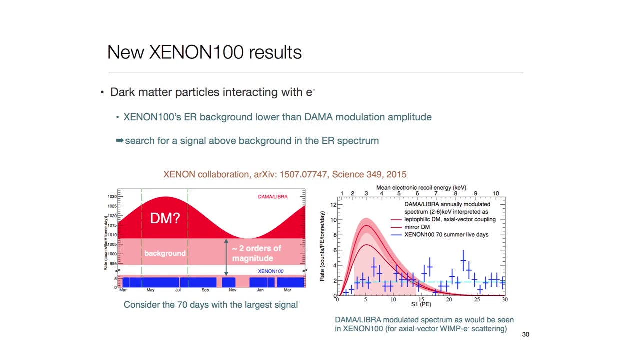 detector. Now there was a new result, recent new result from Xenon-100.. I mention it here Because we actually looked at so-called dyslactophilic models, where we just assume that you have a dark matter particle that interacts with electrons. 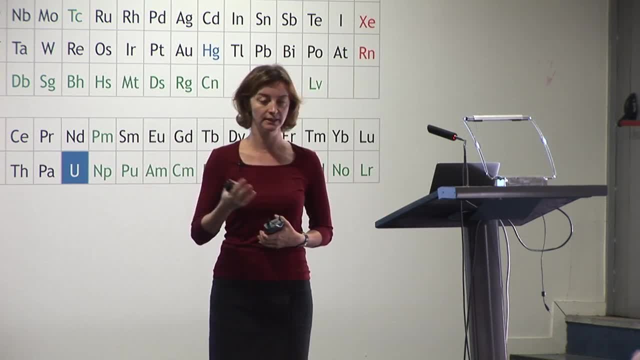 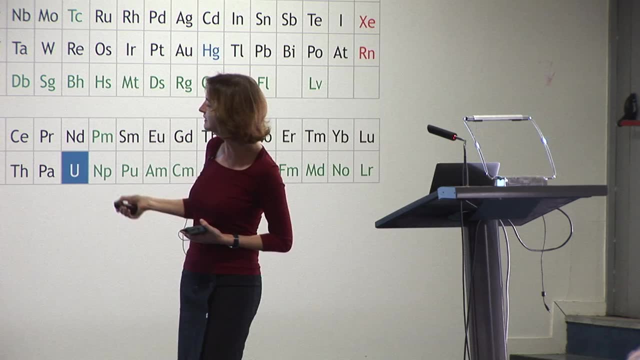 And you try to see whether you actually could see the signal by DAMA, Because Xenon-100 also has a very low energy threshold But, most importantly, it has a background that is more than 100 times lower than the background in DAMA, without any discrimination. 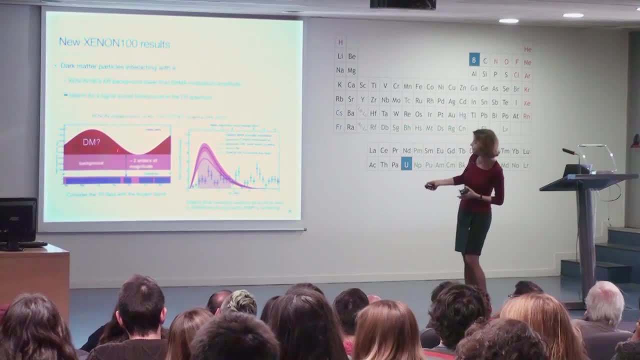 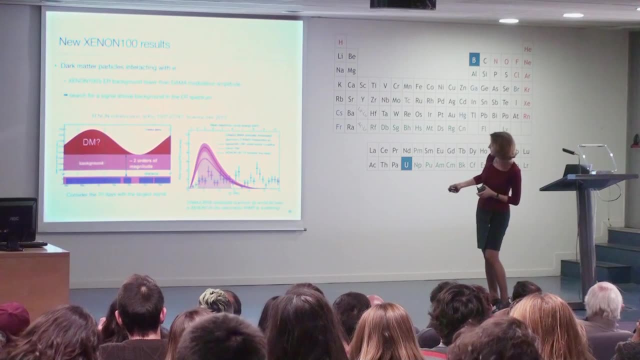 So this is the Xenon-100 background, This is DAMA's background And that may be a signal. So this is just to explain to you very briefly the principle of this And this is now the integrated background here over a certain amount of time. 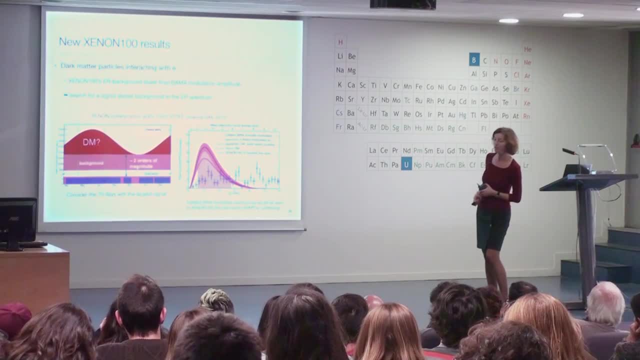 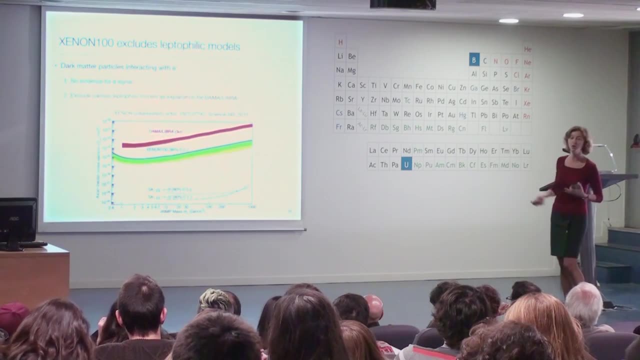 And this is what you would expect from DAMA in these various lactophilic models. And obviously we do not see that And this is why this DAMA region in these models can be excluded. Again, I'm not going to go into details. 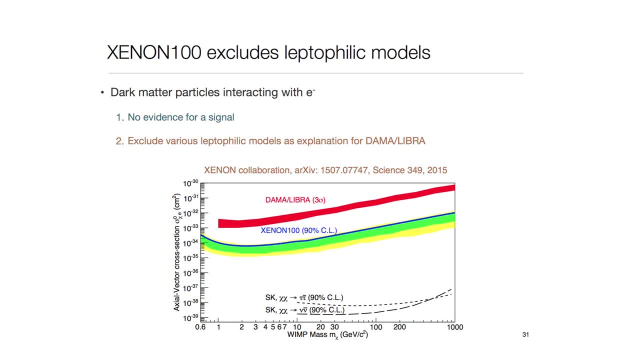 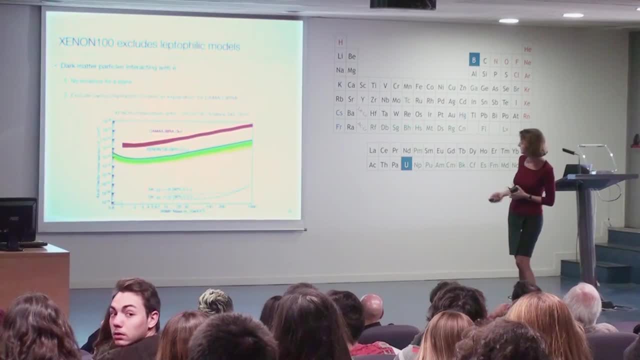 There's another paper where we looked at the annual variation of the event rate, And again there's no measured annual variation, And that also excludes DAMA. That's a PRL that also appeared, But OK, So what is now the future for these noble liquid detectors? Well under construction, I should say under commissioning now is Xenon-100. And the next phase will be N-ton in Gran Sasso. There's also a proposed and approved project in the US. That's the biggest competitor, of course: the LZ, the Lax-Zeppelin experiment. 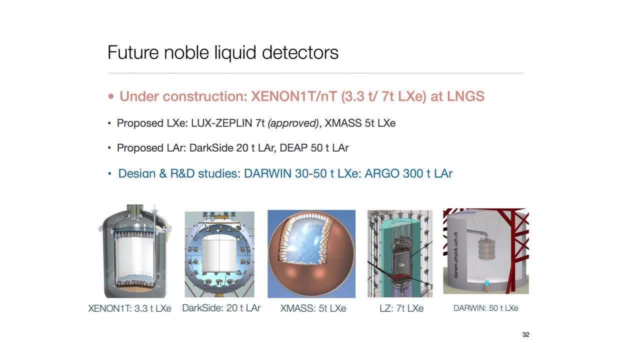 That will also use seven tons of liquid Xenon. And this is the first phase, And this is the second phase, And this is the third phase, This is the third phase, And this is the fourth phase, And this is the fourth phase. 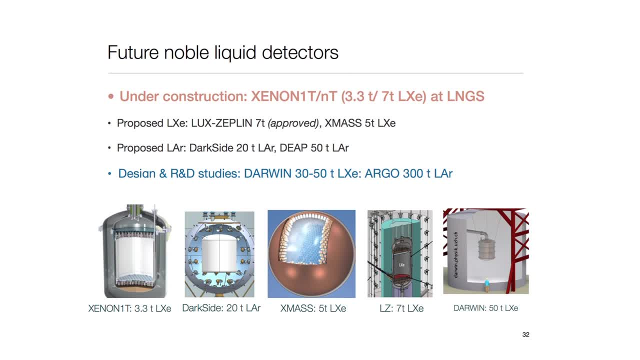 And this is the fifth phase, And this is the sixth phase, And this is the seventh phase, And this is the seventh phase, And this is the sixth phase, And this is the seventh phase, And this is the eighth phase. So there's a proposed and approved project in the US. 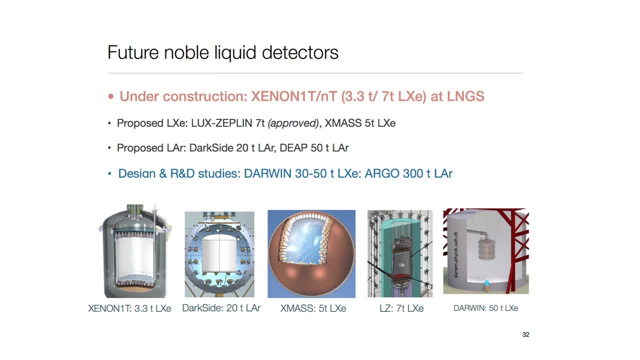 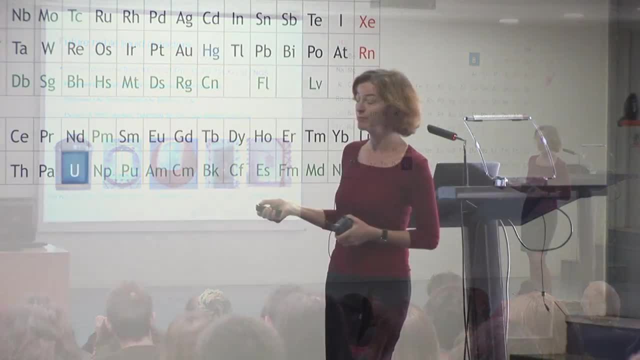 That's the biggest competitor, of course, the LZ, the Lax-Zeppelin experiment, And that will also use seven tons of liquid Xenon. And also there's a proposal for five-ton experiment in Japan. For Argon, there's a proposal of a 20-ton detector in Gran Sasso and a 50-ton deep. 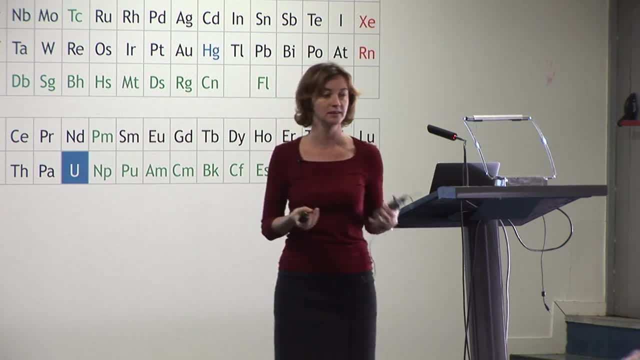 detector at Snow Lab. And finally, there are also some R&D and design studies. We are involved in this Darwin Design study that would operate a 30 to 50-ton liquid Gran Xenon detector for dark matter, but also for other types of physics. 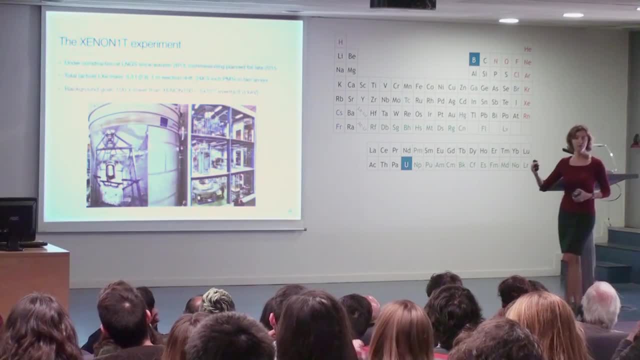 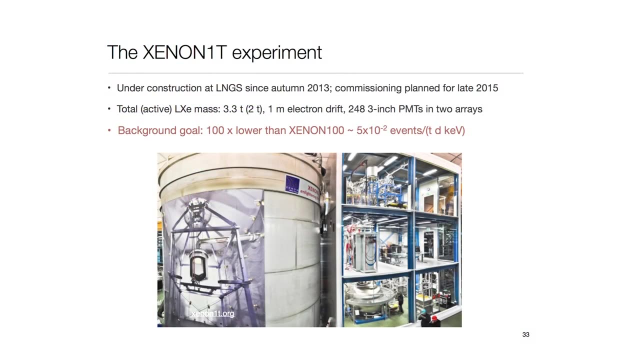 So I'm showing you now some slides on Xenon OneTone, because we just finished installing it in Gran Sasso. we are now commissioning the detector. we started in autumn of 2013 and you can see here this is from outside the water shield. inside now this is a picture. 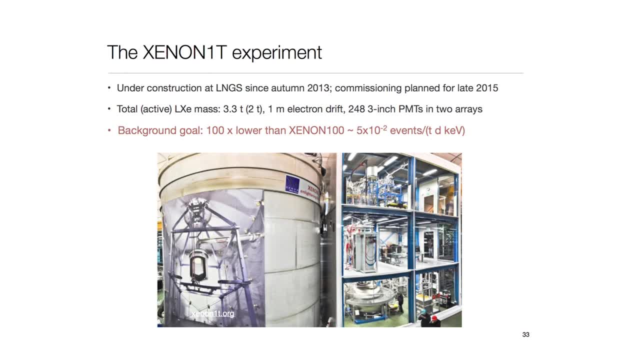 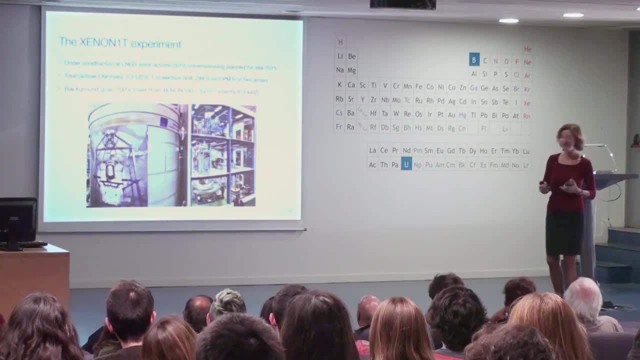 because you can't really see inside, but I will show you. you know, this is just a large water tank, but inside is a Cherenkov shield and then there's a structure that holds the cryostat and then inside the cryostat is now the TPC. but this is the service building and 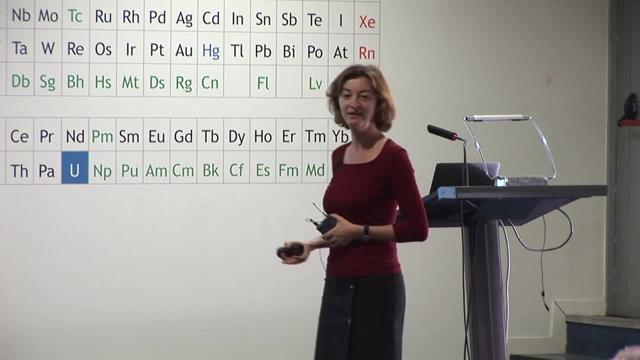 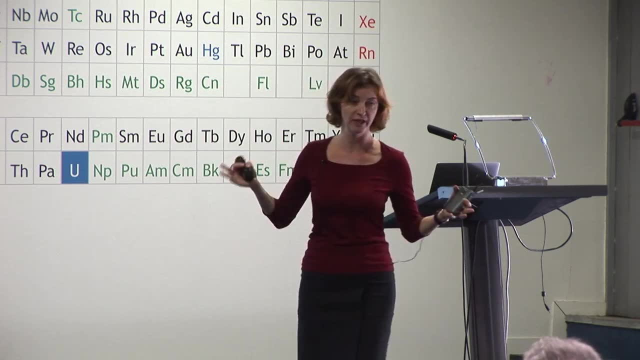 I hope you appreciate it. actually we just had the inauguration mid-November and a lot of people really liked it that it's not closed so you can actually see everything. So we have here the Xenon storage system that is called Restox that can store 7.6 tons of. 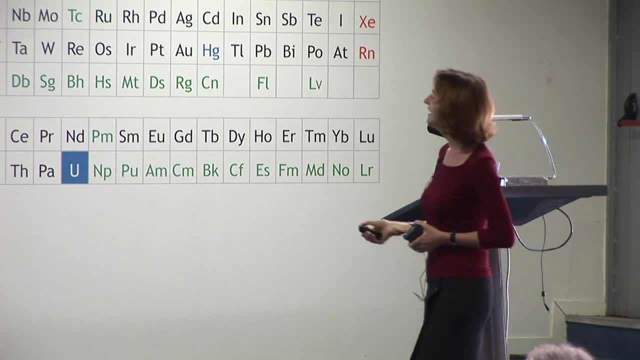 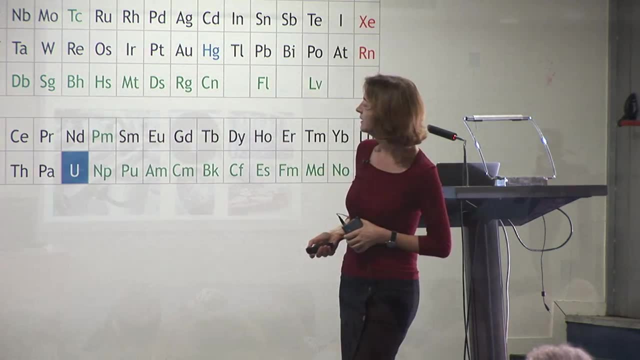 a factor of 100 lower. Then the first phase, that was xenon 10, and in terms of physics I will show you 10 to the minus 47 or so cross section. So here you can see some pictures from inside. this is a cryostat. this is quite important. 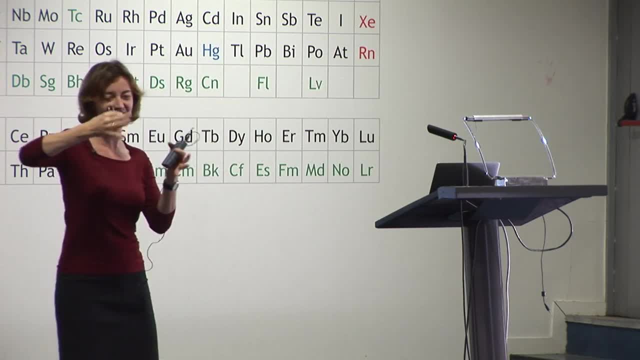 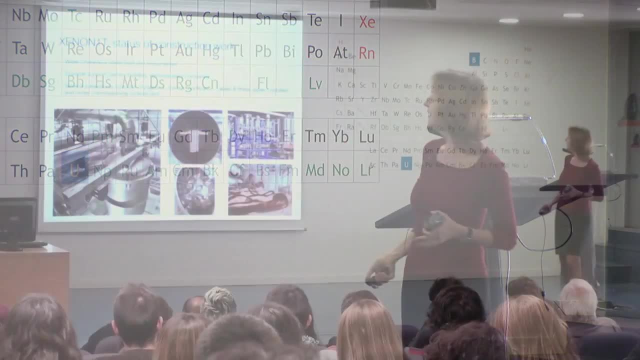 it's a very long pipe. we call it the umbilical pipe. that connects the inner part of the detector with that building. that has all the cryogenic pipes in it but also the pipes for the signal, for the cables here we were preparing, actually the cables in Zurich. this is one of my post-docs. 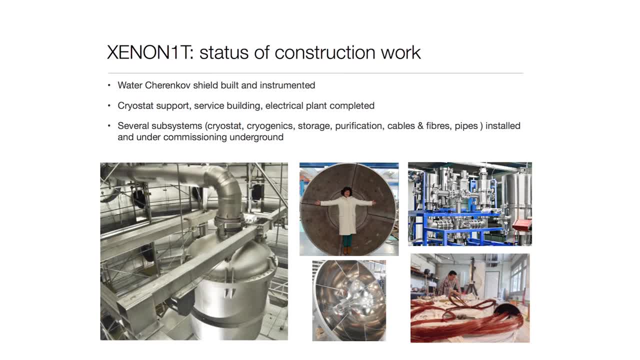 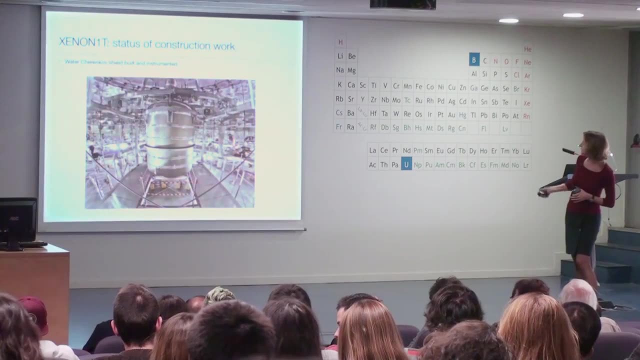 all the signal cables, The high voltage cables and so on. they must be obviously installed in here. well, it's 10 meters, the whole water tank and this is some space to the top, but not much. This is the storage system here. you can see it. so this here is 10 meters tall. 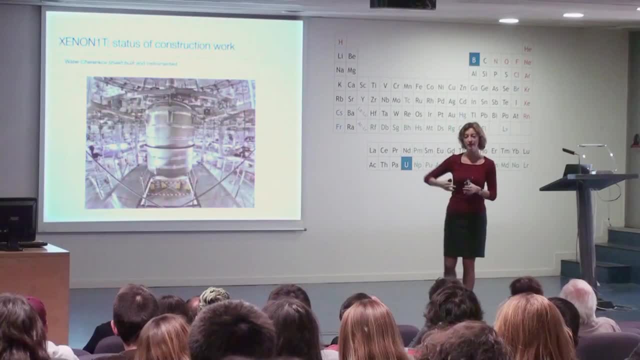 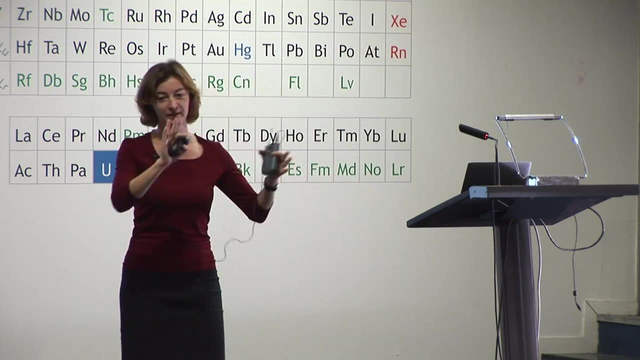 So this is in Hall B. it is next to where Icarus was, so Icarus was on the right of it. now there's nothing there, And on the left of it we have a failed. but maybe I'm not saying anything because okay. 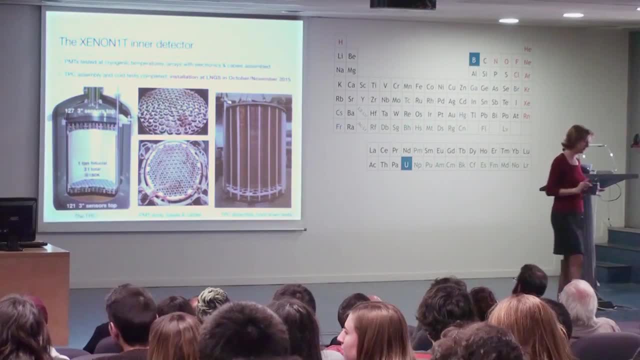 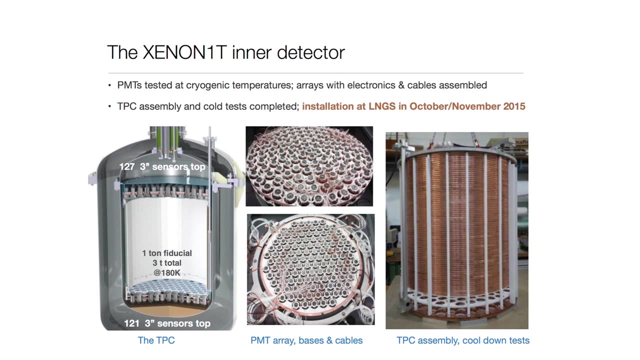 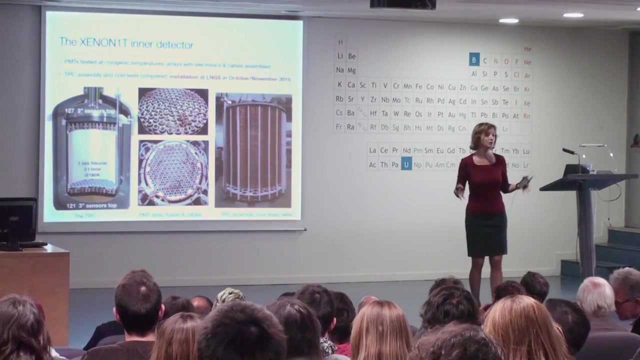 Anyway. so this is the inner detector. where was mostly our responsibility in Zurich? the actual time projection chamber? We have two. you can see here the field cage. we have 74 field shaping rings because you have to have a very uniform drift field for your electrons. you don't want to have any. 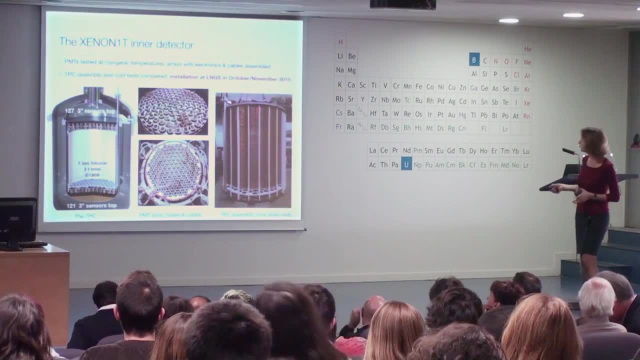 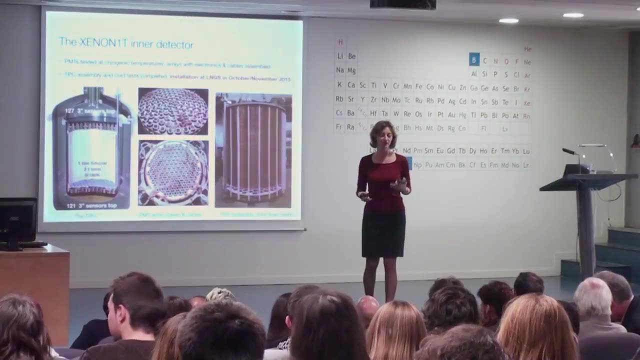 dependence of your signal on the position Then we have. the structure is mostly made out of Teflon. the inner structure, the reflector, because it has a very high reflectivity for the xenon UV light on the one hand. on the other hand, it's radio pure. 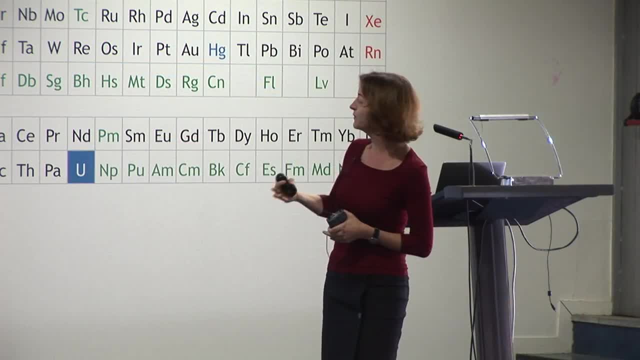 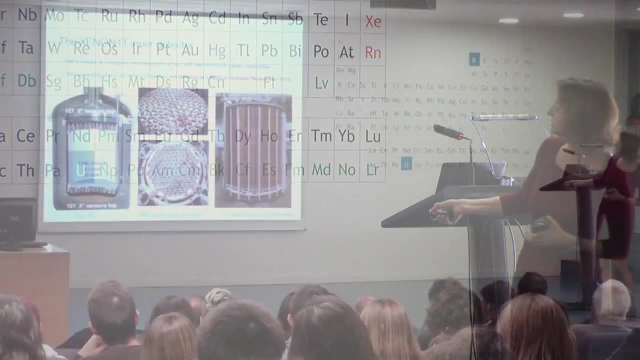 You can see here we also developed the readout for the, so we were also responsible for half of the photo sensors. so we have the three-inch photo detectors with very low radioactivity. This is here their basis, their electronics readout. Well, this is when we were a sensor. 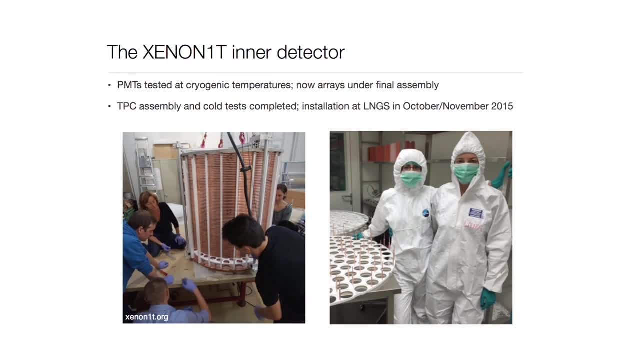 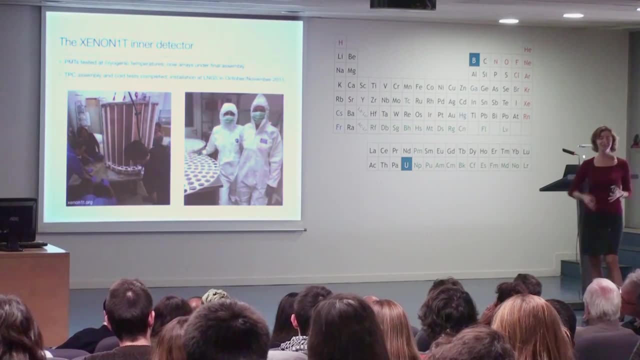 We were assembling and then doing some mechanical cryogenic tests of the TPC in Zurich. You can see here some of my postdocs and students, and here we were assembling the PMT arrays at the Max Planck Institute in Heidelberg. After we assembled everything, we disassembled it, we cleaned and we brought to Gran Sasso. 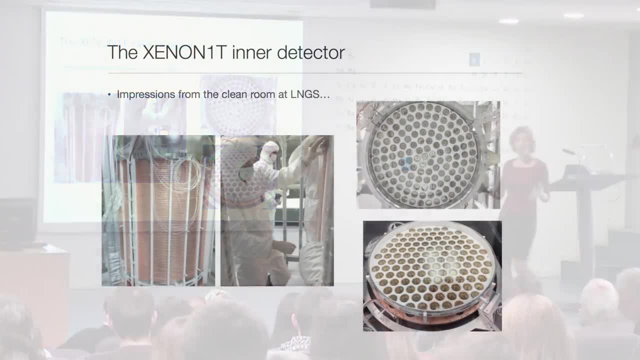 where we assembled all of this in the clean room above ground. and then, finally, the day came when you know these were many, many weeks of work. You can imagine being in the clean room every day until 10 pm or so. 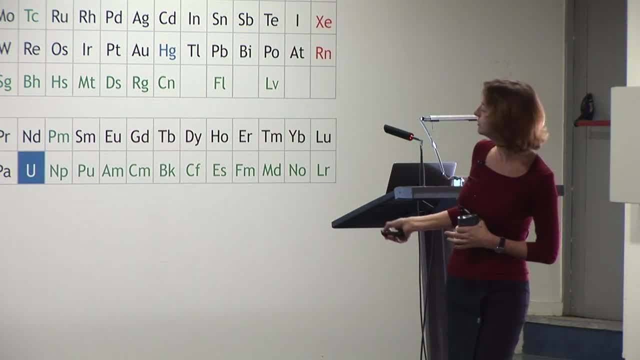 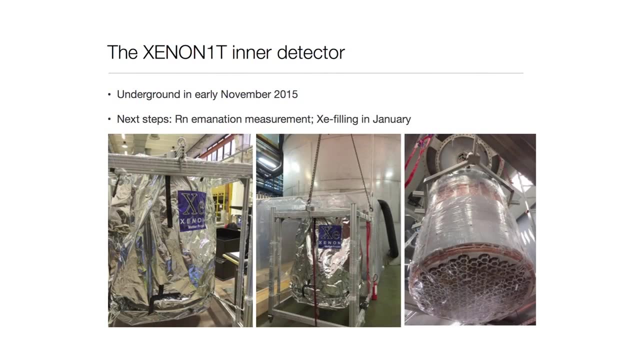 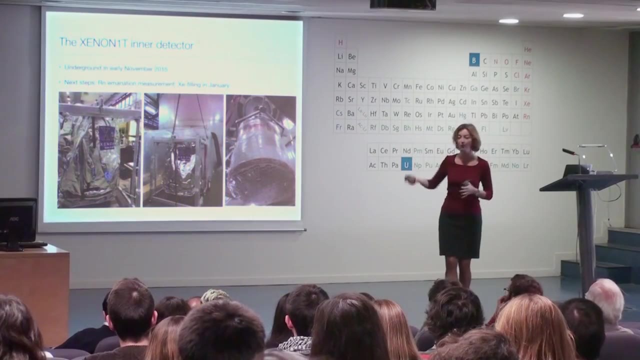 You can see here the nice photo sensor arrays, the bottom array, the top array. and then, finally, the day came when we packed everything, we put it on a truck and we moved underground and then we brought it inside of the water tank. Of course the cryostat had to be open, and then we lifted the TPC. and now it is so that 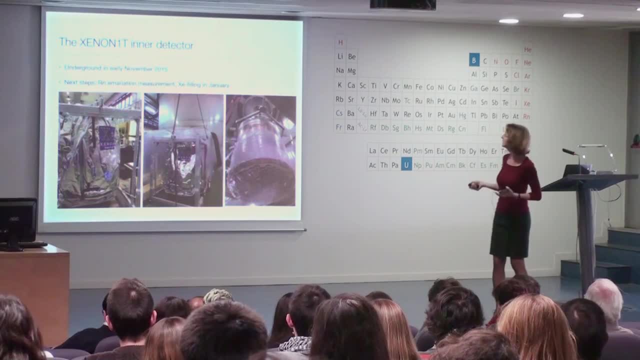 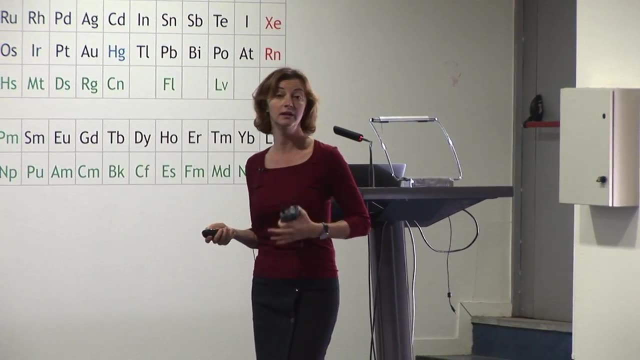 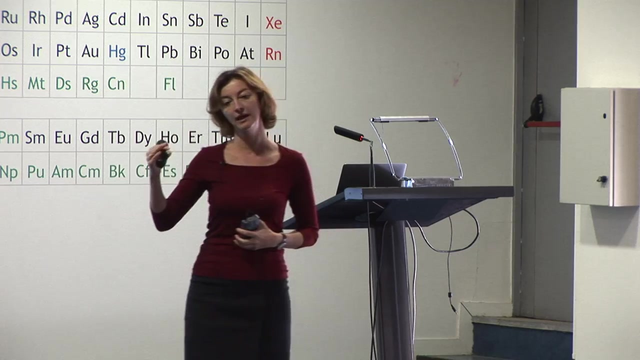 the cryostat will be actually closed within this week. then we first have to do a radiation test. This is the first xenon in the detector, hopefully in early January. So this was the xenon program. Everything is built such that we will have a very fast- hopefully- upgrade to a seven-ton. 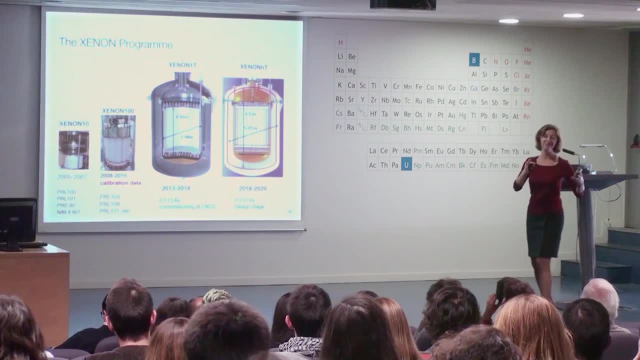 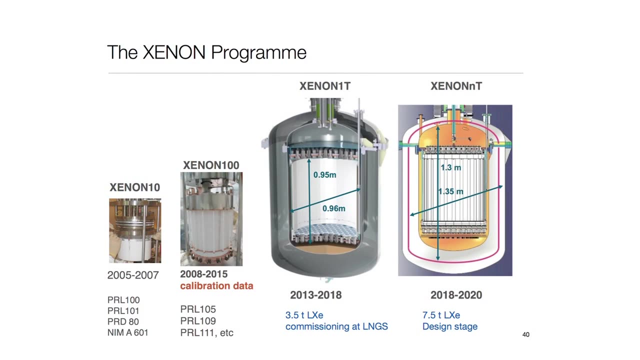 detector. Yeah, we didn't even start the first, the one-ton. so we are talking about, we have to talk about the upgrade already. So, basically, the outer cryostat is large enough, everything is large enough, but obviously we have to build a new inner cryostat and a new TPC. 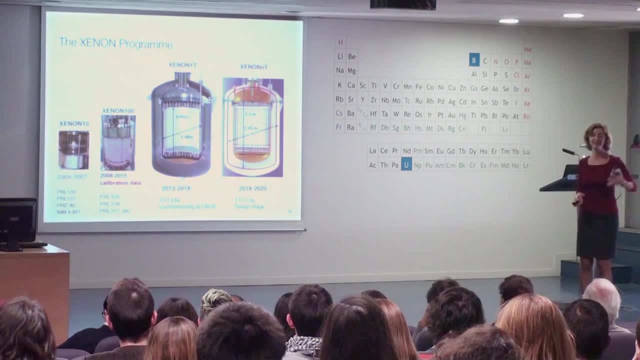 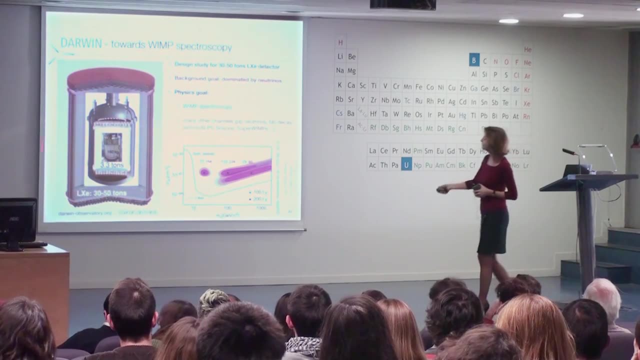 And that is not, is by no means trivial. And we have to get another three tons or more of xenon. And finally we also talk about Darwin. So here we would go to a you know 50-ton detector. Why? Well, because if you see some first signals in one-ton or N-ton or in LZ, you'd like to actually measure this signal with much higher statistics. you'd like to do some WIMP physics, in the sense that you need a certain number of events if you want to determine what is. 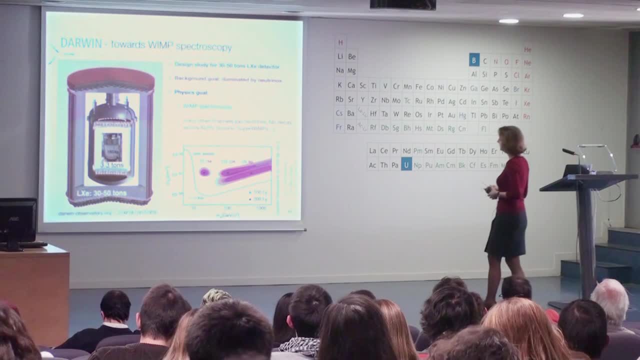 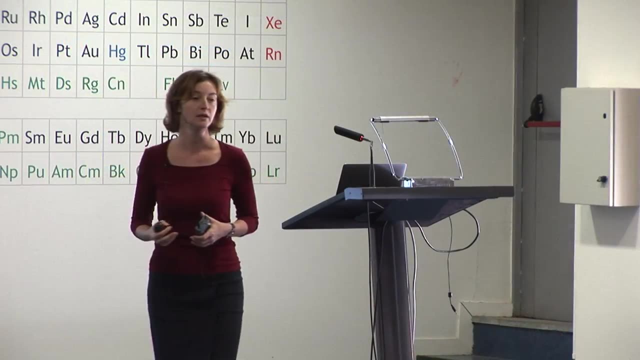 the mass of the WIMP and its cross-section. And it will be. you know, you will have quite some uncertainties. This is a study. there are many studies, but this is the uncertainties here. they actually come from the uncertainties on the astrophysical parameters, on the density, here on the velocity. 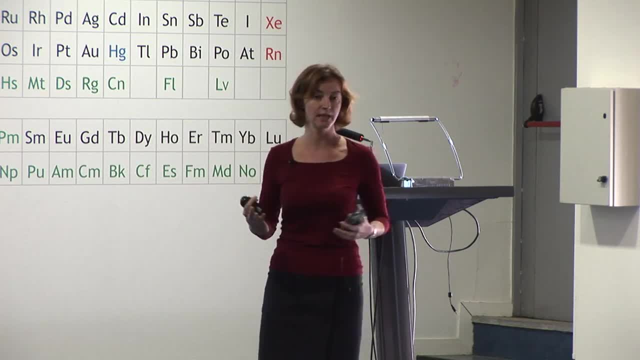 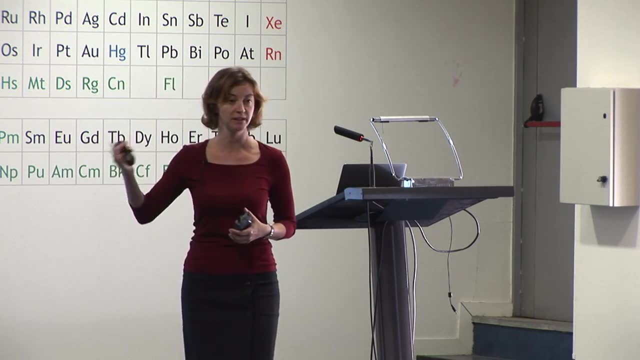 and also on the escape velocity. However, with such a large-leaked xenon detector that has an incredibly low background, you can also look at other physics channels like PP neutrinos double beta decay in 136 xenon and so on. 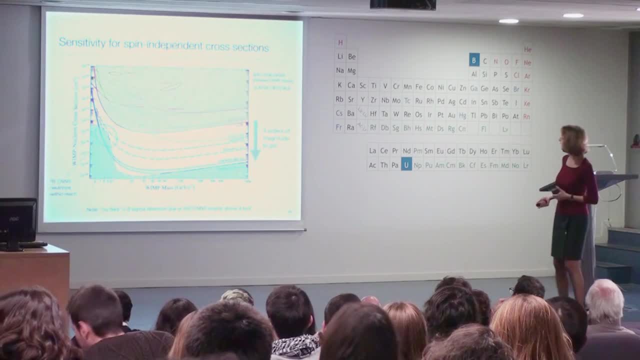 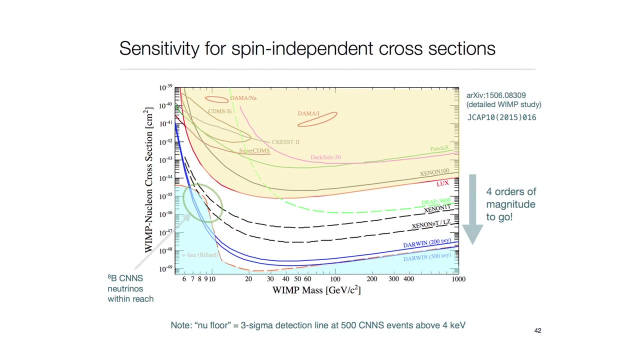 So where do we want to go in this, in this parameter space? So again, we are here now with LUX. This is the prediction for DEEP 3600 that I just mentioned, The prediction for xenon 1-ton, and then N-ton and LZ. 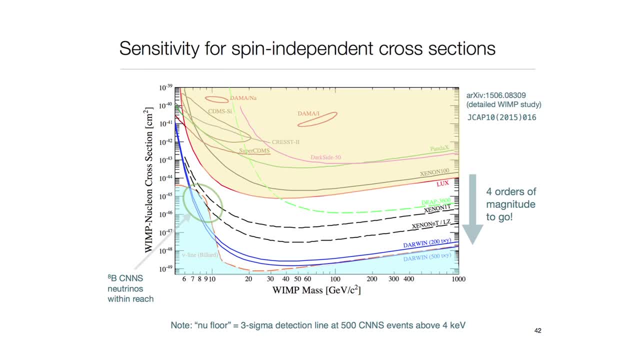 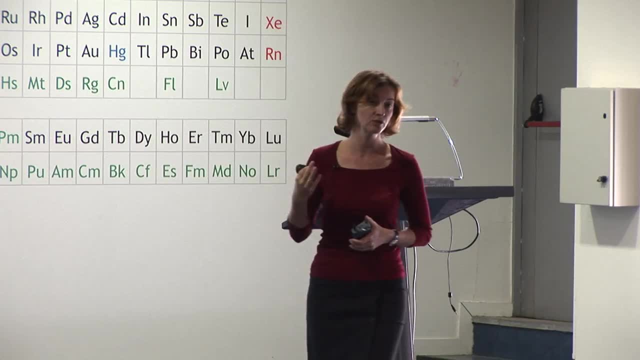 And then finally, this would be for Darwin. We have done quite some detailed study here. for an exposure of 200-ton years. I should say that this region here, where neutrinos are Okay When neutrinos start to dominate, is actually quite you know, the assumptions are that. 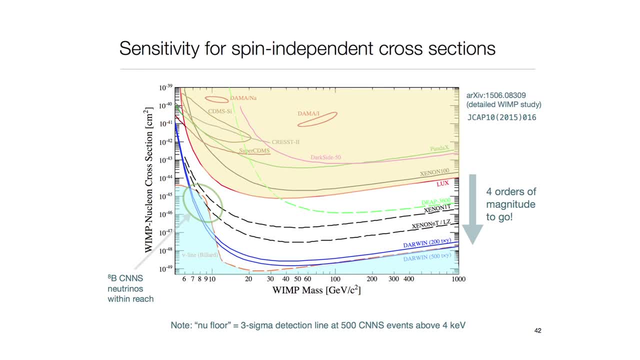 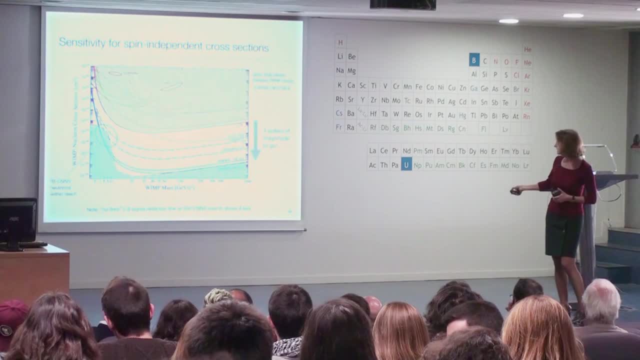 you have a 3-sigma detection line here at 500 events above 4kV. okay, So these are it's a very, very high exposure to reach this. So you can see, even with 200-ton years, we barely get here okay. 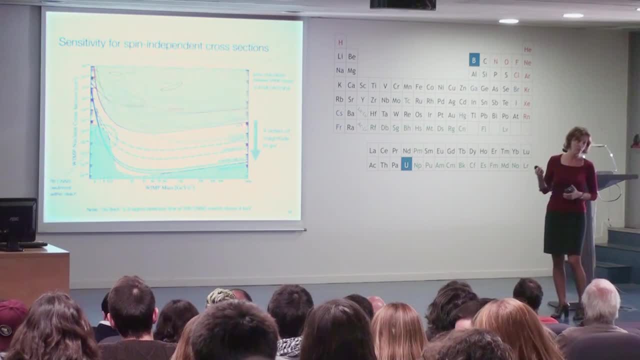 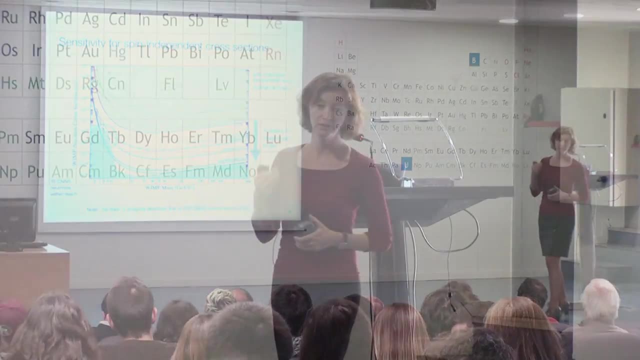 So this is when I said we have here four orders of magnitude to go to actually reach that region on the one hand. On the other hand, here for the Bohr 8, coefficient With Bohr 8, coherent scattering, we will already start to see some events in a xenon. 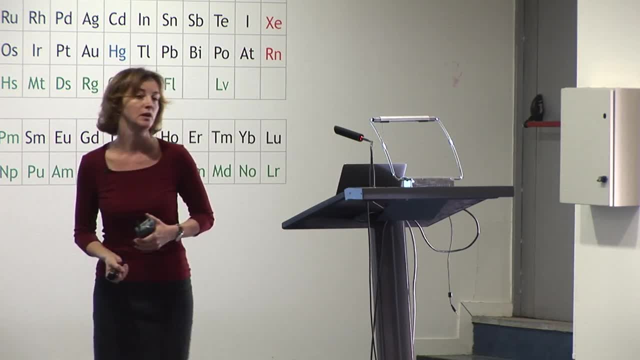 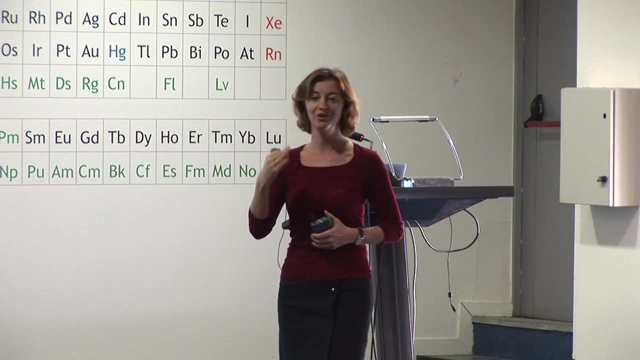 1-ton upgrade. okay, so with xenon N-ton- And we are looking, of course, at the detailed predictions there- It depends a lot on your low energy threshold, on the light and charge yield, that is, low energies, and so on. 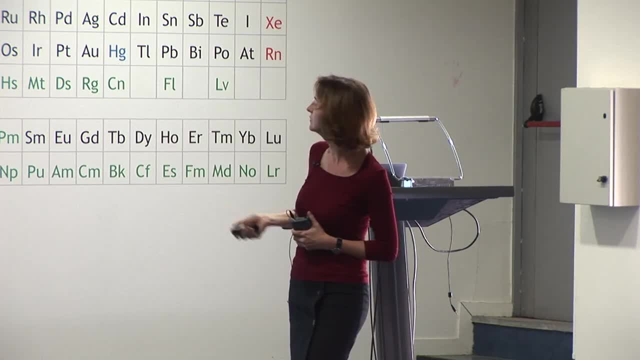 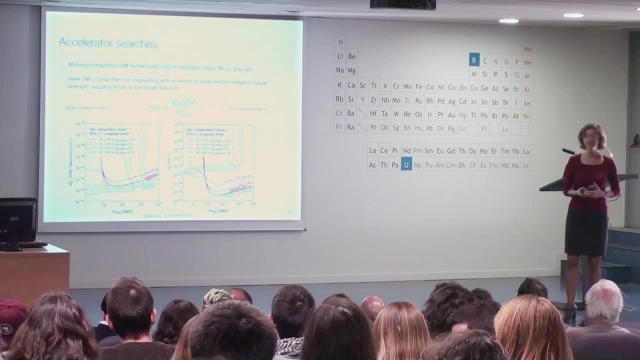 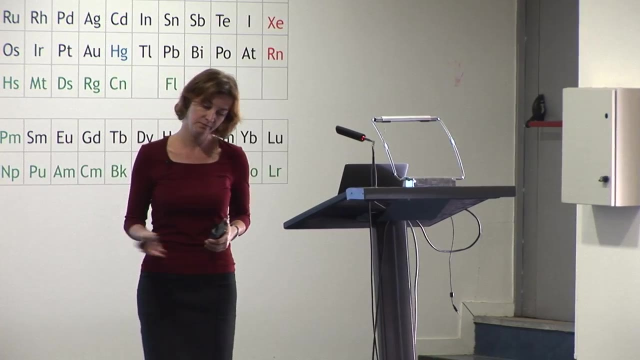 So there's quite some uncertainties there, but it will start to cut into this region. Maybe just one comparison, Okay, because you might ask: you know, how do we compare with accelerator searches? Again, there's a lot of literature here and you know some people go to these so-called 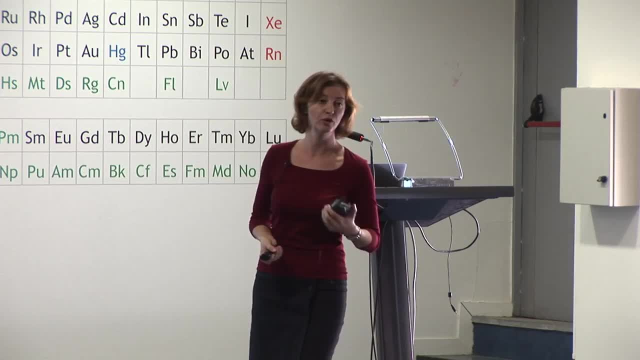 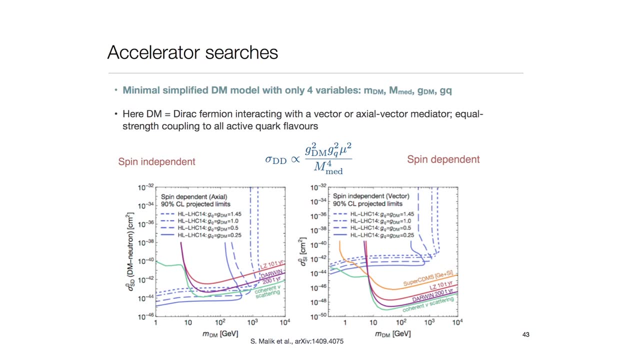 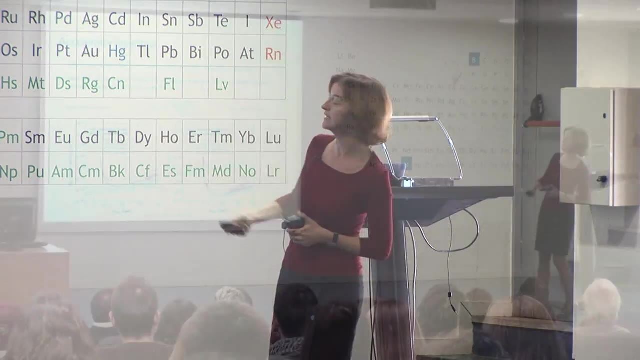 minimal, simplified dark matter models where you only have four variables, basically the mass of the WIMP, the mass of the mediator and then these couplings, and that the cross-section dimension will scale. like this: here, For instance, you could have a Dirac fermion that interacts with vector or via axial vector. 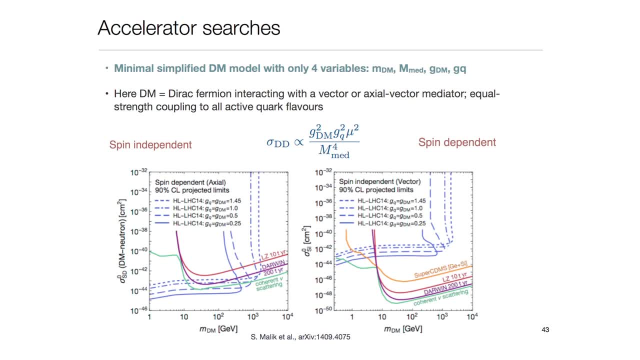 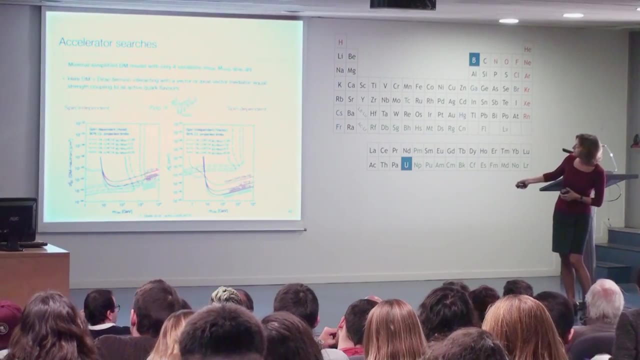 mediator, And this is a study done in this paper. so basically this is LHC14 predictions here for the spin-independent channel for various couplings, because these couplings are of course not known okay, as a function of the mass, and this is then compared here with LZ and Darwin. 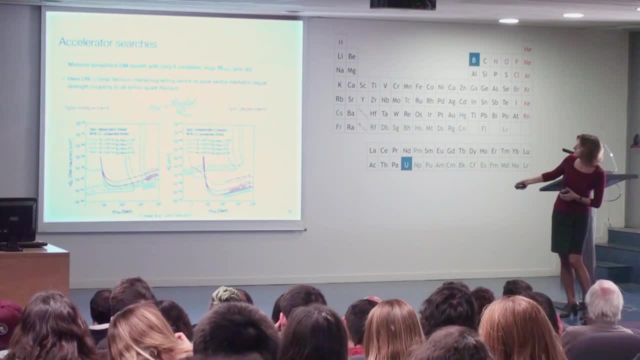 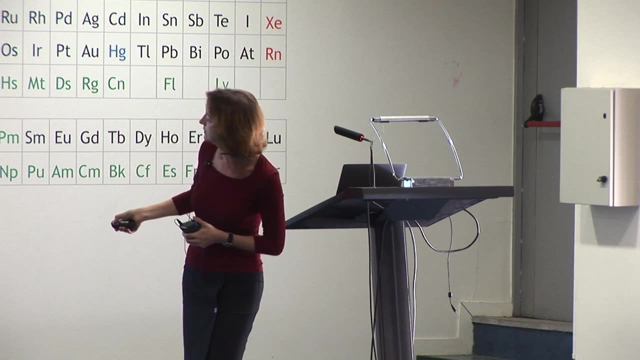 So obviously LHC has here much better sensitivity at low WIMP masses because they are not limited in energy to create this For the spin-dependent channel. Okay, So the channel here? sorry, this should be the other way around. yeah, So this is the spin-dependent, but actually they're quite competitive, but here spin-independent. 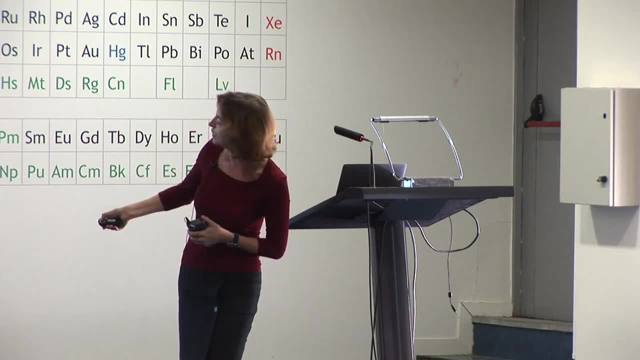 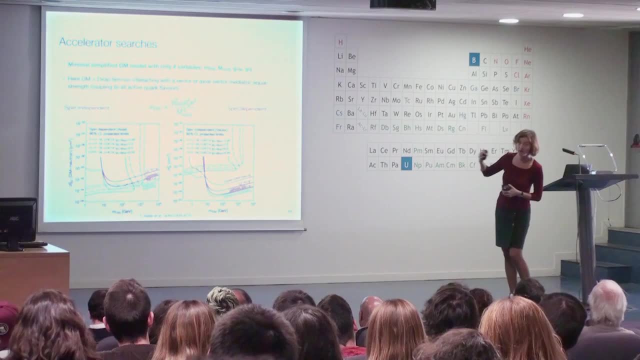 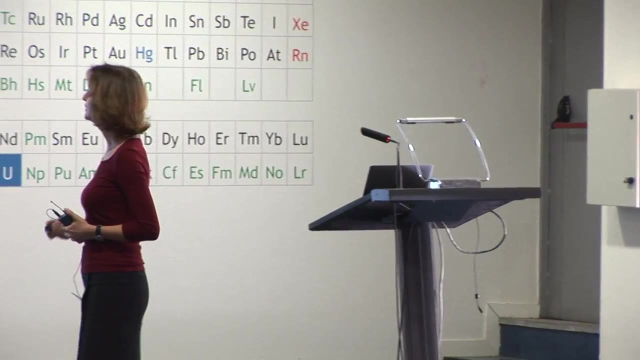 we can see that. you know, LHC is here not really competitive, but still they can probe here this low mass region that is very hard to this, is very hard to measure with direct detection experiments. So and so my last slide. this is just a historical plot. I mentioned that I started to work on 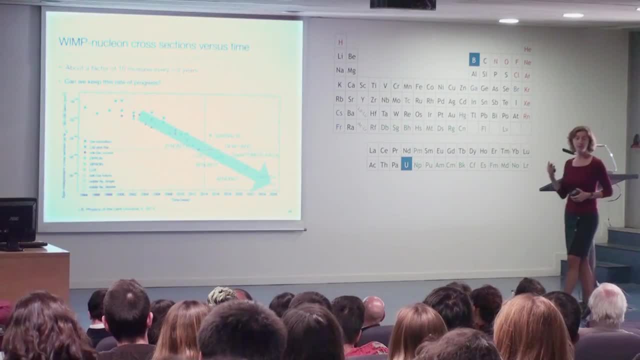 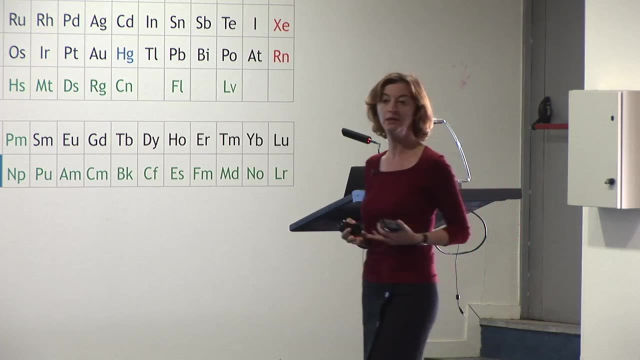 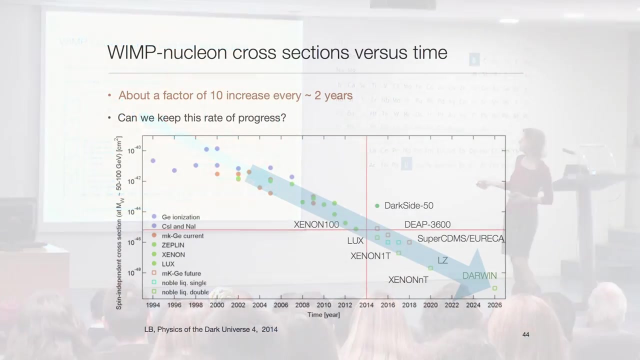 this field very long time ago. so back then we actually were working on double beta decay with germanium ionization detectors, and because the requirements are very similar, namely extremely low background from radioactivity, cosmic rays and so on, we also started to look at dark matter interactions and set here some first limits. but then really the field: 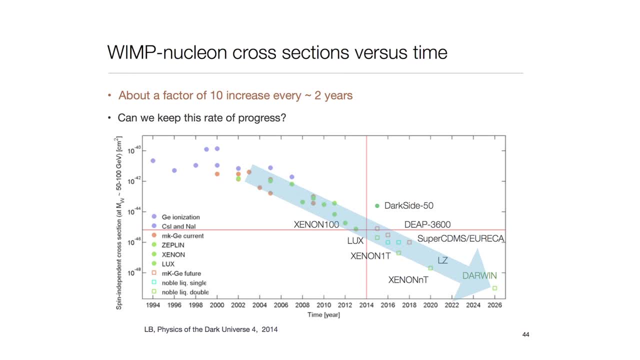 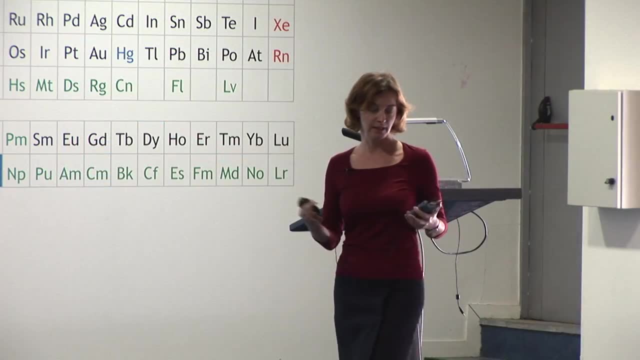 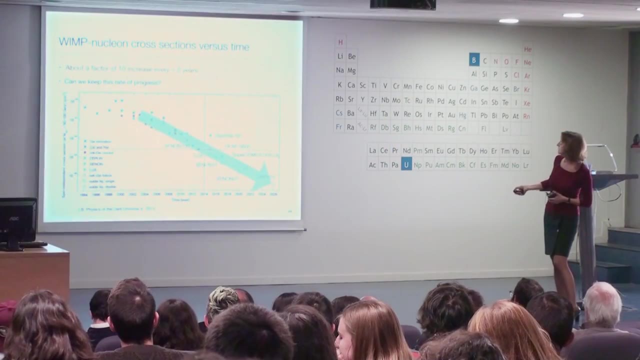 took off once these cryogenic experiments came on board: the millikelvin detectors, such as CDMS, And then later the And detectors that are based on noble liquids, most notably here liquid xenon detectors, you know, such as we were here with xenon 10, then 100, lux, and so on. 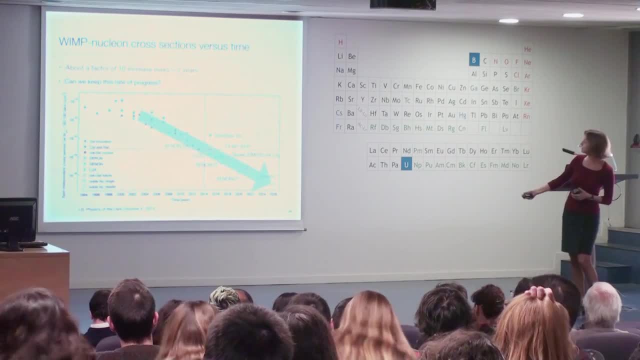 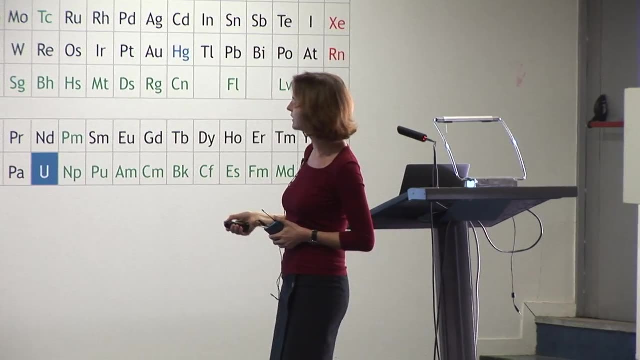 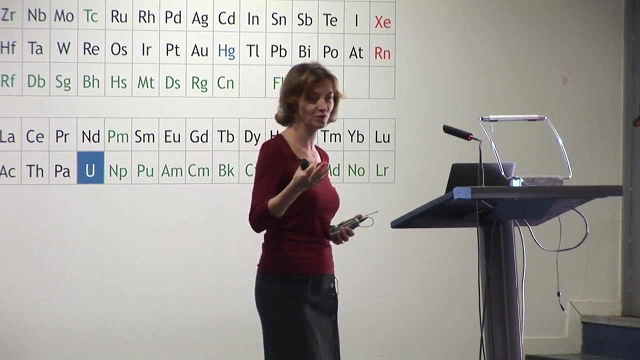 And these are just, of course, now predictions where we would like to go in terms of the cross-section as a function of the year here. So when I actually looked at this plot I couldn't believe it, but here there was about a factor of 10 increase in sensitivity every two years. that was quite amazing. so it beats. 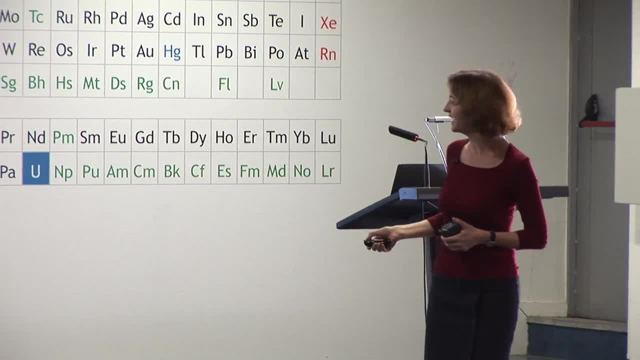 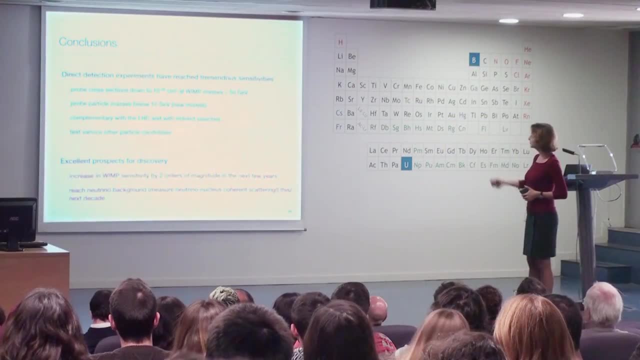 Moore's law. So, on the one hand, On the other hand is: you know, can we keep this rate that we have to demonstrate now? We don't know. Okay, So what I've shown you is, hopefully, that direct detection experiments have reached. 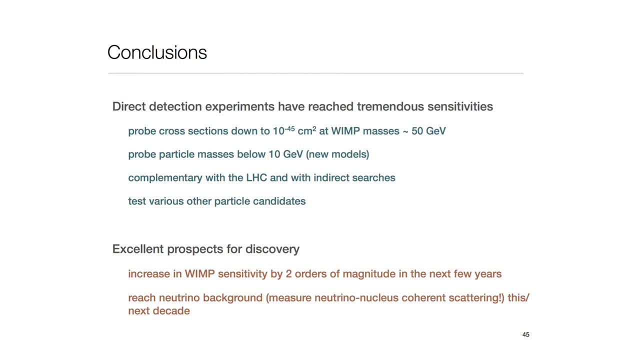 tremendous sensitivities. We can probe now pretty low cross-sections, down to 10, to the minus 45, or even lower now, for mean masses around 50 GeVs. We can also probe other particle, well, particle masses below 10 GeV and, in fact, new models. 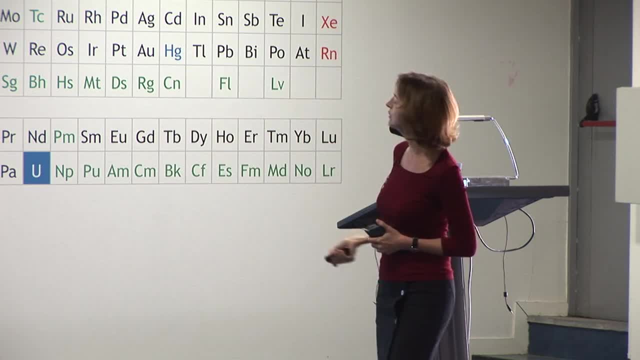 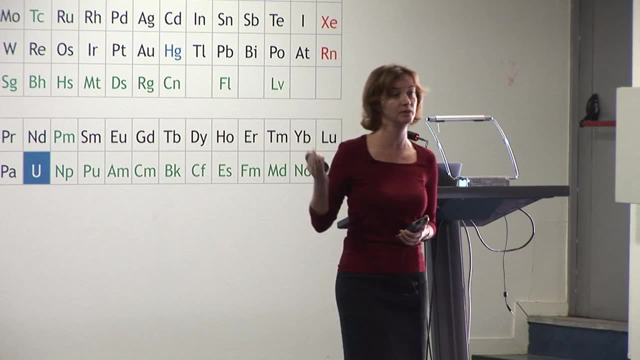 There are also. Okay, Thank you. There's also quite a lot of, There's a lot of literature on this. We are quite complementary with the LHC, but also with indirect searches that I haven't really shown here. With indirect searches it's easiest to compare with searches for a neutrino annihilation. 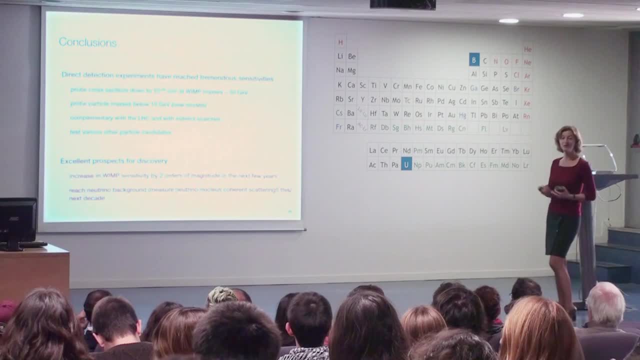 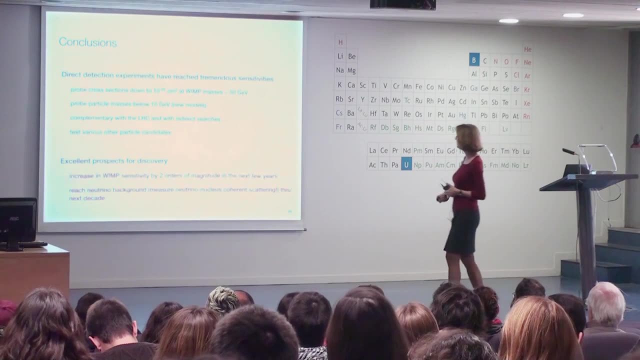 in the sun. Well, I could say that the prospects for discovery are quite good. We have increased this sensitivity in WIMPs by about two orders of magnitudes and we have to increase it in the next few years And hopefully we can reach really this. 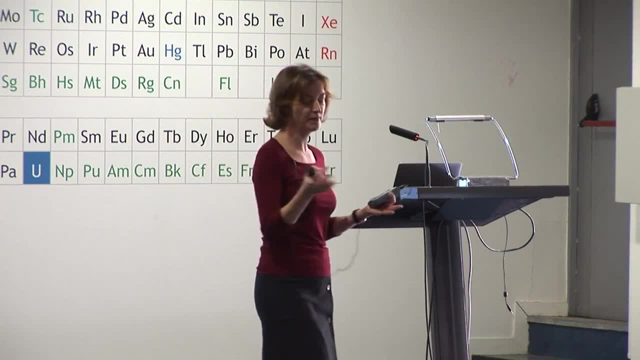 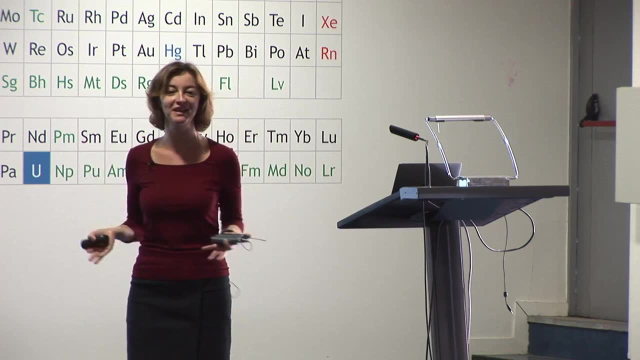 Okay, So, Yeah, So we've got. at least We've got to make saver. Yeah, But we want to. We have to make saver, Yes, Yeah, Okay. So now I will end. So I think that's. 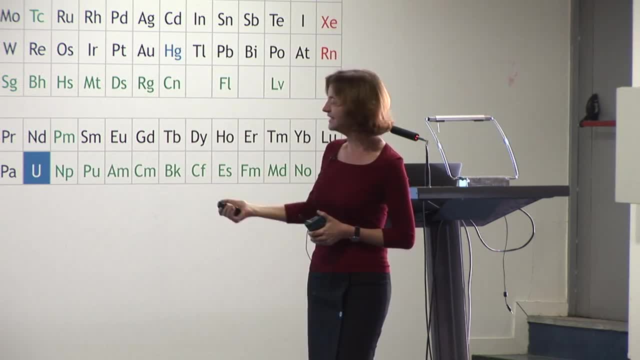 And then Thank you very much. Thank you, That was a pretty good discussion. Thank you for coming. Thank you, Thank you very much. Thank you And thanks to the participants, Thank you, thank you, Thank you very much. 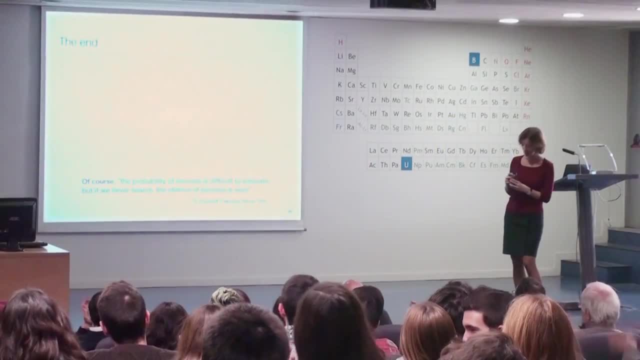 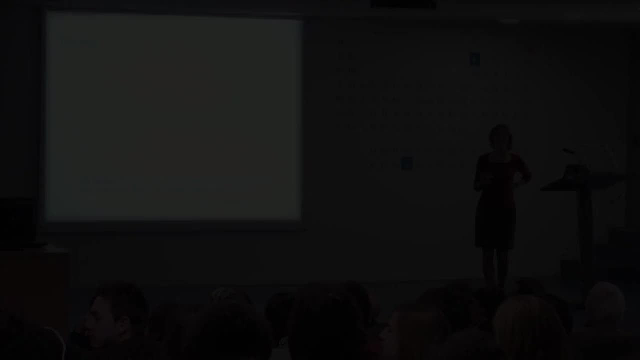 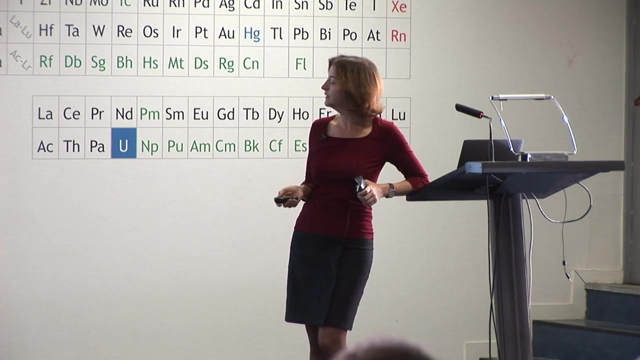 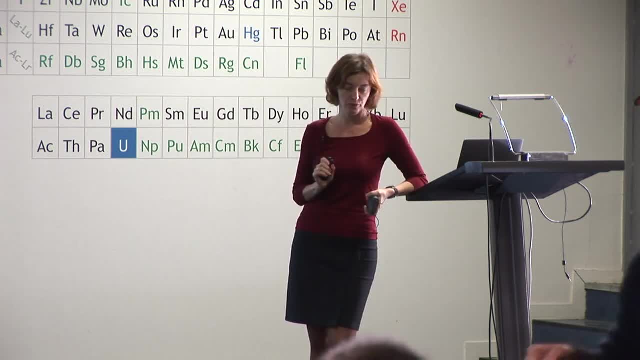 studied, namely directional information that you could use because you know, at least for the solar neutrinos, you know the direction right, That's what you're saying, And you can improve, you can go below it. So this is a study that was shown that assumes gas that is used. 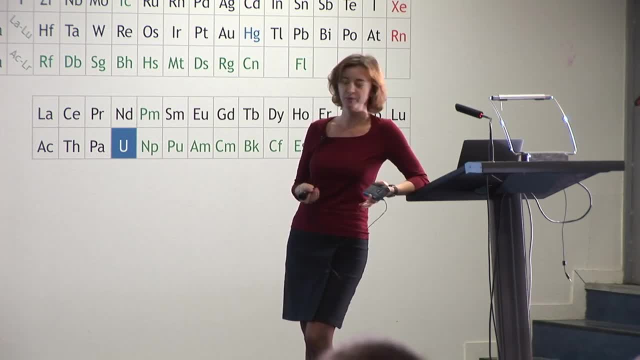 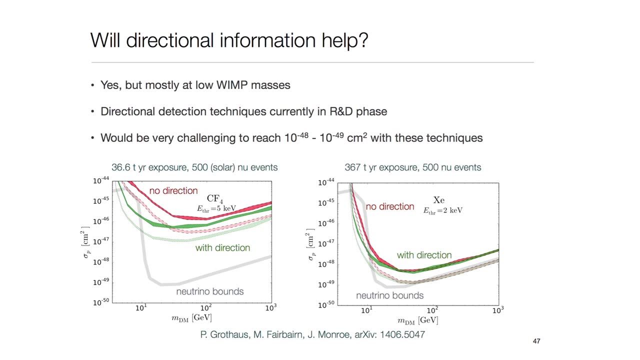 in directional detectors, as I mentioned, they have to be low pressure gas And this assumes xenon, even though in xenon we have no direction. But if you would have the direction that in xenon, you see you can improve here. 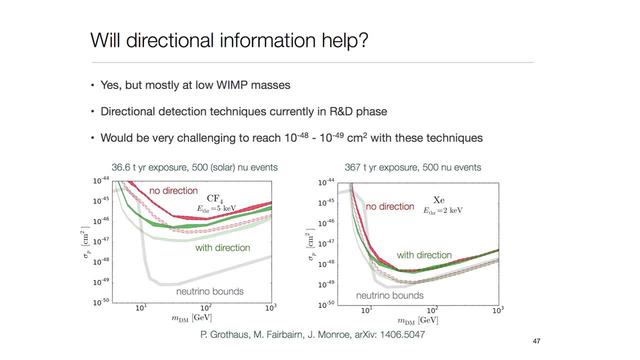 obviously these low mass WIMPs because you have the eight borne neutrino background. But at higher masses there's not much that you can do Because the atmospheric neutrinos they just come from everywhere, right, And similarly, actually here you can get some improvement. 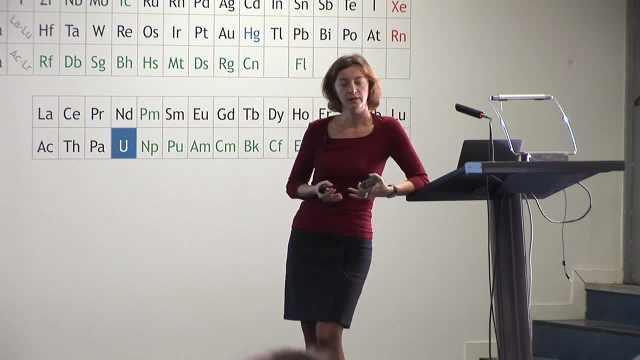 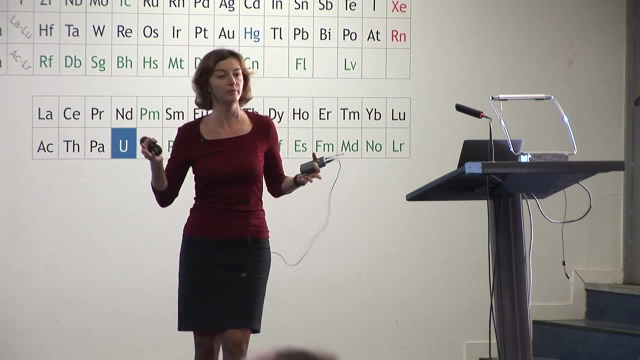 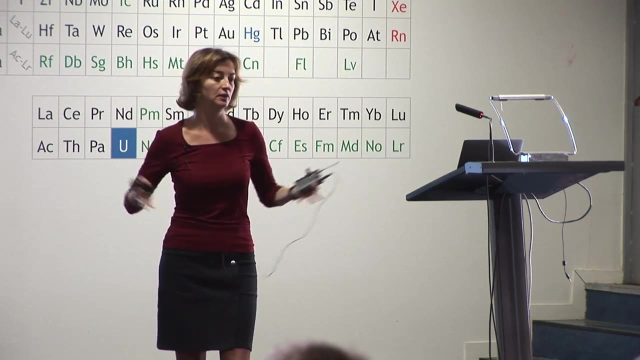 indeed, when you measure the direction. But it will be again depending what the cross-section is, because the current cross-section limits. if you want to build a directional detector, it has to be the size of minos. Maybe some of you are familiar with the large neutrino detector. 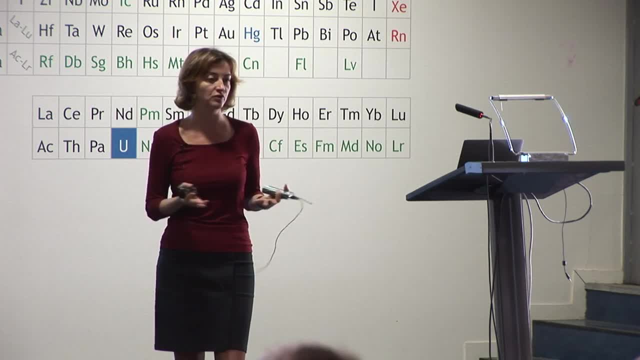 It has to be quite large, But we don't know if the cross-section is 10 to the minus 45, it's probably not right. So if you go to 10 to the minus 49,, well then, building a detector that has. 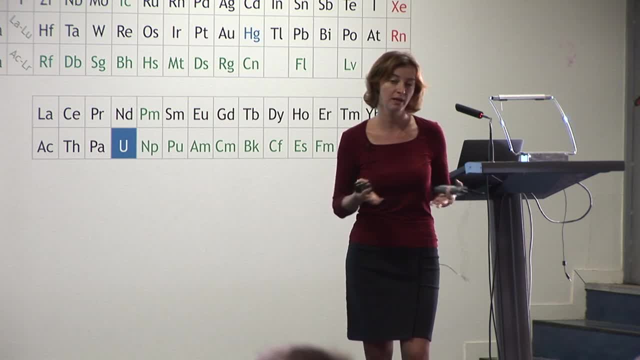 directional sensitivity. it will be gigantic. You may want to do it, but I think you will only do it actually in case you have a discovery. Because if you have a discovery with any of these detectors, then you say, OK, I know. 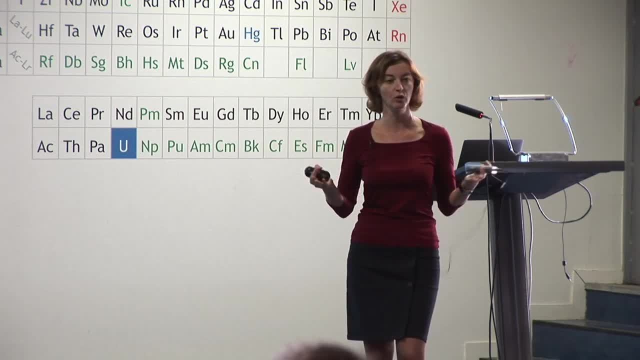 more or less what the mass is, what is the cross-section? I know what type of directional detectors I want to build to confirm that, But if you have nothing, then going and building I don't think you will get the money for that. 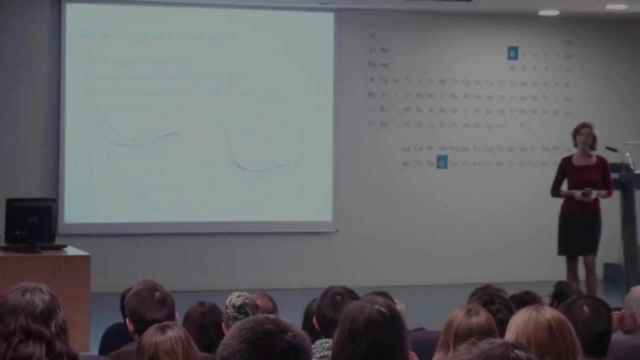 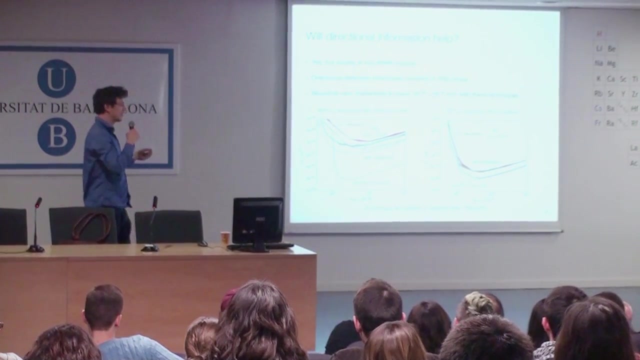 or that anybody will probably do it. A quick, slightly naive question: Is it possible to use this space? Is the spin dependence that we, if we do see a spin dependence, does that tell us something about the spin of the particle, or is that something separate? Well, that's also a good question. It will be so. to look for spin dependency, you have to have, of course, a nucleus that has non-zero spin right, total angular momentum, Like in xenon. it's 129, 171.. 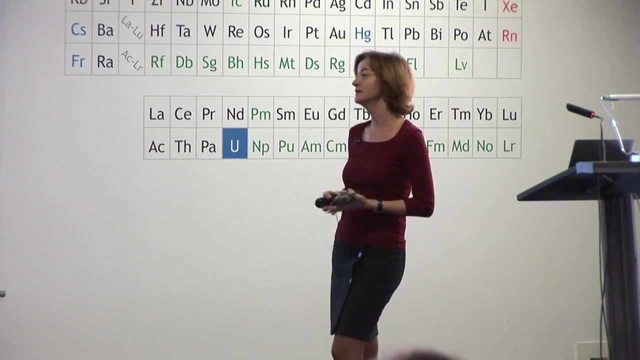 But also your dark matter particle has to have a spin, yeah, But then from a direct detection experiment. Yeah, But to actually determine the spin of that particle, that will be very difficult, Actually even determining that what you see is due to spin interaction, spin-spin it. 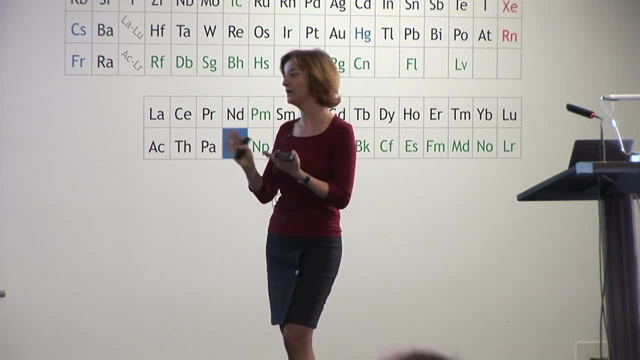 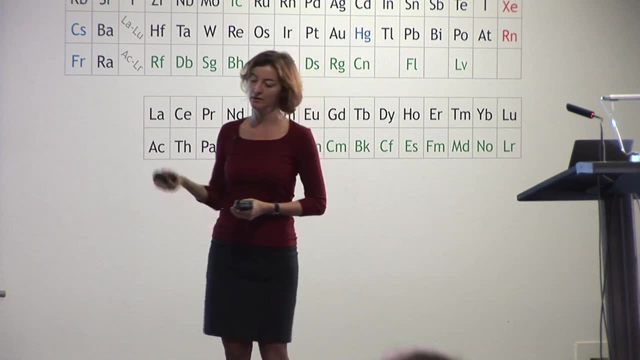 will be very hard. You know there are ways to do it: by comparing different materials, by looking for spin-dependent, inelastic scattering and so on. because inelastic scattering, the cross-section for spin-independent is much, much lower. so it's totally suppressed. 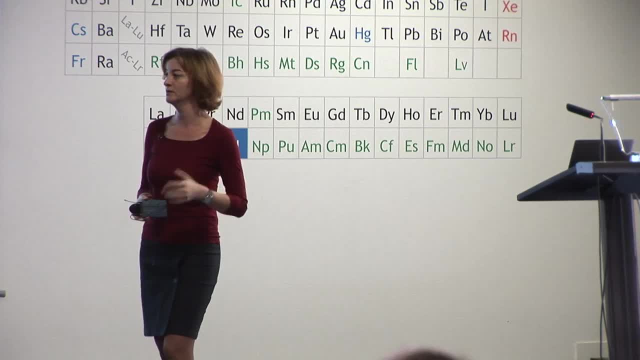 But I think there you really need a collider experiment to determine the spin. yeah, All right. Thank our speaker again.